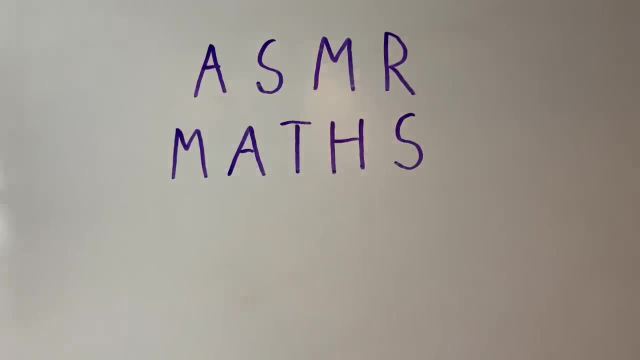 on the channel before. We have done quite a few before, and in tonight's video we're going to be solving a multitude of variety of difficult, easy, average maths problems, And I'm going to be doing it all on this whiteboard, so we're going to have some nice colourful 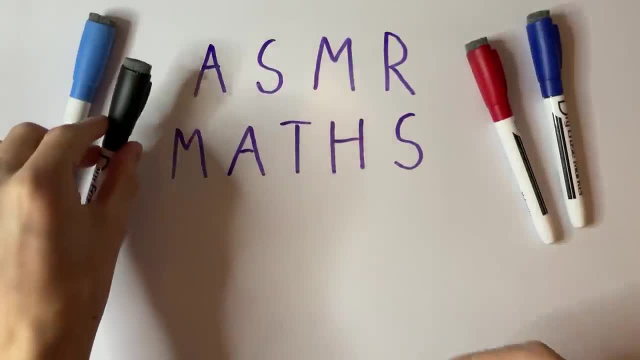 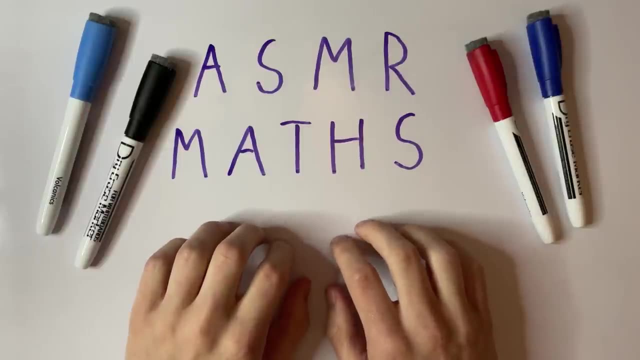 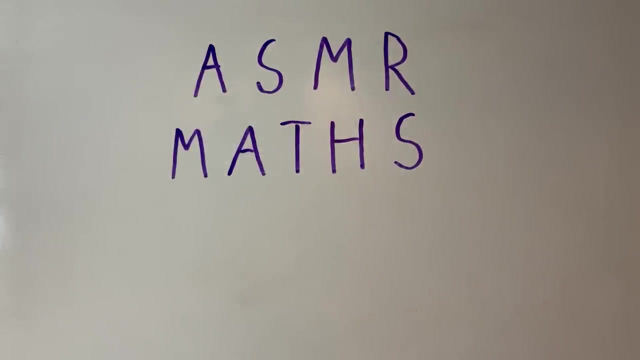 pens to do the questions on this board and it'll just be a nice little layout for you guys to watch. And, as I mentioned, this is not the first time. we've done a maths video before. I've done several maths-related videos before and I always get people asking me to up the 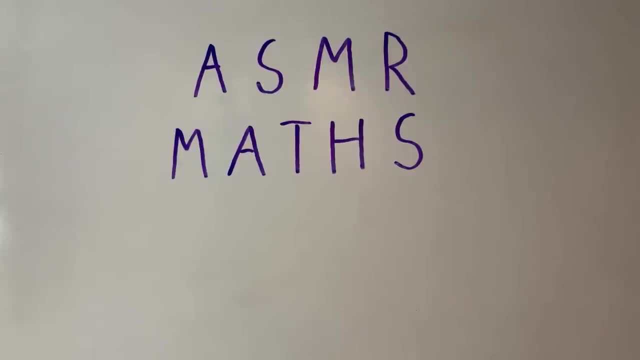 difficulty of the questions I do or do a few more complex mathematical concepts, And so that's why in tonight's video, with the timestamps below you can see, we're going to be doing a whole bunch of different questions, ranging from calculus questions with 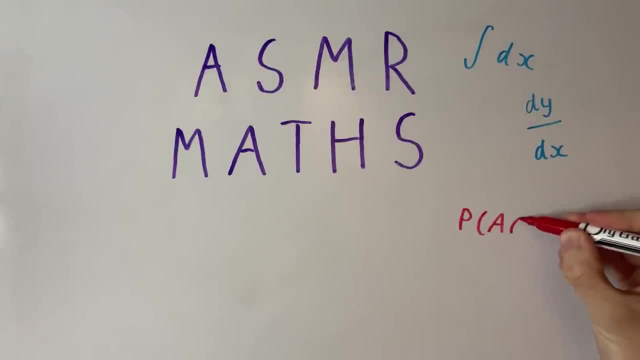 integration, differentiation, statistical problems, including probability, and lots of other data analysis questions. There'll be questions about geometry, questions about limits, questions about diagrams and curves and all that kind of stuff. lots of different questions that you can see with the timestamps below. 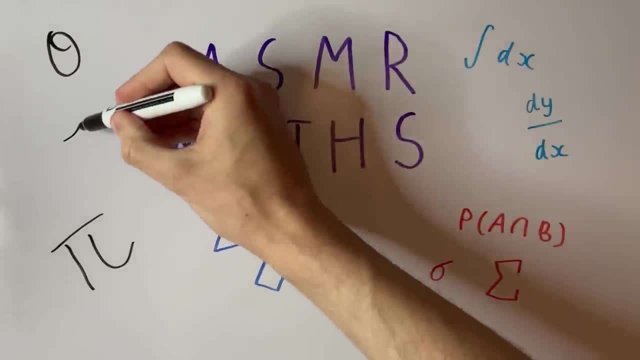 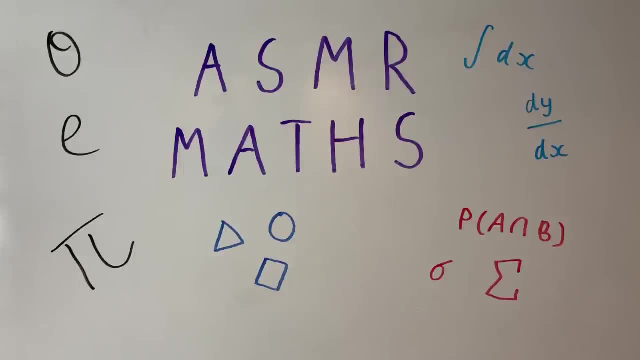 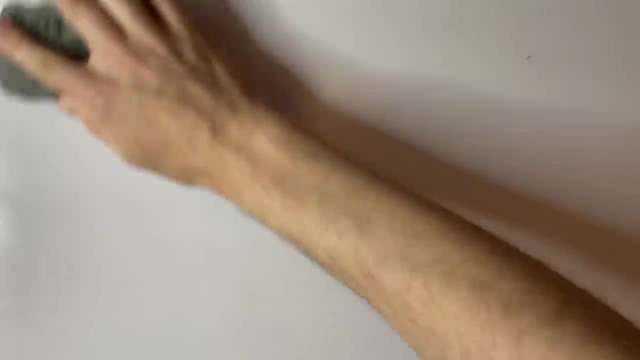 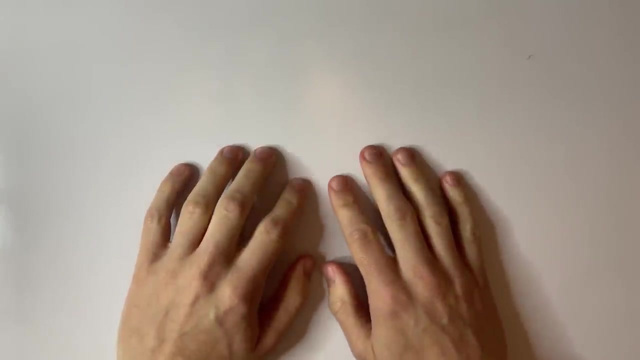 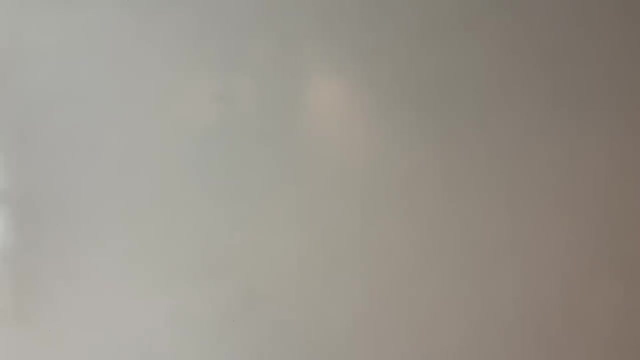 speaking of which a lot of you guys might not know, i actually study, study, study, study mathematics at university in scotland, and it is a dream of mine to one day go on to teach high school mathematics and so to help me improve my teaching ability and to help others learn mathematics. 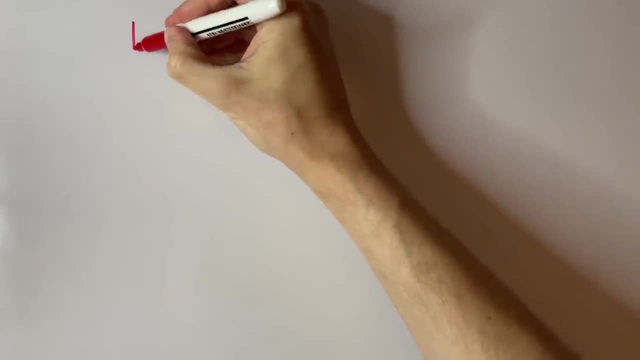 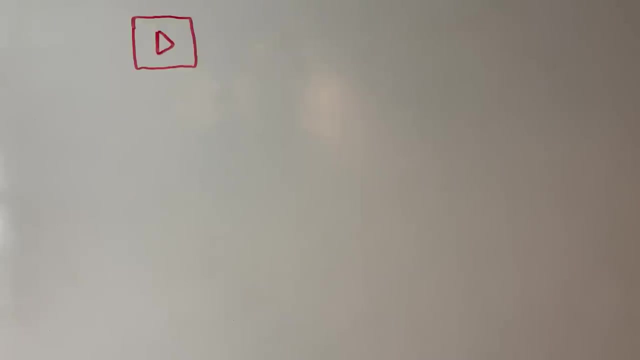 especially at times like these when it's difficult to get out the house and not everyone's able to attend school. i have actually created my very own youtube channel where i will be teaching scottish qualifications mathematics levels, and this channel is called sqa maths, which i will link in the description down below. if you guys would like to go and check it out, drop me. 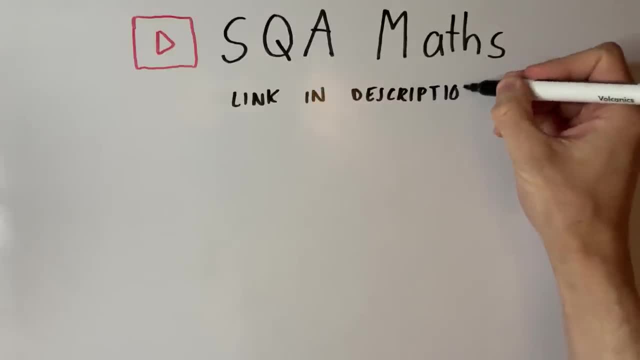 a like and subscribe, if you haven't already, and i will see you guys in the next video. so thank you so much for watching and i hope you enjoyed this video and i will see you in the next video. bye, bye, um, but if not, it might still also make sense to you guys as well. so please, if you get the chance, 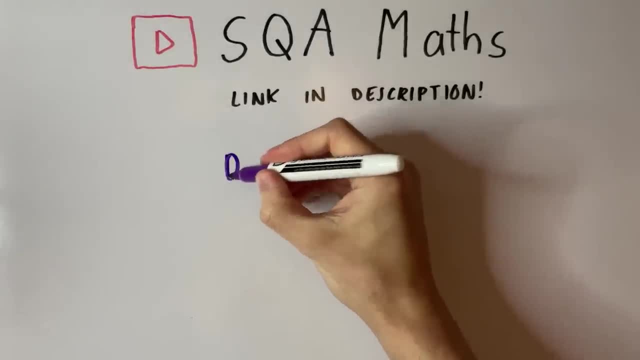 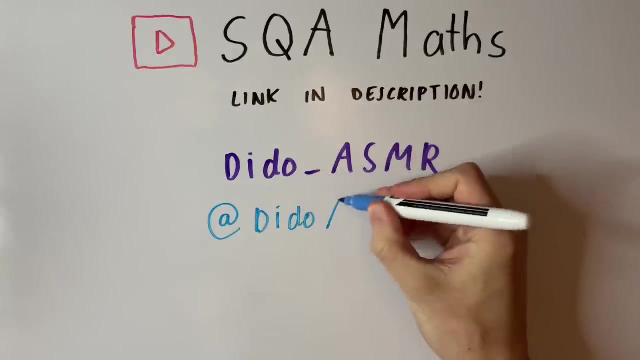 do go and check it out, give me some support, give me some feedback. it's all welcome trying to improve and become a good teacher. and also, before we get into tonight's video, i do want to quickly say: if you guys have any problems math related or just want to have a chat about maths, do not hesitate to. 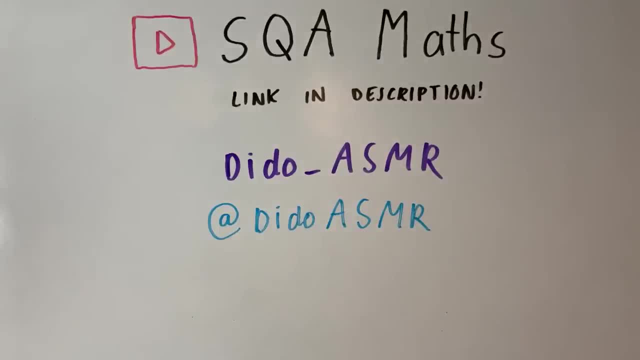 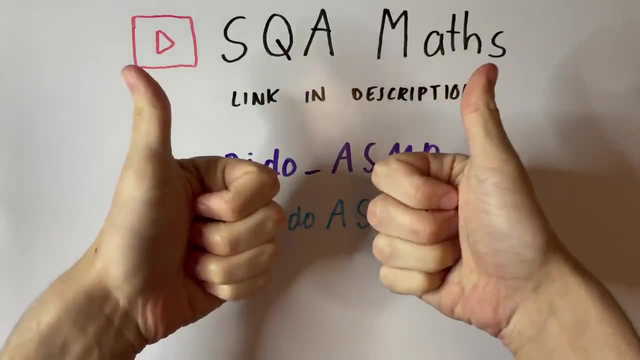 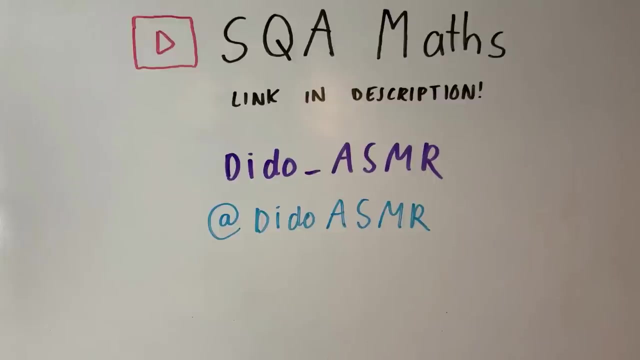 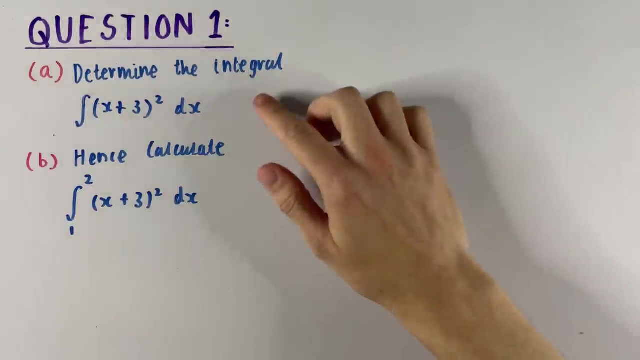 send me a message on instagram or on twitter, as you can see on the screen now: instagram on top, twitter at the bottom. if you have any problems, feel free to send them my way. anyways, i'ma stop rambling. let's get on to tonight's relaxing maths. okay, so for question number one, it looks like we 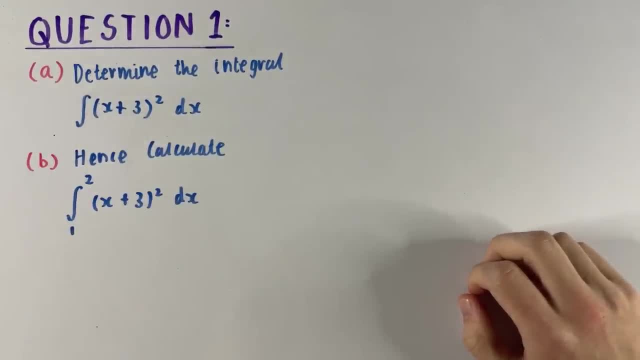 are going to be starting with a bit of a simple integration, as we have two parts to this integration question. part one: we are asked to determine the integral of x plus three, all squared dx, and then part b says, hence calculate the definite integral from one to two. 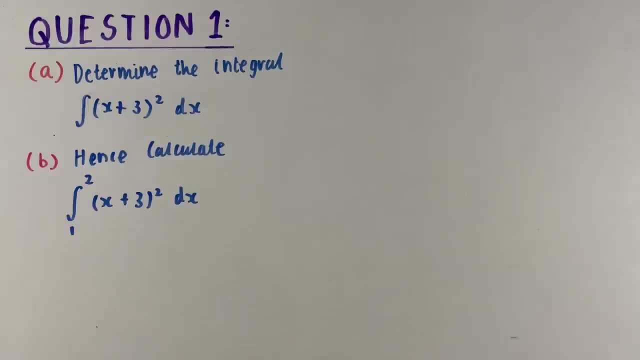 of x plus 3 squared dx. So very nice integration question to begin the video. So let's jump into how we're going to go about solving part A, because it looks like we need to do that before we do the definite integral in part B. Okay, so let's begin by determining the 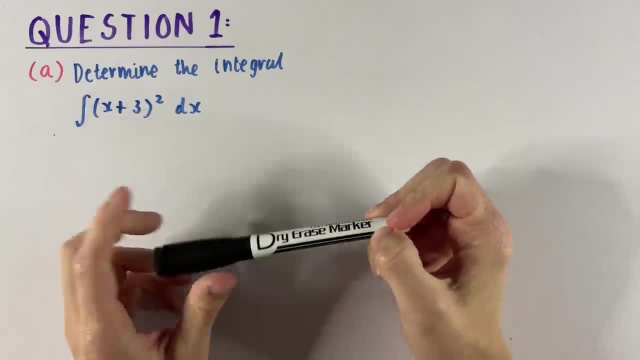 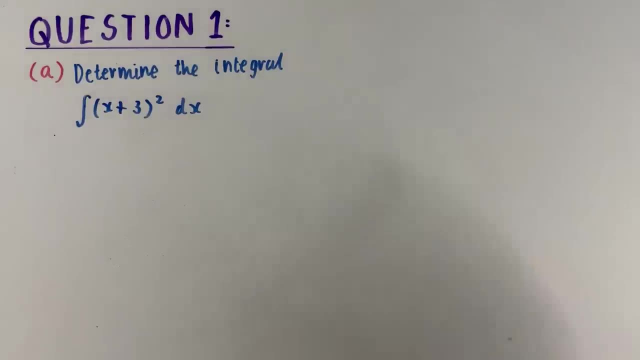 integral of x plus 3 squared dx. Alright, so, as you know, we've got this function in terms of x. Now I think the best place to start with this question is maybe simplifying the integral for us a wee bit. So let's say that we are essentially evaluating the 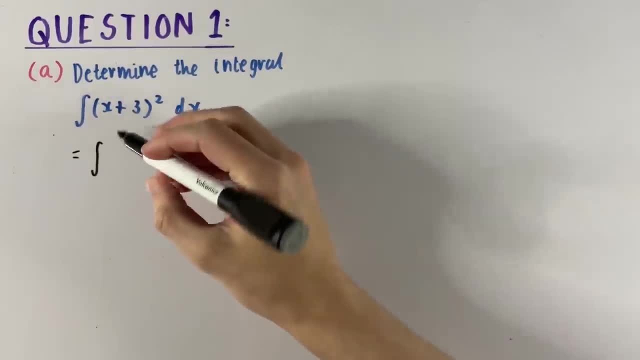 integral of x plus 3 squared dx. So let's say that we are essentially evaluating the integral of this bit expanded. So let's expand the brackets first. So we're going to get x squared, We're going to have plus 3x, plus another 3x, So it's going to be plus. 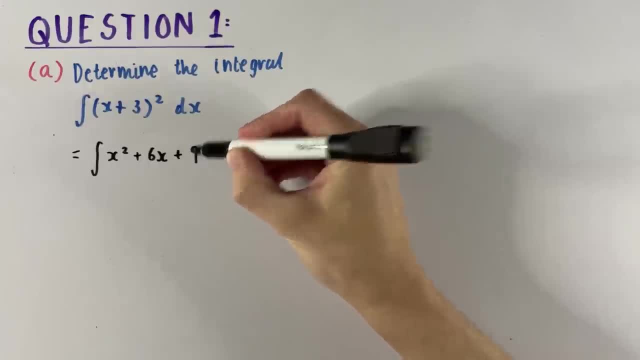 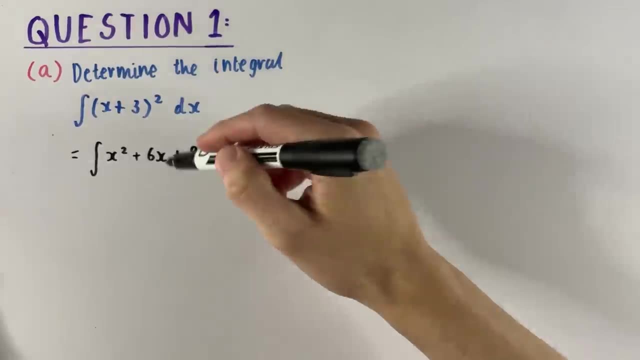 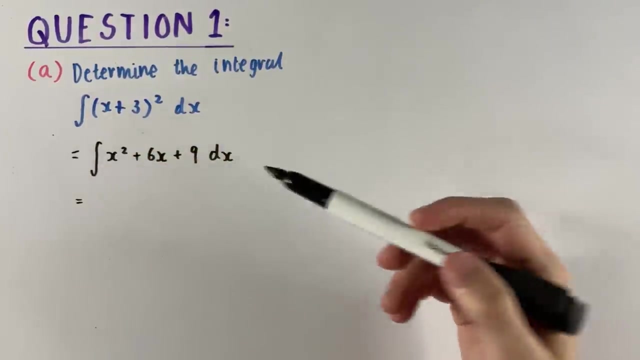 6x plus 9 dx, So this just makes it a little bit easier for us to start with, which is the same thing as this here. So let's evaluate this integral. This is going to be well. by our rule of integration, you increase the power by 1 and divide it by the new power. 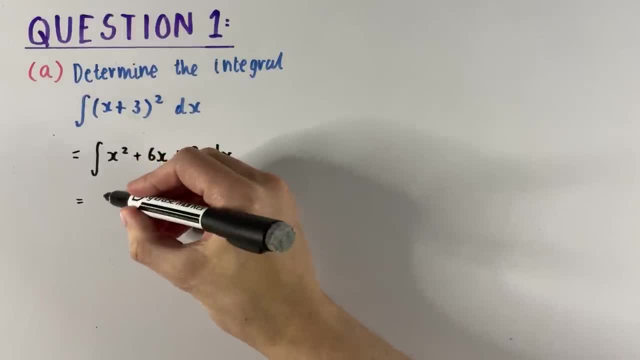 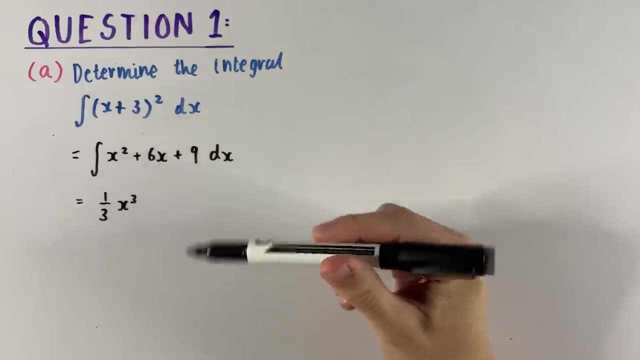 So it's going to be x cubed divided by 3.. I'm just going to write 1 third x cubed. essentially the same thing. Now, here we're going to have 6x squared divided by 2.. Now 6 divided by. 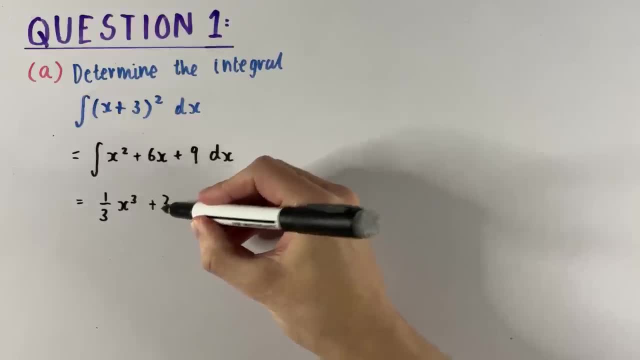 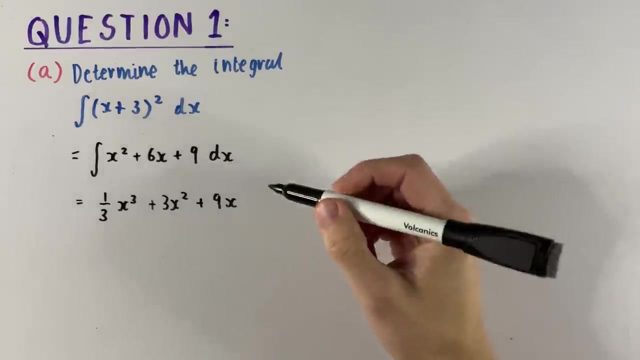 2 is just 3.. So this is going to be plus 3x Squared, And then we're just going to put plus 9x, because this is technically x to the power of 0. So it just goes to x. Then we divide by 1. Just gives 9.. And don't forget: 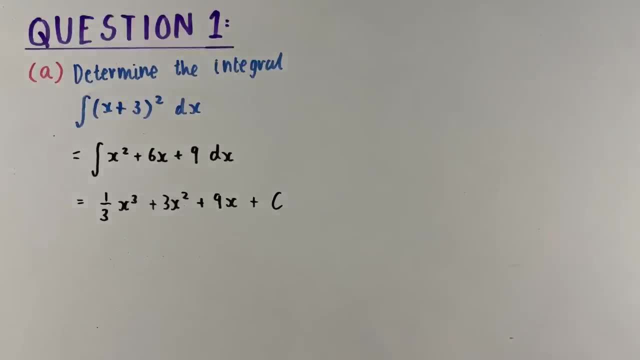 we have the constant of integration, So plus c, And that seems to be it for this part. We can't simplify this anymore, So everything looks good And I'll leave that as my final comment. So thank you so much for watching. I'll see you in the next video. Bye. 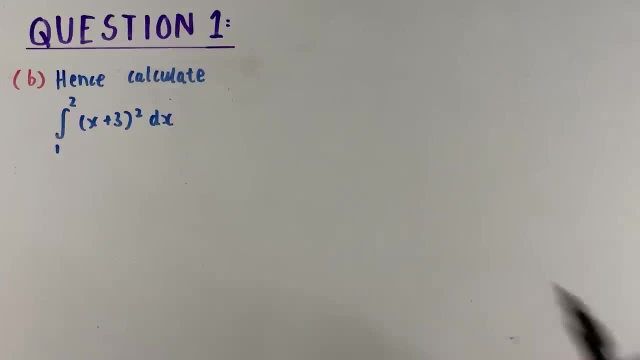 Final answer. So for part b, we recognize that we've still got the same integral from part a. However, this time the integral has limits Or it's a definite integral. we could say So. from the first part we said that the integral is equal to 1 third x cubed. 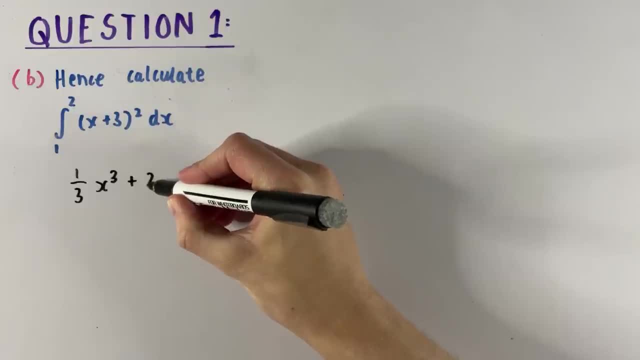 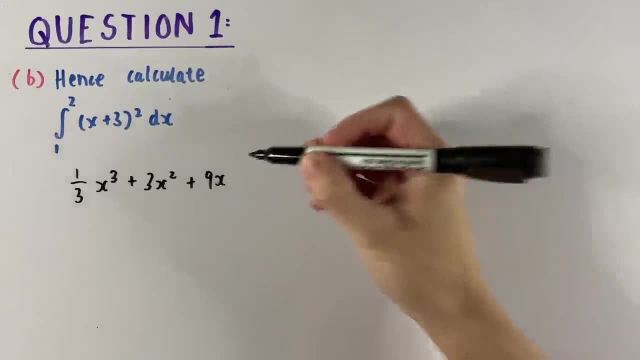 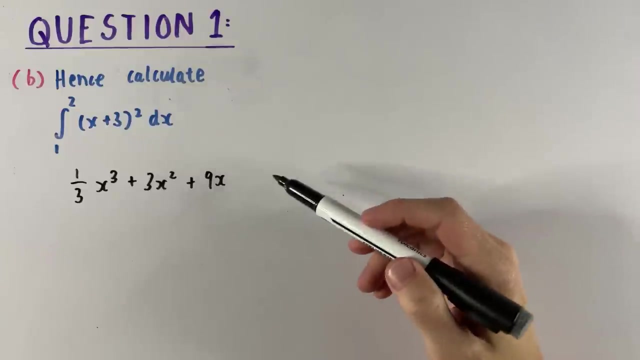 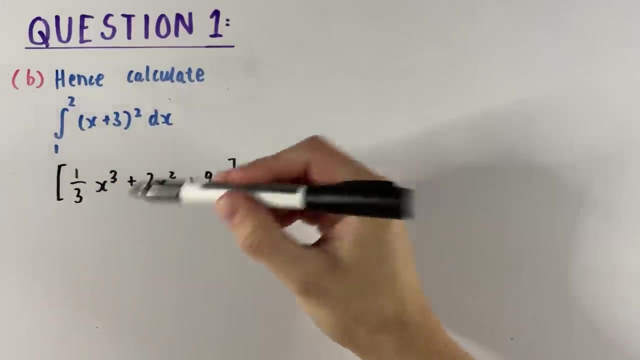 plus 3x squared- I was just trying to remember it- Plus 9x Now, because this is a definite integral question, we do not need the constant of integration. We simply want to evaluate this integral from the limits 1 to 2.. So when we do this, we're going to have a constant. 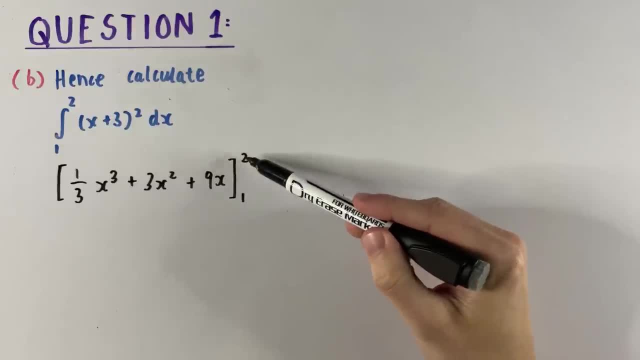 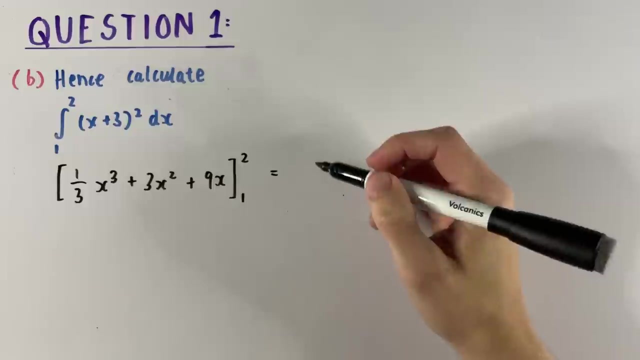 of integration. So when we do this, we begin by subbing in the top integral, definite integral. We want to sub in the 2 to this first And then we want to subtract when we sub 1 into this as x. So let's sub in 2 first We're going to have, let's just sub it in like this: 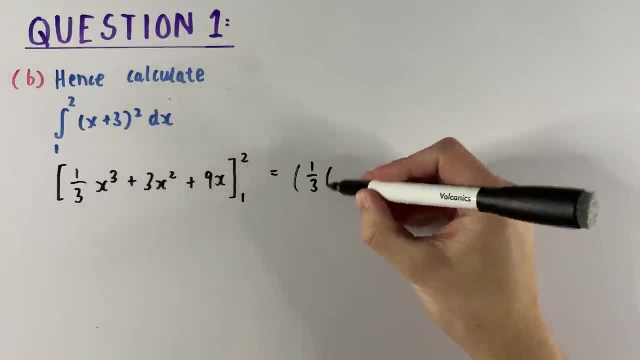 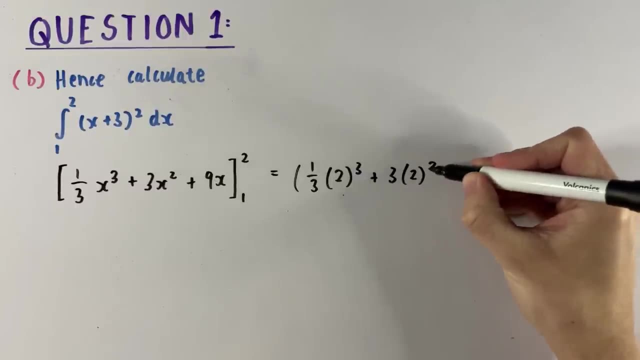 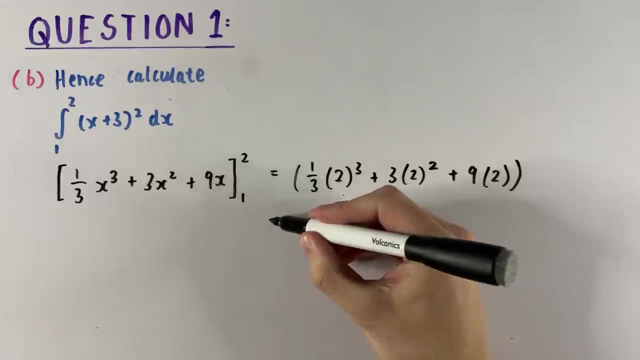 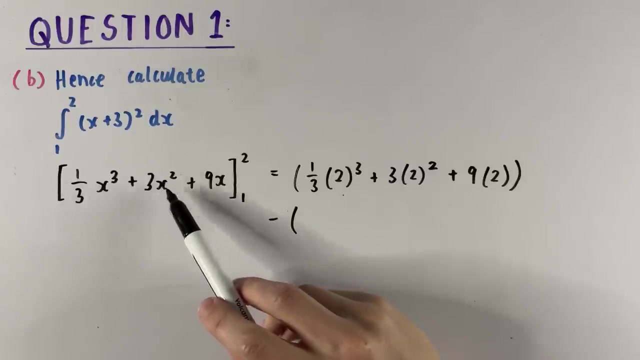 Let's do 1 third times 2 cubed, Plus 3 times 2 squared, Plus 9 times 2.. Like this, And then we are going to subtract, subbing in 1.. Now 1 cubed is just 1.. 1 squared is just 1. And 1 is just 1, obviously. So I'm. 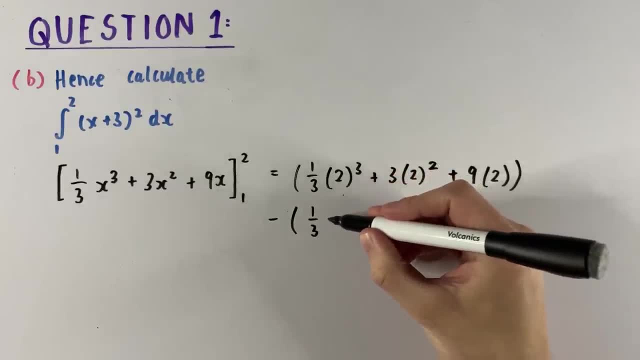 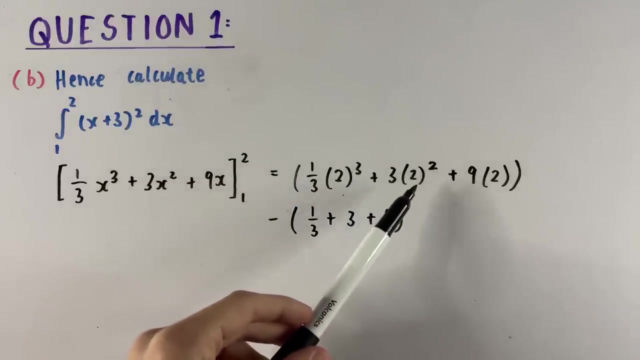 just going to write this as a third plus 3 plus 9.. Now for this particular question. you could multiply this through, So you'd get 8 over 3 times 12. That would be plus 18. And then minus this bit. But that's going to take a. 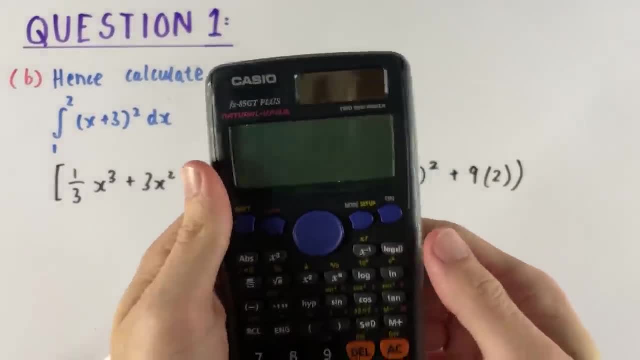 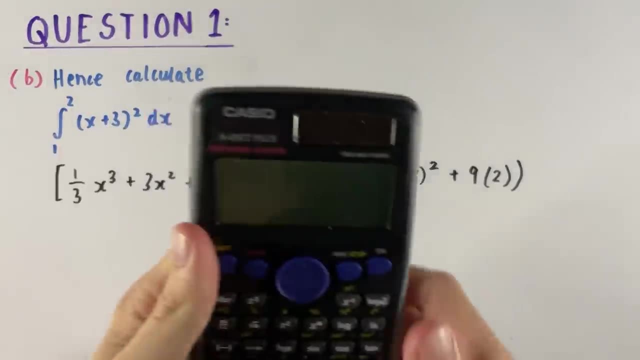 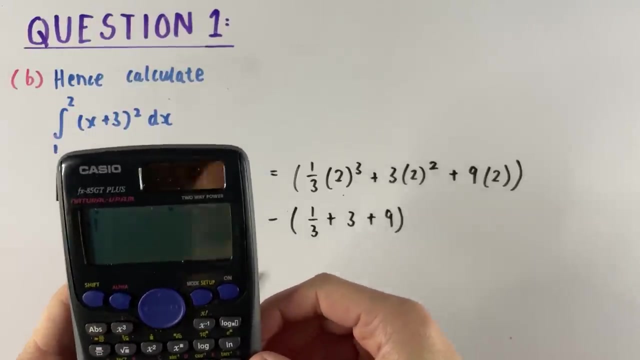 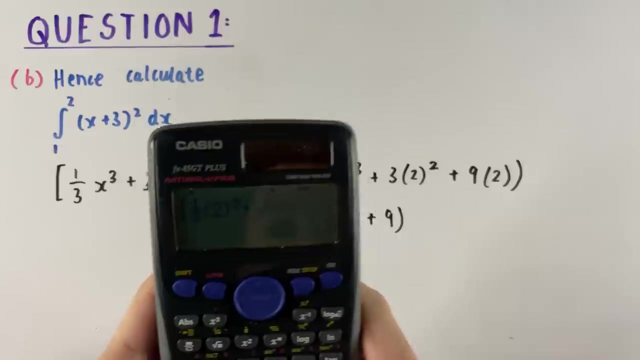 bit too long. So I have my calculator. Let's just plug this. Let's plug this equation into our calculator. So in the first bracket we have 1 third times 2 cubed plus. we said that was 12.. I'll just put it out for you, though, so you can. 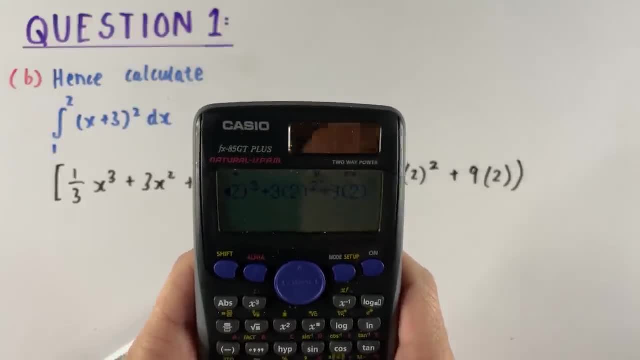 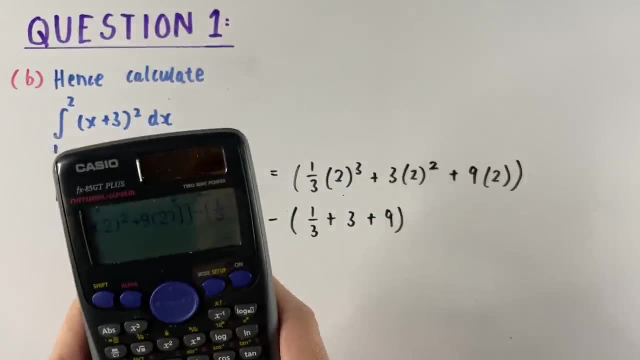 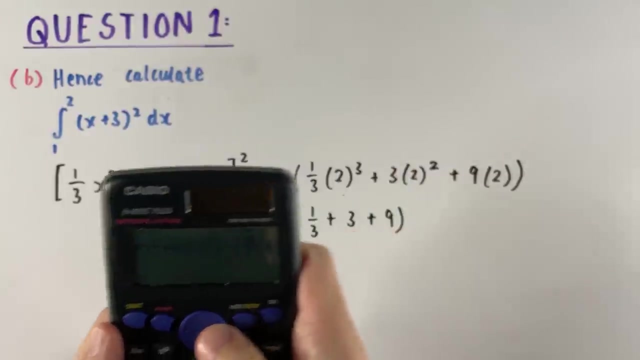 see Plus 9 times 2.. And then we're subtracting. We said a third plus 3 plus 9.. And oops, I've made an error somewhere. I think I've just missed a bracket of some sort. 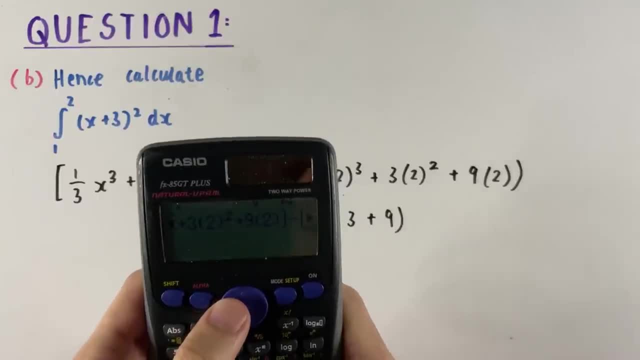 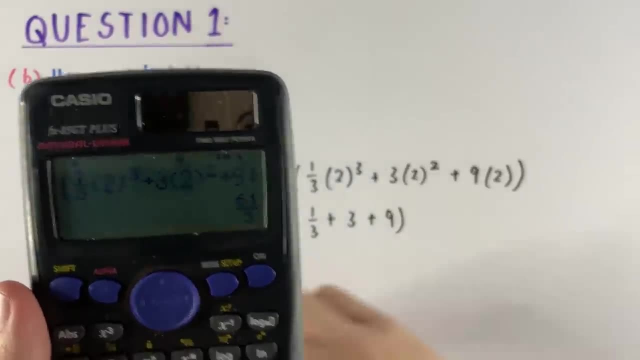 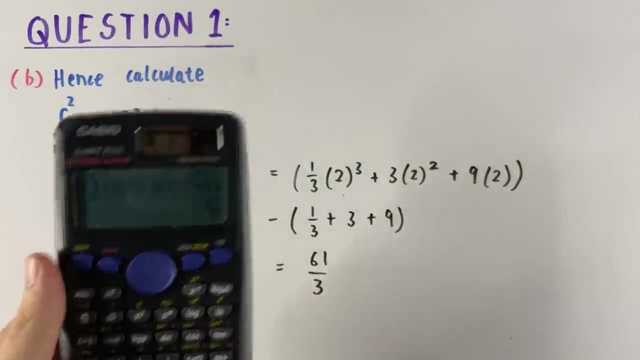 Oh no, I've done an extra bracket. That's what I've done. There we go. That should be it, And we get 61 over 3 as our answer, And that is going to be our final answer for question 1b. 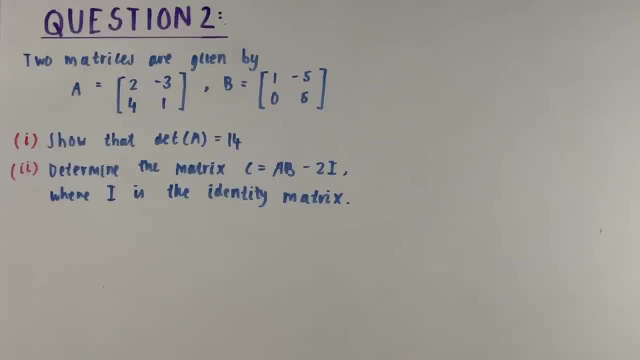 All righty, So moving on to question number 2.. We have what looks to be a question involving matrices, And I love matrices. They are literally one of my favorite things in math. So hopefully, fingers crossed, this question should be approved. 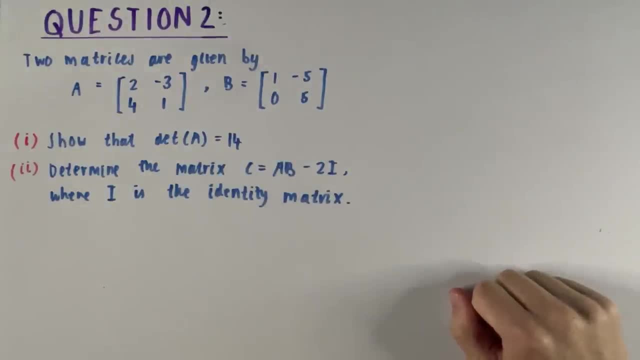 But let's take a look at what the question says. So question 2 says 2 matrices are given by, and we have 2, 2 by 2 matrices, The matrix A given by this matrix here, 2, minus 3,, 4, and 1.. 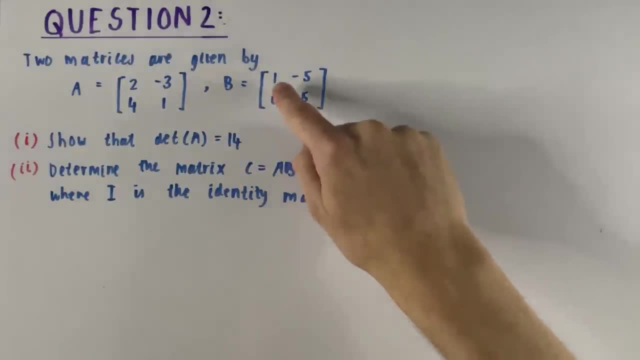 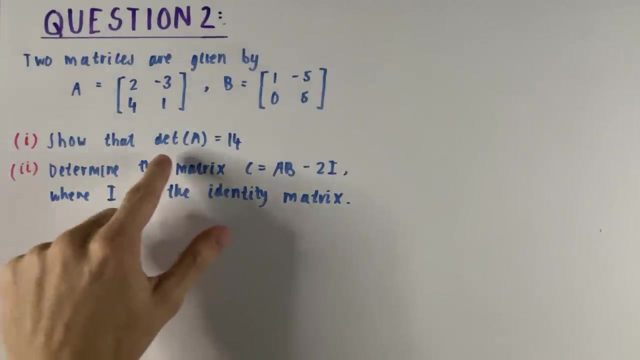 And the matrix B given by 1, minus 1.. And the matrix B given by 2, minus 5,, 0, and 5.. We have again 2 parts to this question. We have part 1 that says: show that determinant of A is equal to 14.. 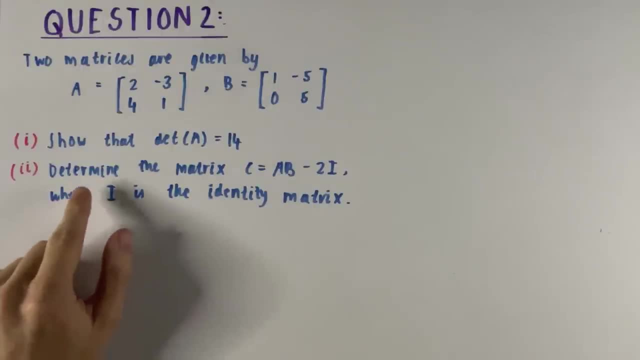 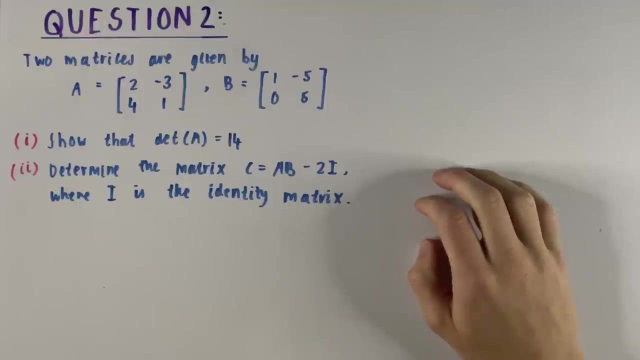 And part II or part 2, that says, determine the matrix C, which is A times B minus 2I, And it even tells us where I is, the identity matrix. So let's attempt this matrices question, or matrix question, beginning with part I. 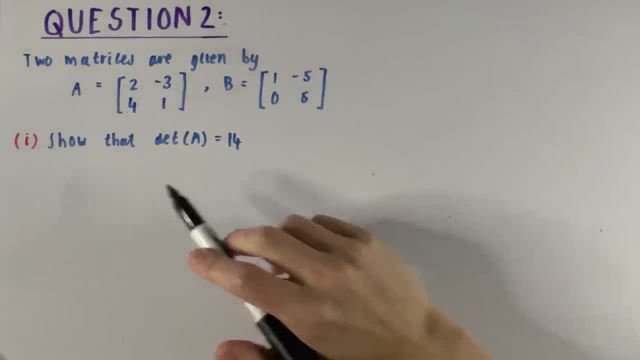 All right. So for the first part, we are asked to show that the determinant of A- this is what this dead a thing means- is equal to 14.. Now, I love it when you get 14.. I love it when you get 16 to 15.. 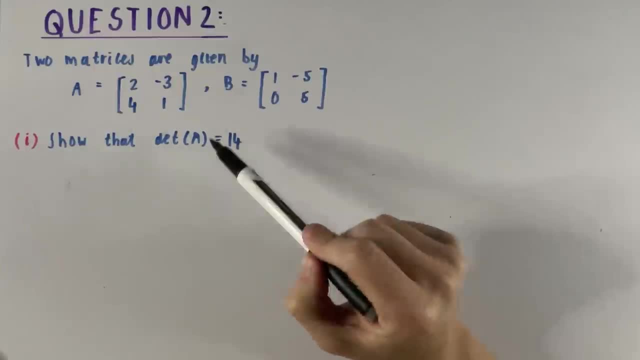 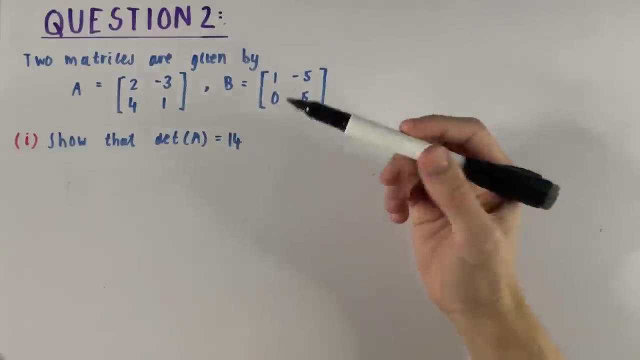 I love it. you get questions that say: show that, and then some sort of equation or formula, because then you know if your answer is correct. So we know, if we get 14 in this question that we have shown it correctly. we just have to do the correct method. Now, as we all know, 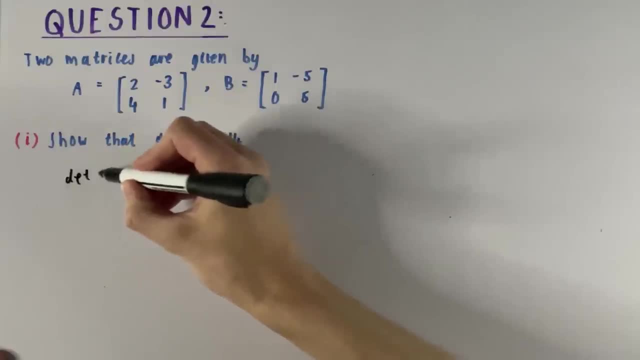 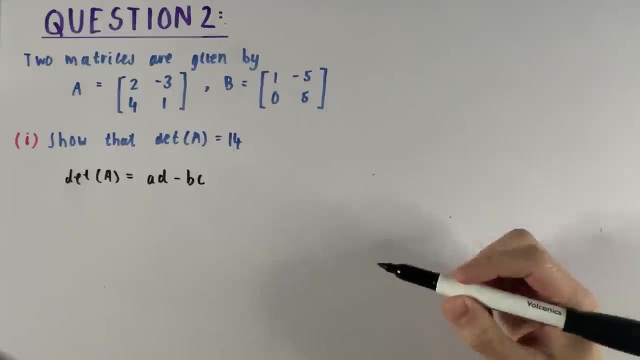 the determinant of a matrix is equal to well. the determinant of a 2 by 2 matrix is equal to a d minus b c, where a, b, c and d are the elements a, b, c and d Now given. 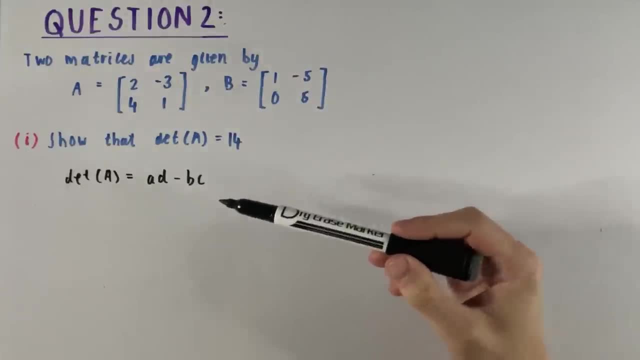 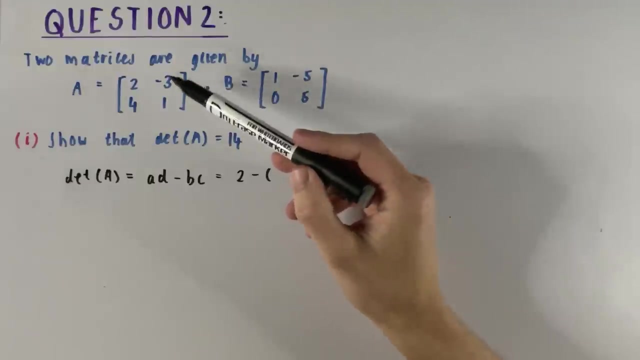 there are- or granted, there are- other methods to calculate the determinant, but in our case this is going to be 2 times 1, I'll just put 2, minus. now we'll do this bit in brackets because we don't want to get our signs mixed up, so we have minus b. 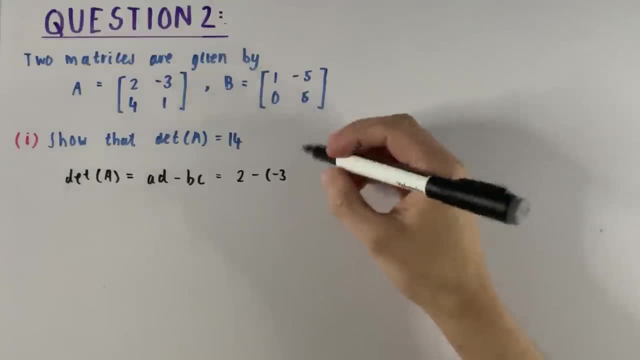 or just b in our case, which is minus 3, times 4,, which is c. So let's evaluate this: We've got 2, and then this is going to be minus minus 12, so it's just going to be minus minus 12, which is just plus 12, which is 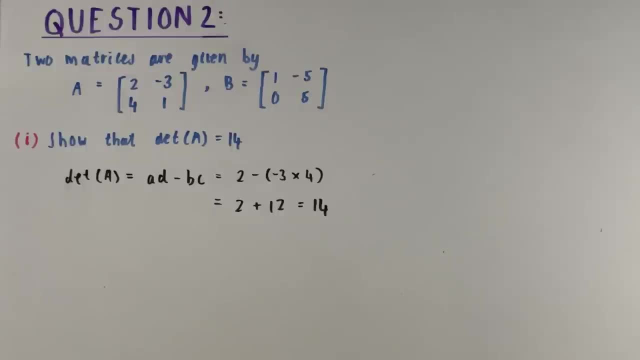 equal to 14.. So that is us showing that the determinant of a is equal to 14.. Now that doesn't look like a lot of working, but because it says show, I figured it just wants us to do the method of calculating the determinant. So I think 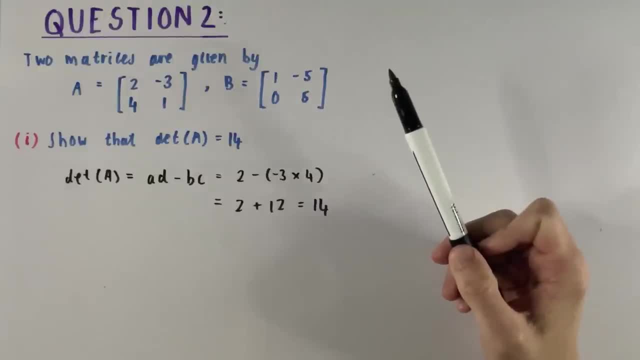 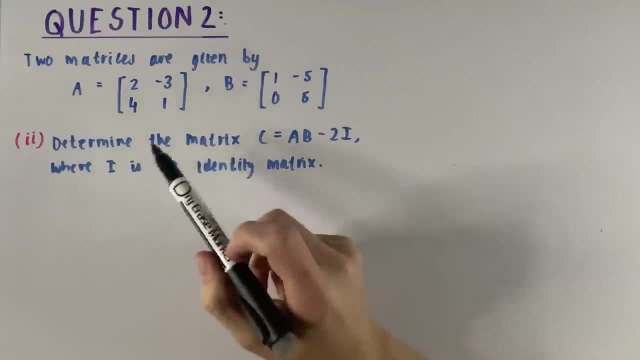 that should be all for that first part, Alrighty. so moving on to part 2.. It says: determine the matrix c, which is given by a, b minus 2i, where i is the identity matrix. so we can look at this matrix c in two parts. We first have 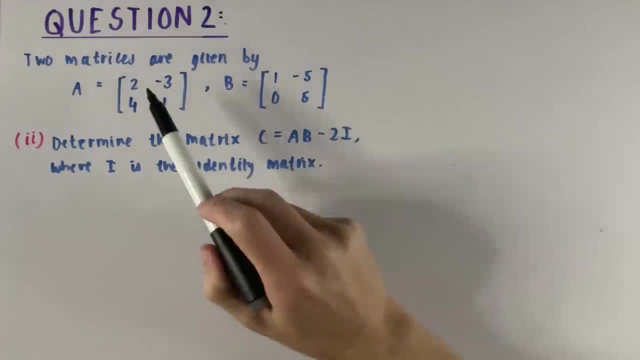 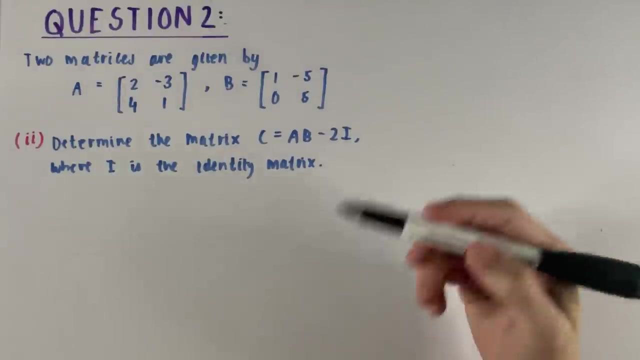 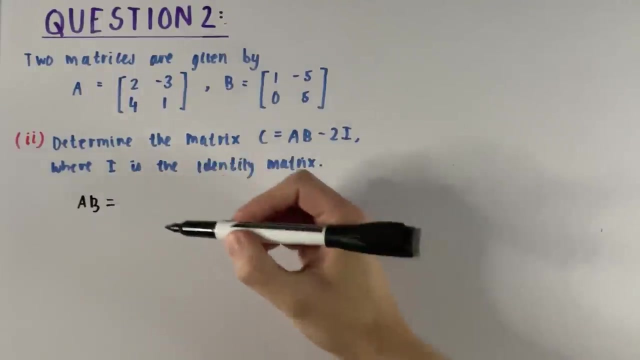 the product product product of the matrix A and the matrix B. And then we are subtracting the product of 2 times the identity matrix, as it tells us. So let's do this in both steps. Let's begin by calculating the matrix a- b, So a b is going to be the matrix A. 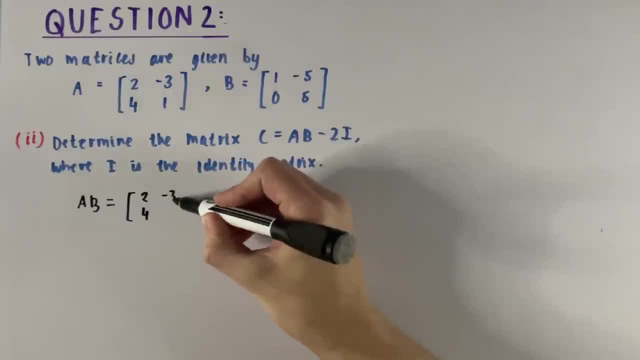 which is 2,, 4, minus 3, and 1,, multiplied by the matrix 1,, 0, minus 5, and 5,, which is the matrix B. Now for matrix multiplication. we multiply the well, the first element in. 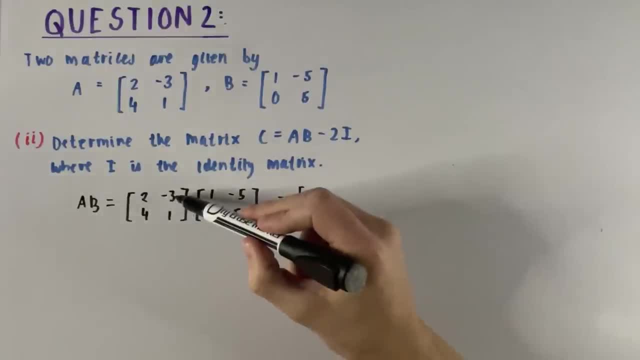 our matrix is going to be the first row times the first column. so we�re going to have 1 plus minus 3 times 0.. So minus 3 times 0 is going to be 0.. 2 times 1 is just 2.. Let's. 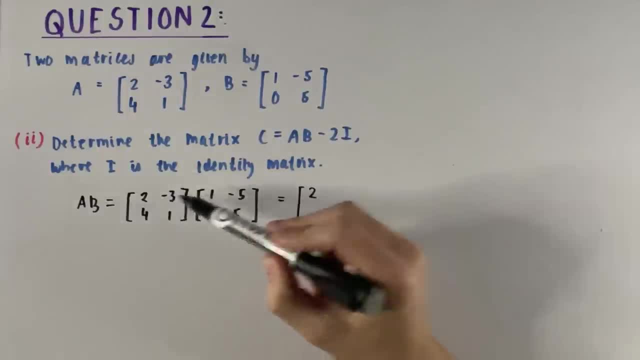 do the top right element, So we do row times, second column. So we've got 2 times minus 5, which is minus 10, plus minus 3 times minus 5,, which is minus 15.. So we have minus 10.. 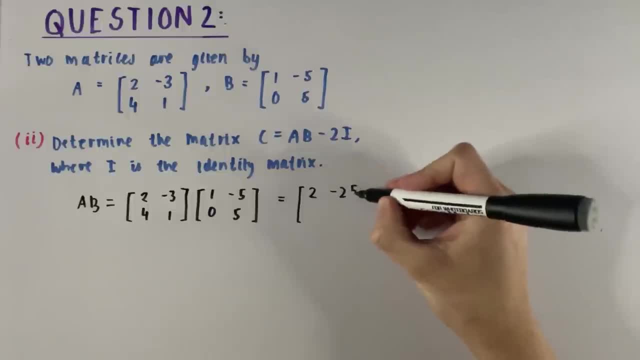 Minus 15, which is minus 25.. Let's move on to the third element. We do the row times the column. So 4 times 1 is 4, plus 1 times 0 is 0. So it's going to be 4.. And the last. 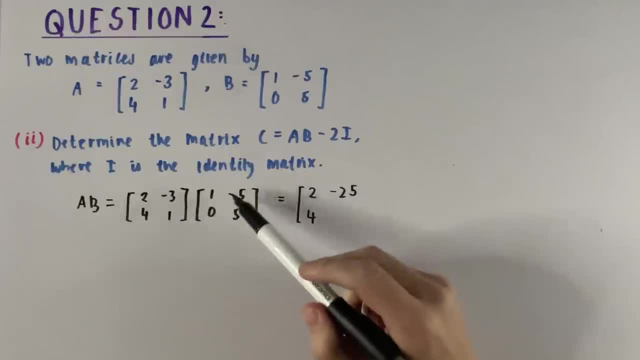 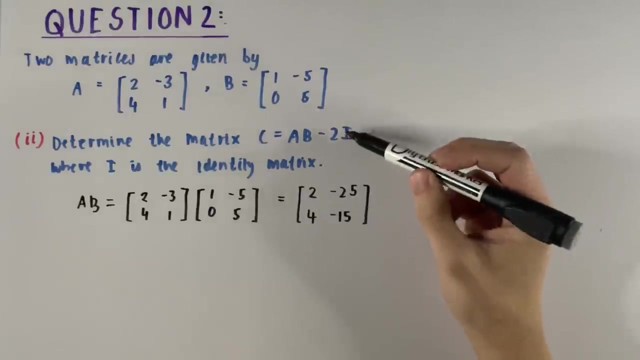 element we do row times column. So 4 times minus 5 is minus 20.. Minus 20, plus 1 times 5 is 5.. That's going to be minus 15.. So that's the first part of C. The second: 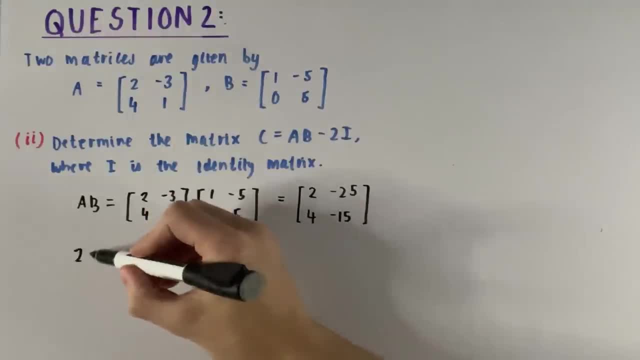 part. we want to work out what 2i is. So 2i is just 2, the scalar 2, multiplied by the identity matrix, which is just 1, 0, 0, 1 with the diagonal. 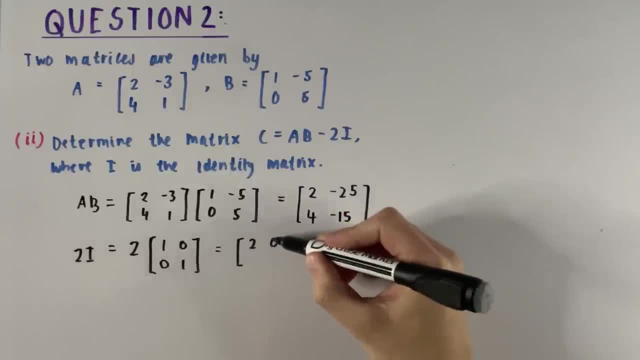 So this is just going to give us 2, 0, 0, 2.. So we can say thus: C is equal to ab minus 2i, which is equal to this thing. here We said it's 2, 4, minus 25, minus 15, minus. 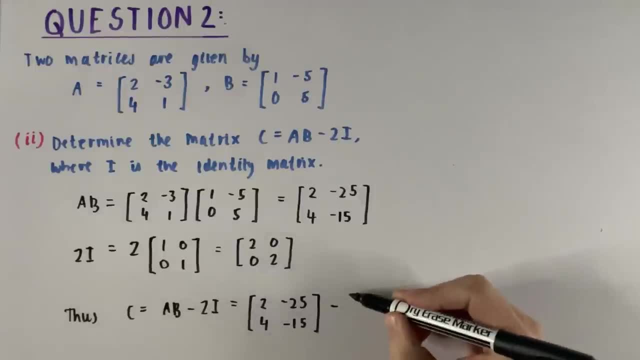 15. Subtract, subtract 2, 0,, 0,, 2, which we can just subtract each element now, So 2 take away 2, 0, minus 25, minus 0, minus 25, 4, subtract 0, is 4. And minus 15, minus. 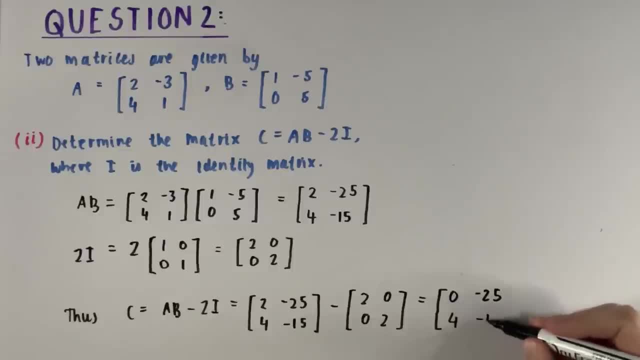 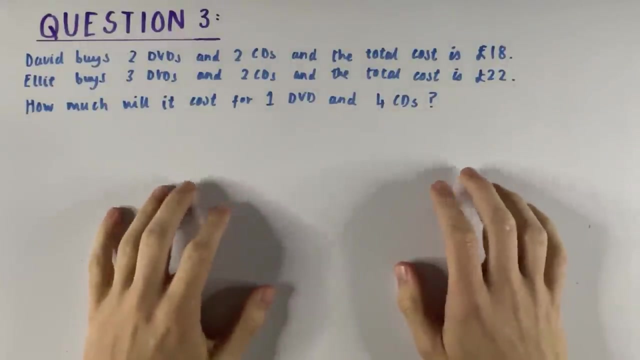 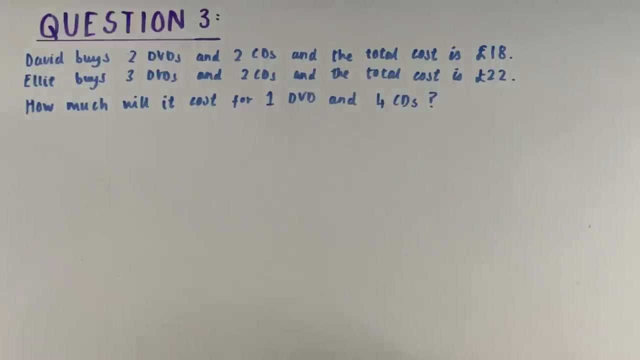 2, is going to be minus 17.. And that there is the matrix ab minus 2i, just like. so The next question, Question 3.. We have this little statement here. It says: we've got David buys 2 DVDs and 2 CDs Boy. this is quite an old question, by the looks. 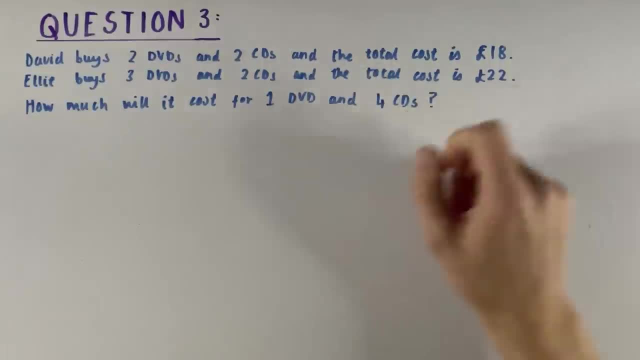 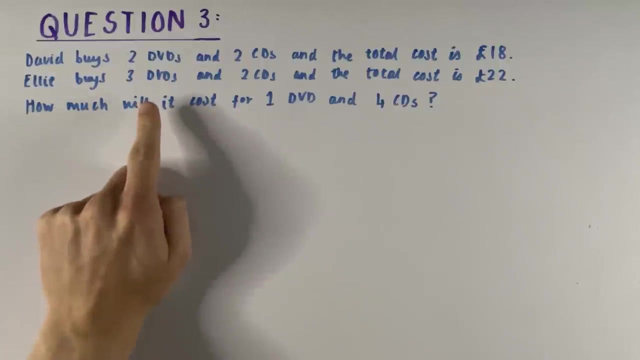 of things, And the total cost is 18 pounds or $18,, whatever you prefer, 18 euros. And we are also told that Ellie buys. He buys three DVDs and two CDs And the total cost is 22 pounds. How much will it cost for? 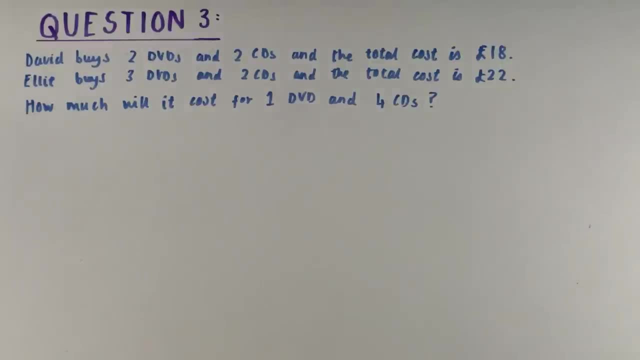 one DVD and four CDs. Now it looks like this is going to require a bit of simultaneous equations, Okay, Which is, by generating multiple equations, we can determine unknowns such as the price or cost of a DVD and the price or cost of a CD. 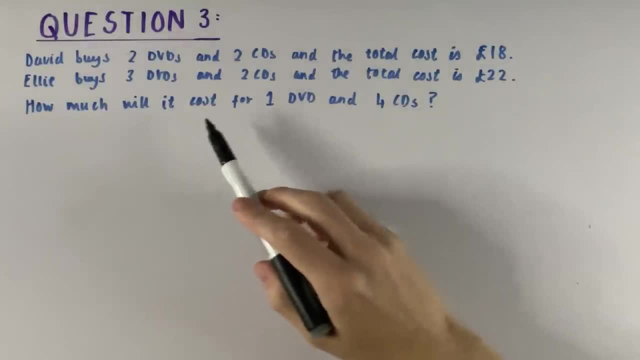 And it looks like that's what we need to do, because we need to also work out how much it will cost for one DVD and four CDs. So let's begin by making a couple of equations from what David and Ellie have bought, So we can say that David, David, David David bought two DVDs- we'll just call a DVD the letter D- and two CDs, which we'll call C. 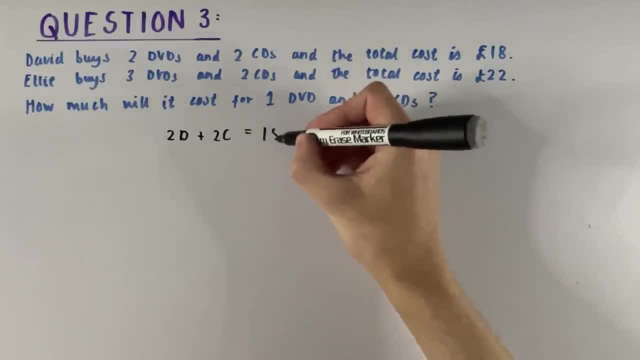 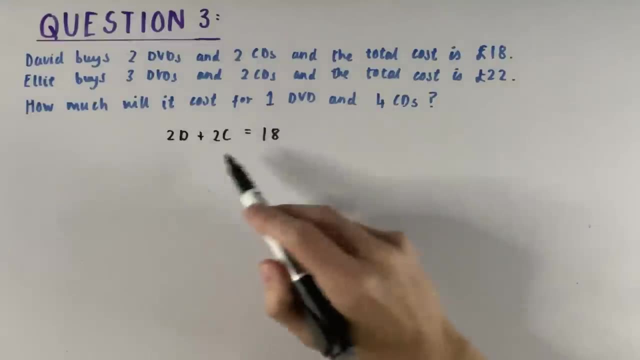 And his total cost was £18.. We'll just, We'll just neglect the pound sign for a moment. So that's our first equation. We're told that Ellie buys three DVDs and two CDs And her total is £22.. So we've got two equations here. 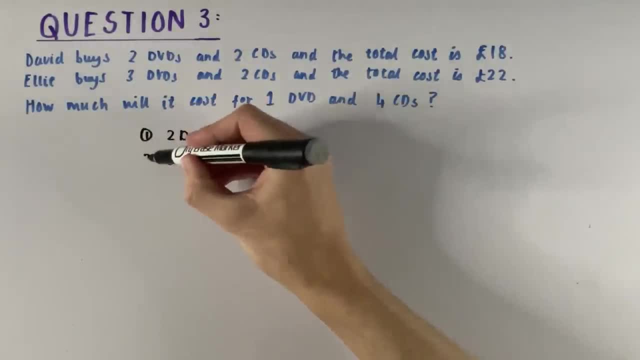 And I'm going to label them one and two just to make it a bit easier for us Two. Now, there's several ways we could do this. We could begin by rearranging the equations for 2C and set them equal to each other. 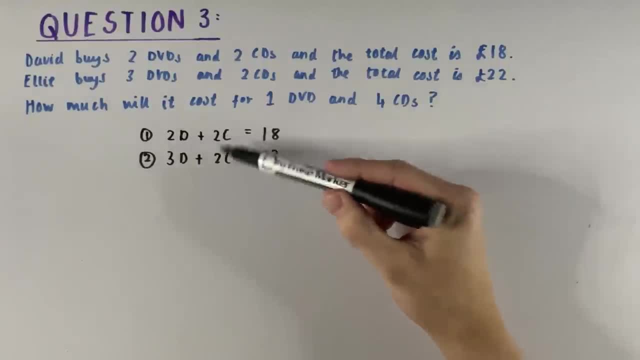 But, but, but, but, but. but. they both have this 2C in them, So we can actually just do equation one subtract equation two, To which, when we do this, we just do 2D minus 3D. 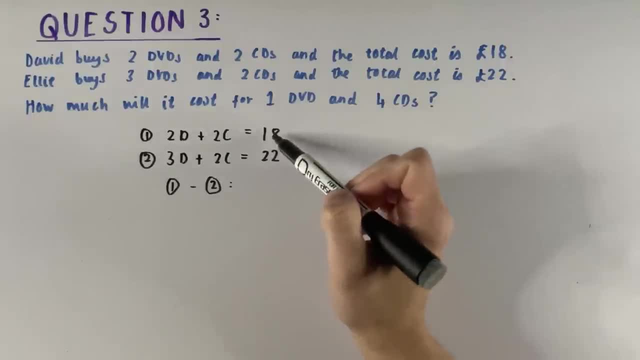 2C minus 2C and 18 minus 22.. And in doing so we will eliminate. eliminate the cost of a CD. So we have negative D, which is 2D minus 3D, and then 18 minus 22 is going to be minus 4.. 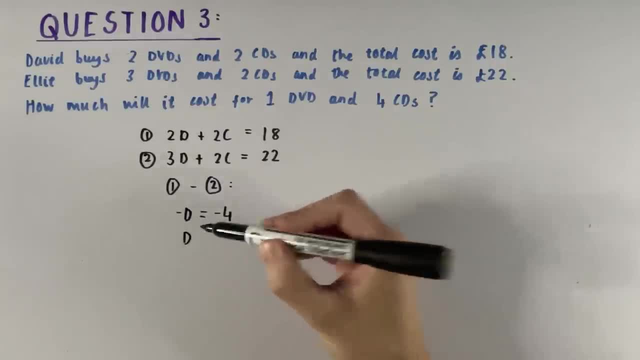 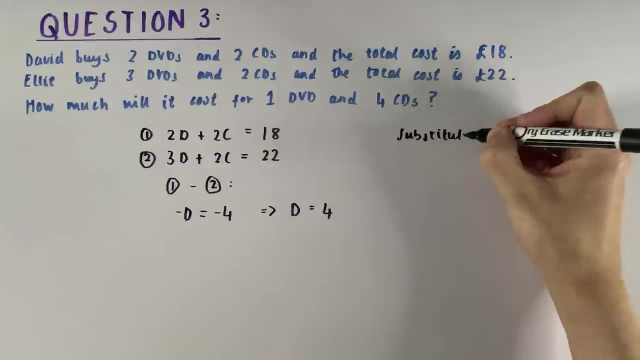 Now we can also just say that they're 4.. Therefore, in fact I'll do this off to the side here- I'll just say that this implies that D equals 4.. Now we can substitute, substitute D equals 4 into one of these two equations. 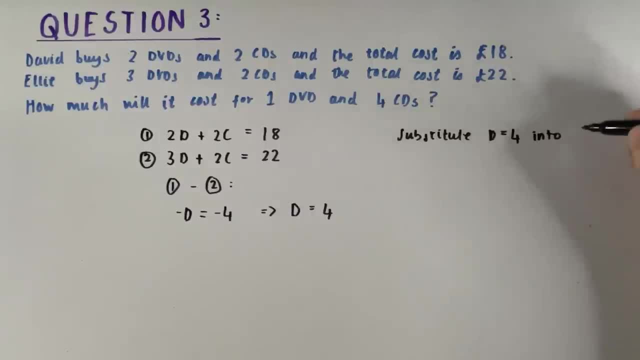 I'll just go Into equation one. two, Evaluate what C is. So we have 2D, which is 2 times 4, plus 2C is equal to 18.. So we get 8 plus 2C equals 18, or 2C equals 10.. 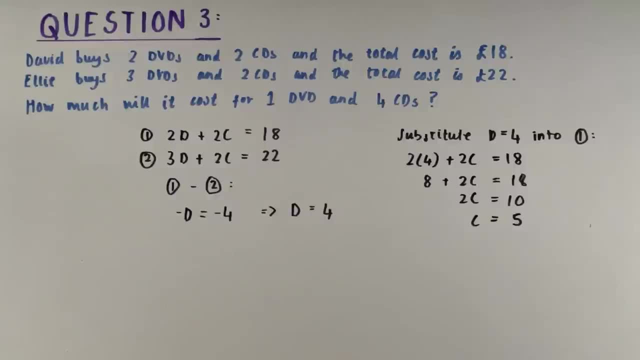 So therefore, C equals 5.. So in doing this, we have evaluated that a DVD cost £4, and a CD cost £5.. Now the good thing is, we can actually check if this is correct by substituting them both back into each of the prices to see if they do cost 18 and 22.. 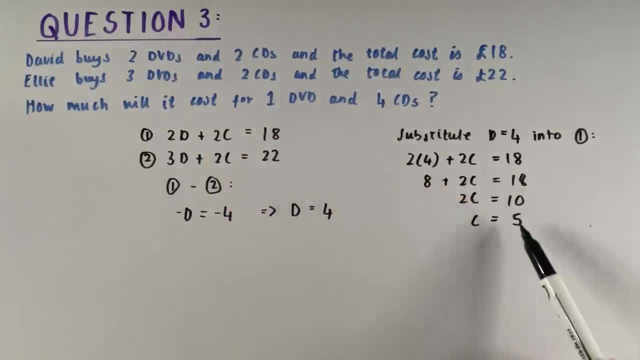 So 2 of each is going to be 8 and 10,, which is 18.. And then 3 and 2 is going to be 12 and 10,, which is indeed 22.. So we know we're doing this right. 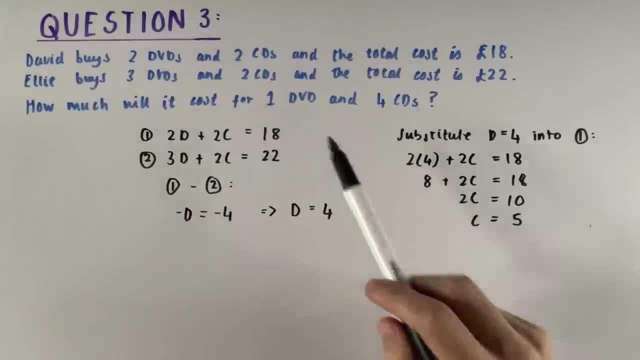 However, now we need to work out how much it will cost for one DVD and four CDs. So we have this equation- Let's call it equation three, which is 1D or just D plus 4C. We can sub in our values. 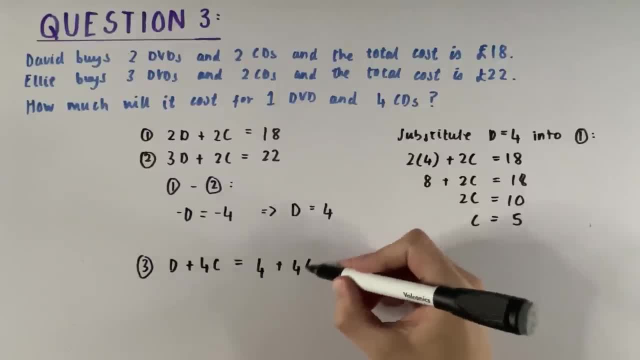 D is 4.. C is 5,, so plus 4 times 5.. So this is going to be 20 plus 4,, which is 4.. So we can say thus: one DVD and four CDs will cost. 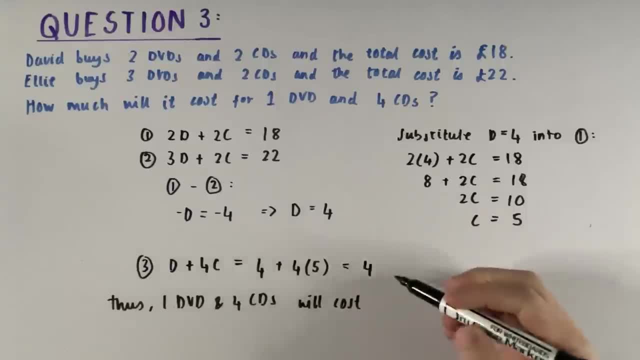 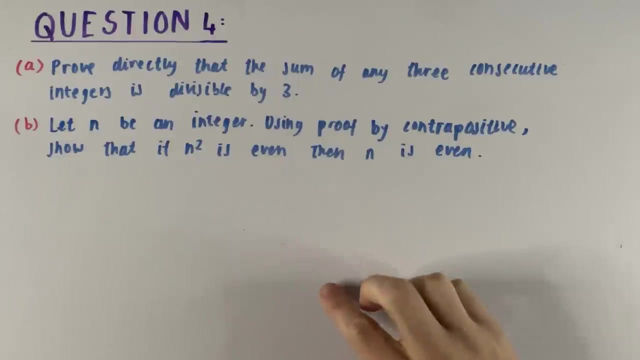 .4.. Why did I put 4? I meant to put 24.. Will cost £24.. And that is going to be the end of that question. there For question number 4.. 1,, 2,, 3, 4.. 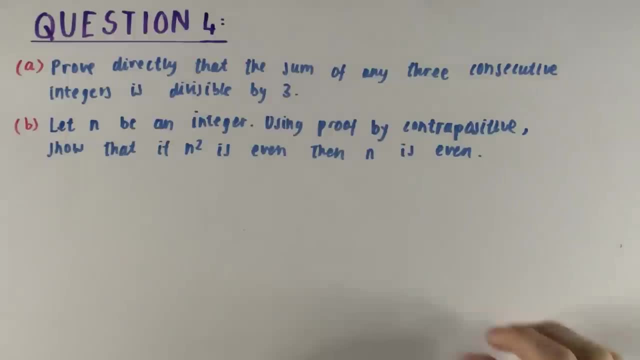 We have a couple, couple, couple, couple, couple of of of of proof questions- Probably my least favourite thing in math. However, they come up a lot, So we will tackle them as best as we can. 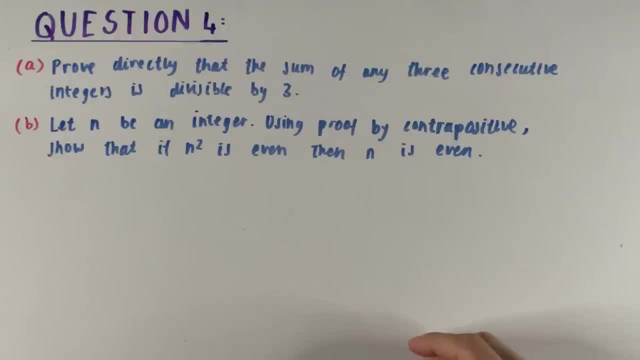 So the first part, part A. We have proof directly that the sum of any three consecutive integers- consecutive integers- is divisible by 3.. And then for part B. By the way, do you know what the best thing about part B is? 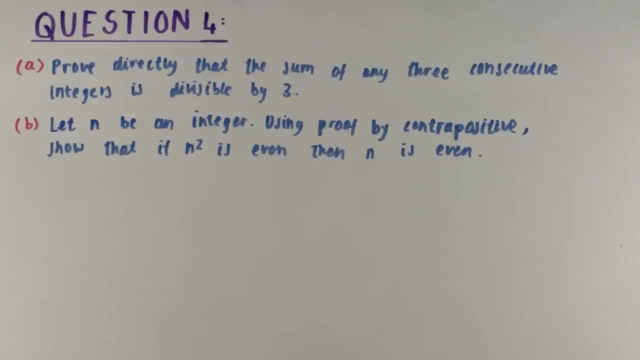 It comes after the part A: Okay. So part B says: let N be an integer, using proof by contraband and positive Show that if N squared is even, then N is even. Okay. So let's tackle, tackle, tackle, tackle, tackle. 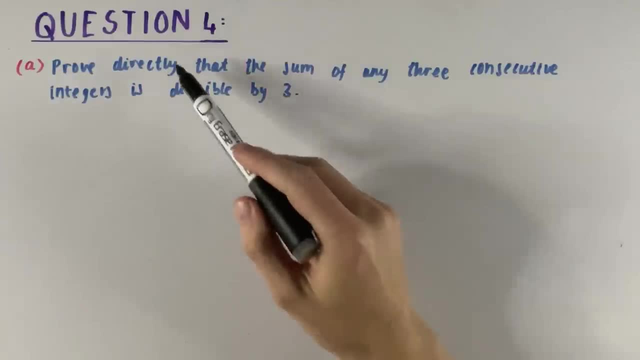 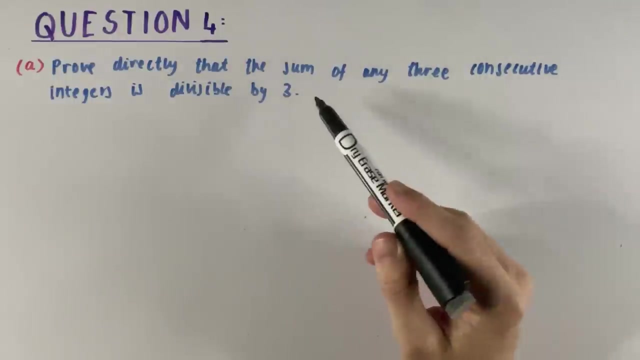 the first proof And we are asked to prove directly. So we have to do this proof, um well, direct. So we are told that the sum of any three consecutive integers, so one integer plus another integer plus another integer, 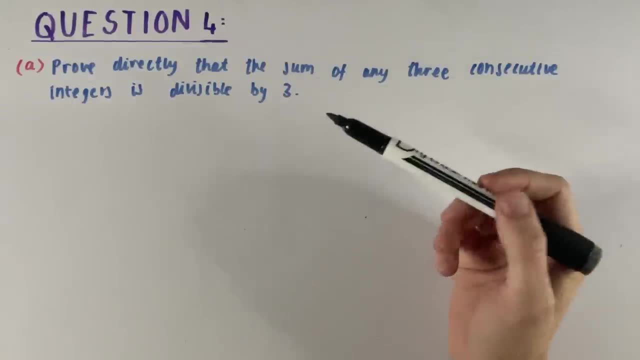 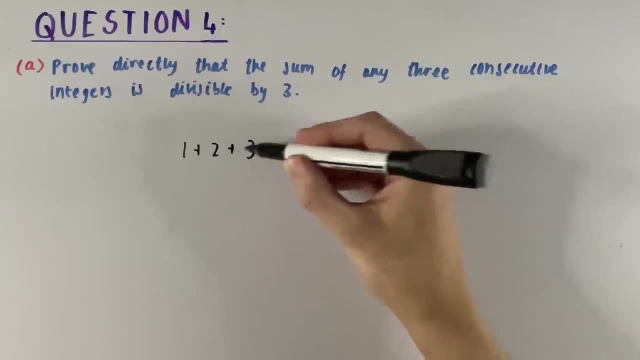 one after the other. so 1,, 2, and 3,, for example, is divisible by 3.. Now we can see that this is true. That gives 6,, which is divisible by 3.. 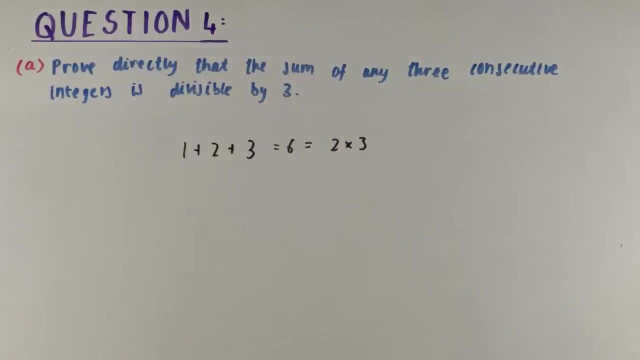 That's 2 times 3.. But that's not good enough. We have to show that this works. We have to show that this works for all integers. So let's begin by picking a few integers. So let's make our integers. 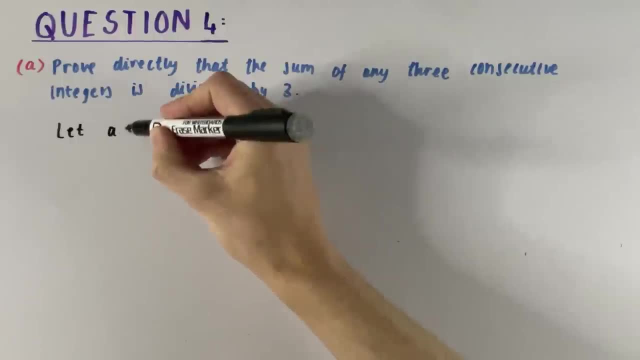 Let's say: let let's say A equals. let's say A is equal to N, Some integer. We'll say B is equal to the number before N. Let's say N is our 2.. The number before 2 is going to be 2 minus 1.. 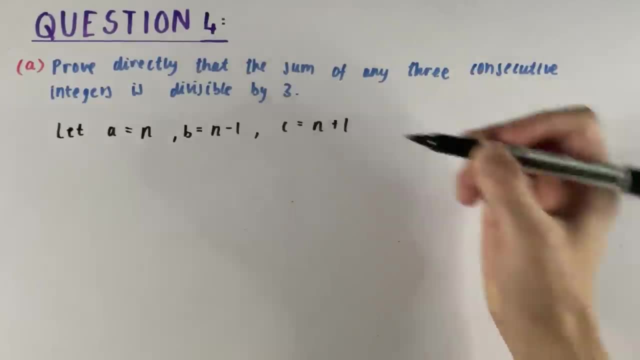 And we'll say C is going to be N plus 1.. Now we have to let A, B and C be an integer. So we must state where A, B and C are integers, And that's what this little thing here means. 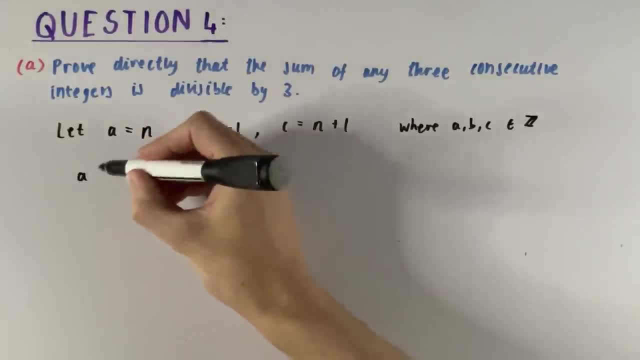 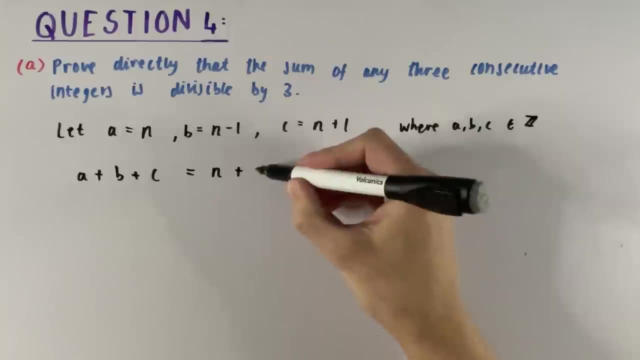 So let's do the sum of this. Let's do A plus B plus C, So this is going to be N plus. we'll do N minus 1 plus, and then N plus 1.. Like so, And this is equal to. 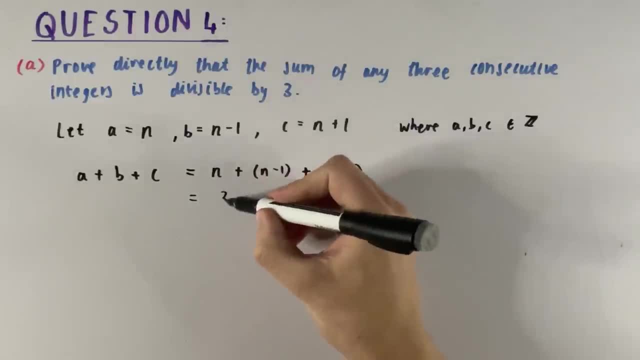 we've got N plus N plus N, which is 3N, And then we're going to have minus 1 plus 1, which is 0. So A B plus C or A plus B plus C. sorry. 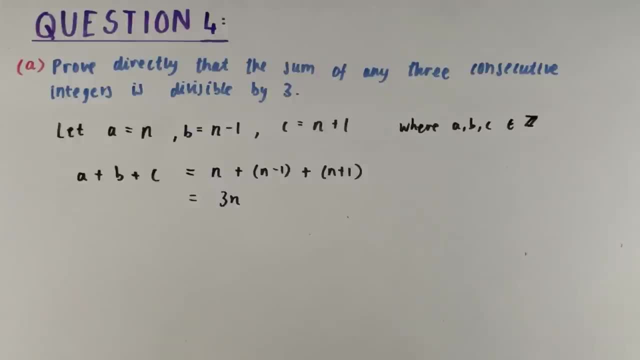 is going to be 3N Now, as we said. oh wait, we need to actually say N is an integer. Forgot to mention that. so we can see that this is equal to .3 times an integer. 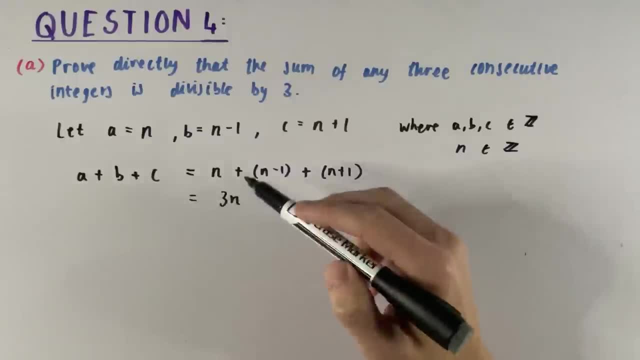 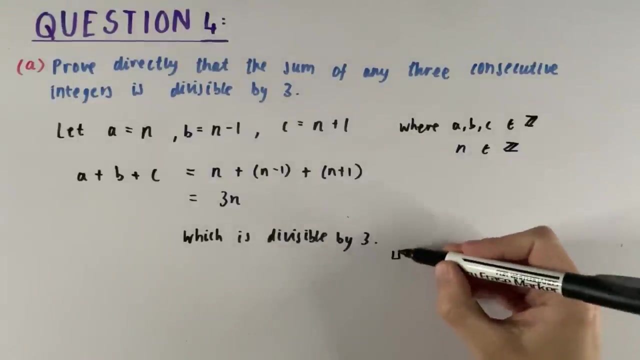 Which is obviously divisible by 3.. Because we've got this scalar 3. So we can just say which is divisible, divisible by 3.. And this is actually enough for the little proof here. 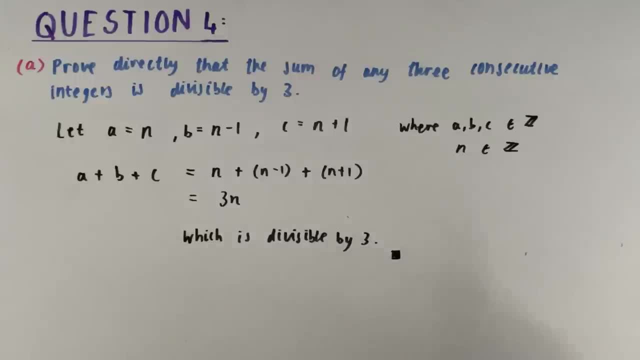 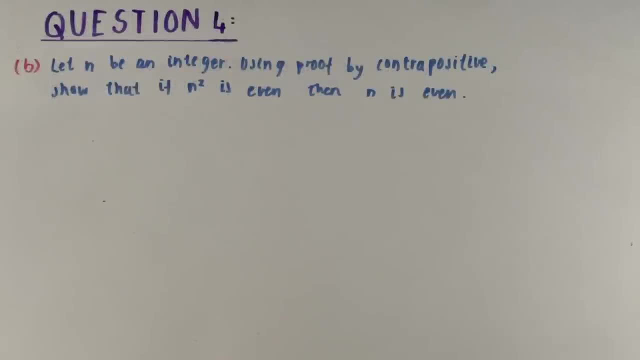 Because we're just told to proof directly, so we don't need to do any more. That has done it All in that statement there. Okay, so for part B. Part B, We are told: let N be an integer. 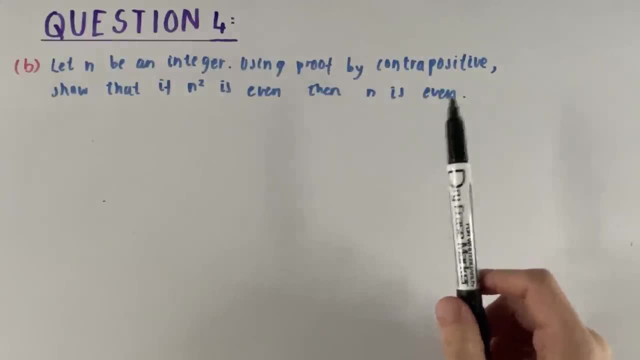 And by using proof by contrapositive, which I'll explain in a wee moment what that means. We are asked to show that if N squared is even, then N is even. So what does this? 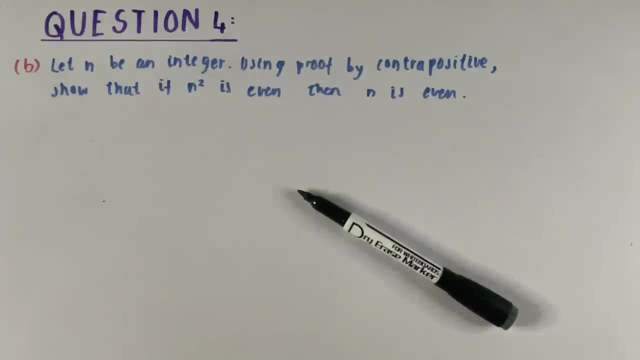 proof by contrapositive mean. Well, essentially, what it means is take our statement. our statement here is: if N squared is even, then N is even, And it basically means contradict. 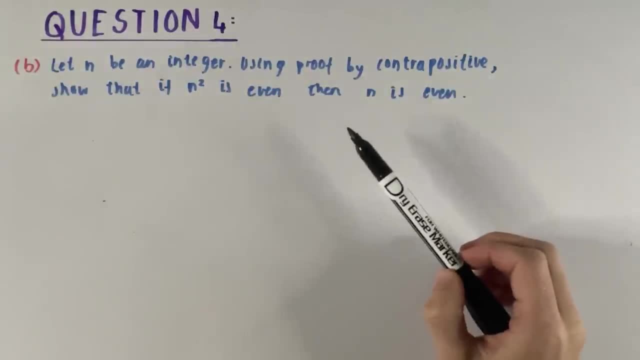 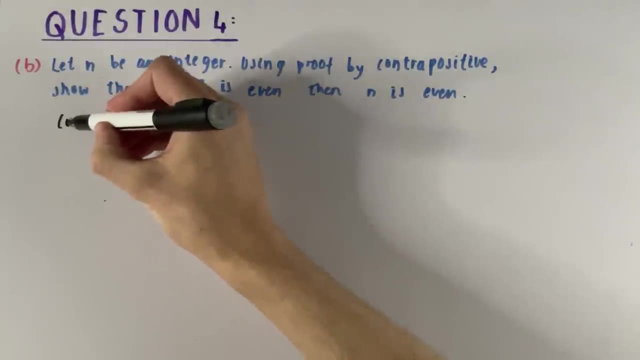 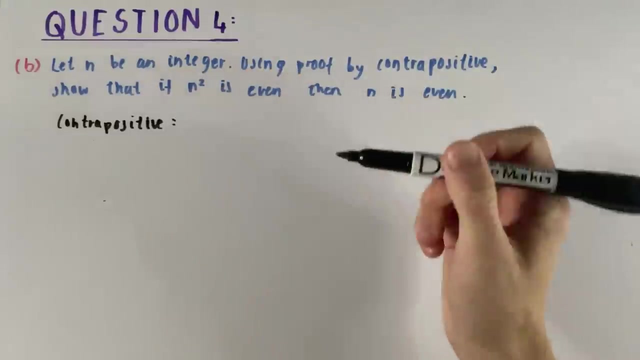 or do the converse of the opposite of this. So, in our case, our contrapositive statement. let's write out what it's gonna be: The contrapositive. I'm not very explaining this very well. 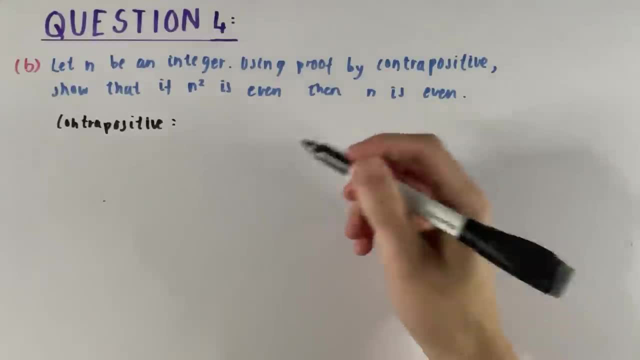 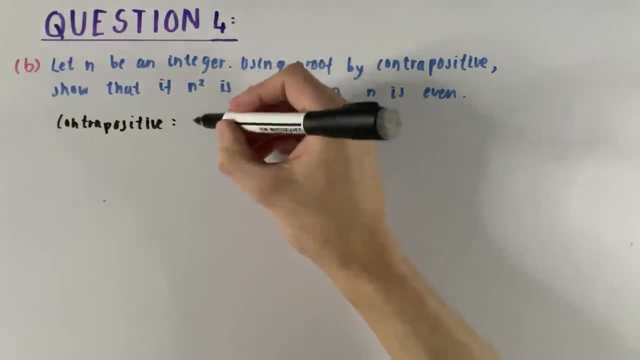 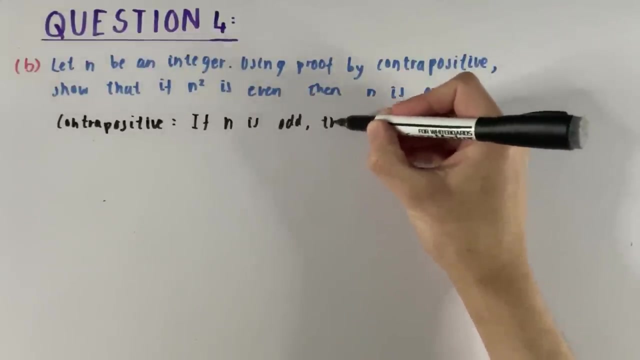 but you'll see when I write this out. It would be flip this around and change the even to odd. So our contrapositive is: if N is odd, then N squared is odd. 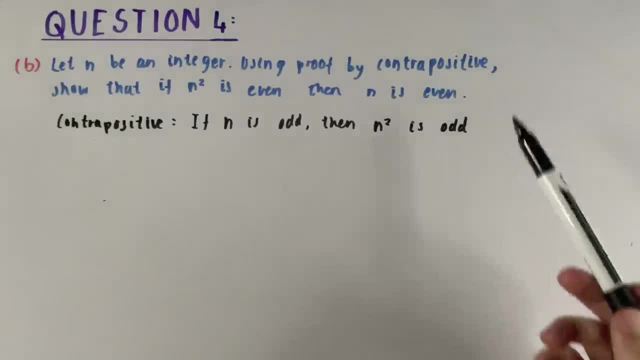 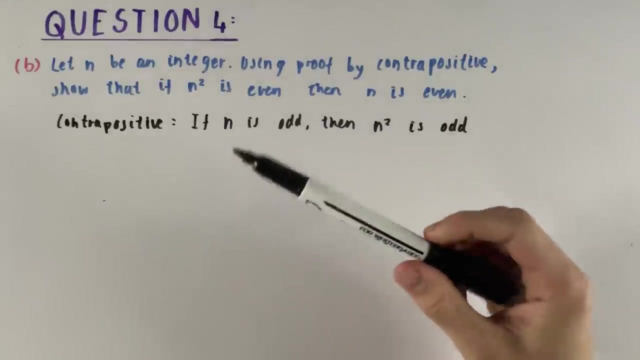 And by doing this contrapositive. if it proves that it holds, then this statement here also holds. So let's give this a go, shall we? So if N is odd, so N is our integer. 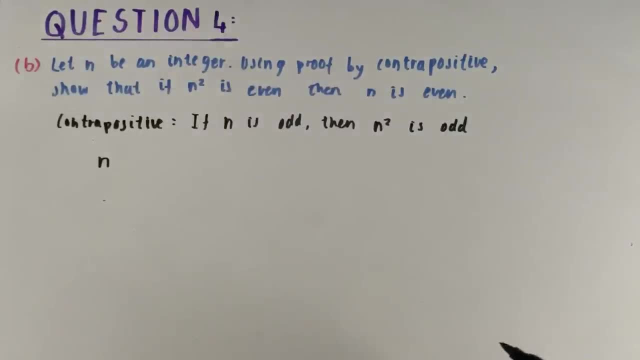 as we're told in the question. now, if we want to pick an odd number, we know that two times any number is an even number. For example, two times three is six, two times four is eight. 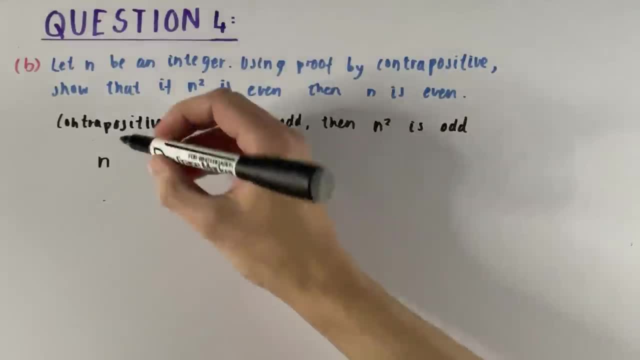 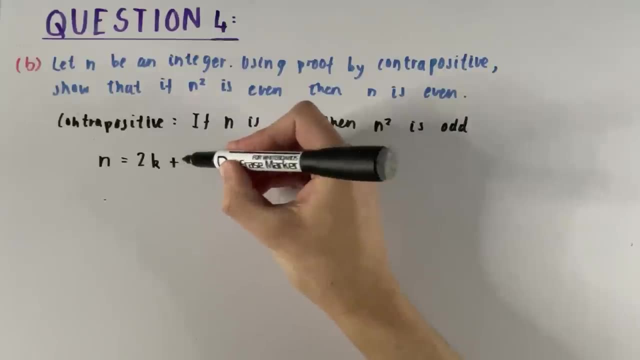 you'll always get an even number if you multiply it by two. However, if you add one to this even number, let's say k add one, you will always get an odd number for any integer k. 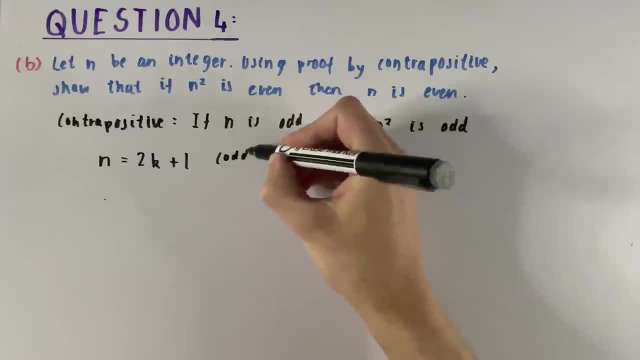 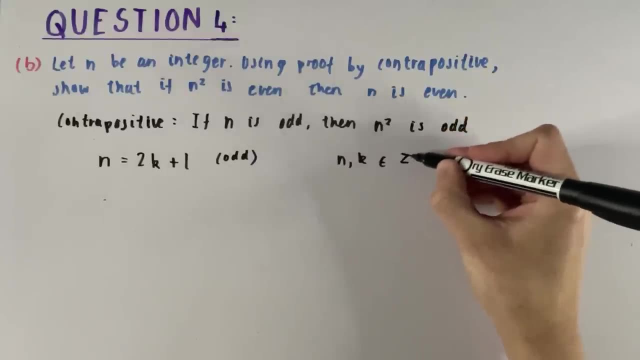 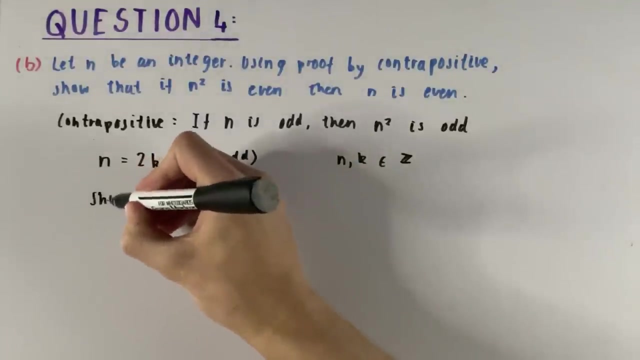 So this is an odd number. Now we need to say that N and k are both integers in this case. So let's we want to basically, using this, show that N squared is odd. 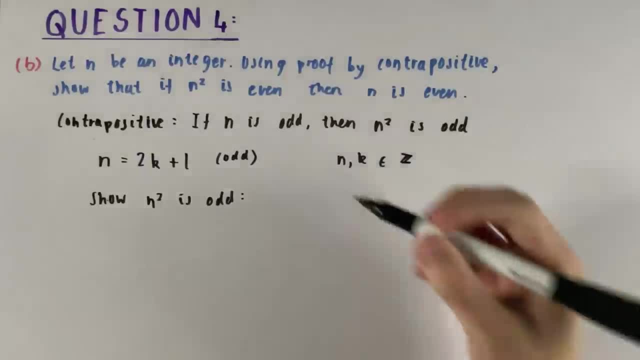 So let's do that, So let's calculate what N squared actually is. So it's going to be two k plus one squared, which is just we're going to have. 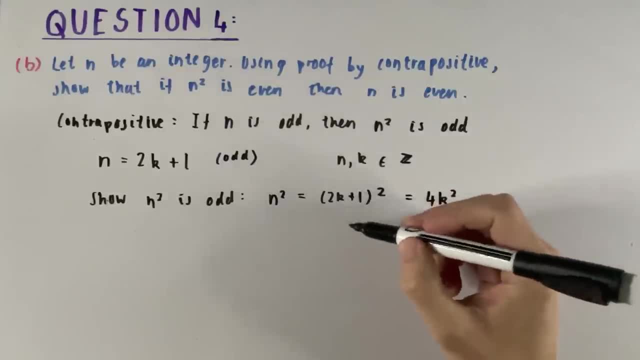 four k squared. squared the first term, add the second and third terms, which is going to be plus four k, then one times one is going to be plus one. Now we want to show that. 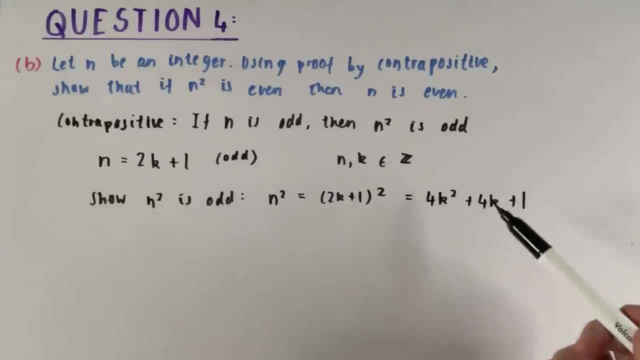 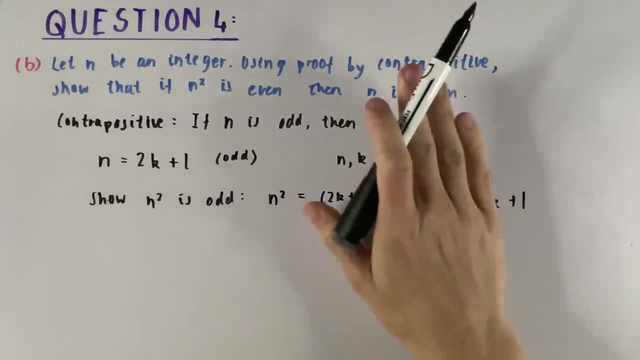 this number here is odd. So, using what we did before, we want to show that two times some integer plus one. Now we've got this little plus one at the end, So we want to show that. 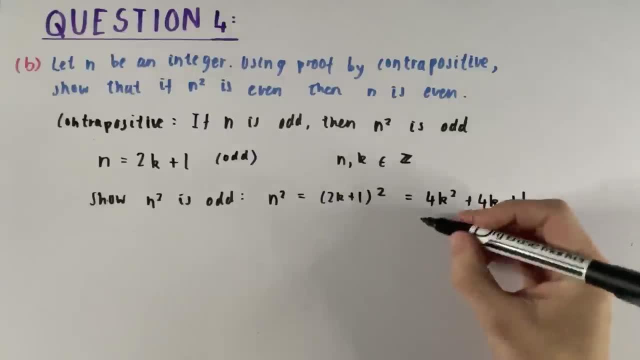 this part here can be made with a multiple of two, So let's take out two and write what we've got. now We're going to have two k squared because two k squared. 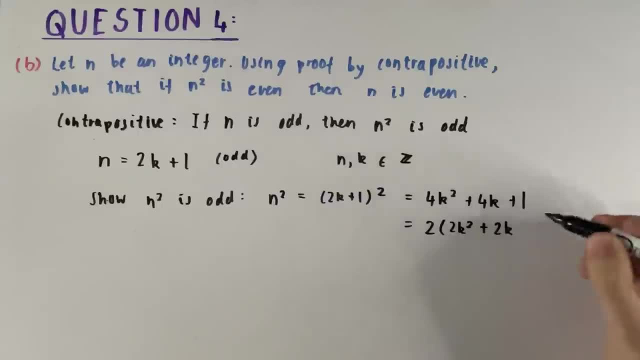 times two is four k squared plus two k. That gives us four k plus one. Now we said k is an integer. So no matter what, this is because we're multiplying it by two. 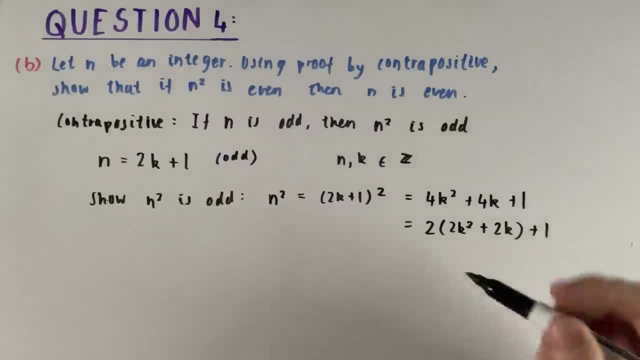 we can't even number and we're adding one, So we say this is odd. So therefore we can say so the contrapositive statement. that's what we wrote at the top here. 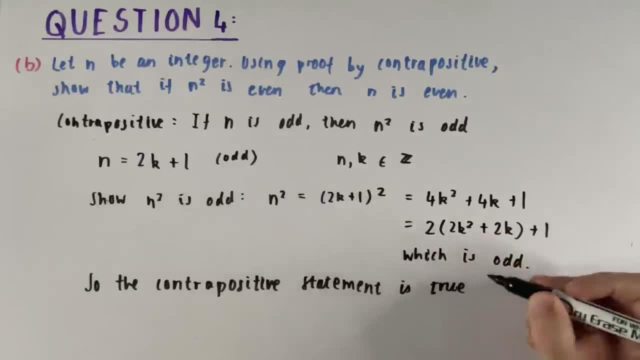 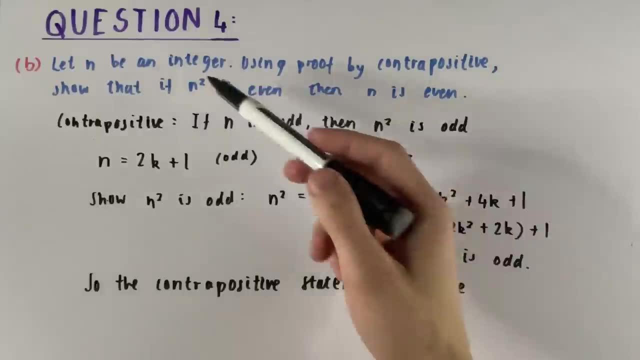 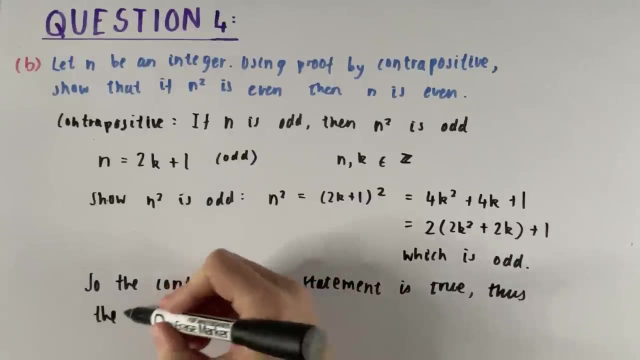 is true And by doing this proof by contrapositive. if the contrapositive is true, that means that the original statement is true. So we'll say that's, the original statement is also true. 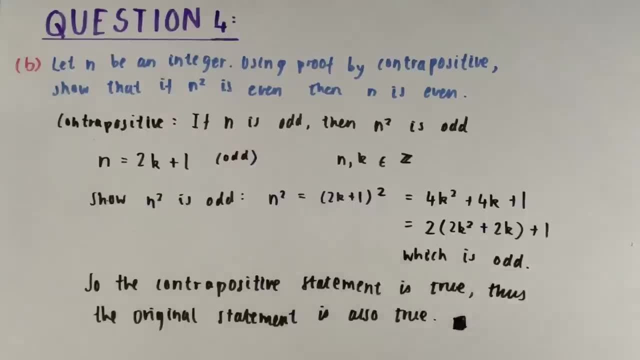 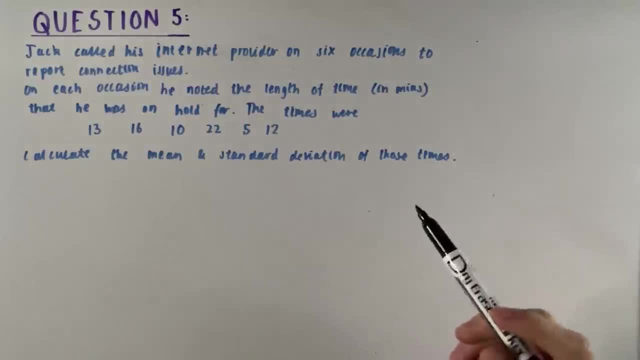 Like so, And we'll do our little proof symbol at the end. Next up, it looks like we are going to be doing a bit of statistical analysis: Statistical statistical statistical statistical analysis. 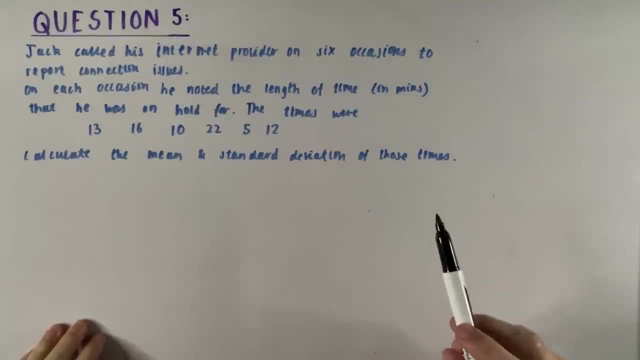 I quite like statistics, So question five. We've got this big wordy question. It says Jack gold, his internet provider, on six occasions to report connection issues. Been there, Jack. 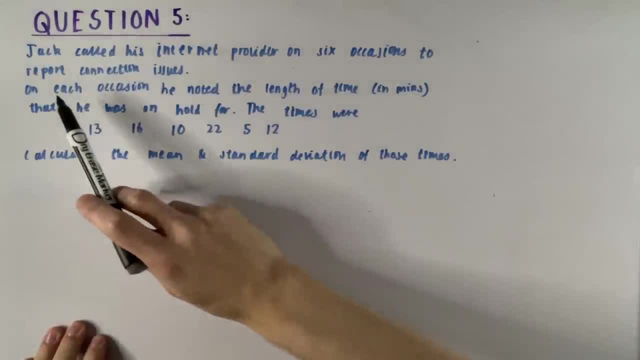 I feel your pain. On each occasion he noted the length of time in minutes that he was on hold for. The times were thirteen minutes sixteen, ten, twenty-two five. 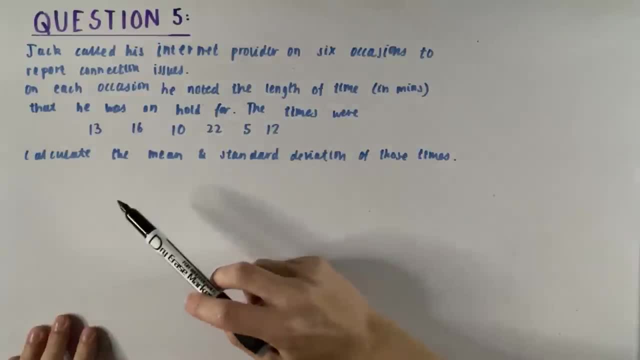 and twelve. Boy, that twenty-two time must have been very bad. Then we're asked to calculate not only the mean but also the standard deviation of those times. Okay, We might have to do quite a lot of calculating here, so I hope I have. 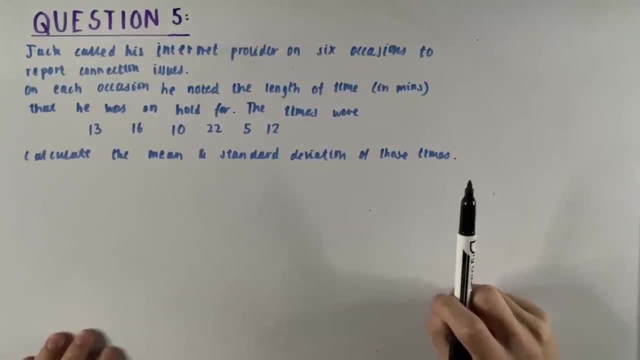 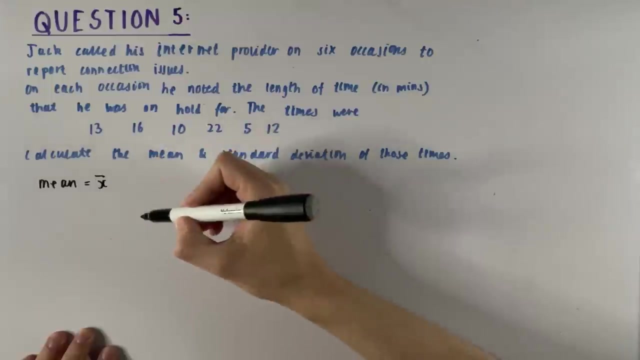 left enough space. but let's begin by calculating the mean. So what is the mean? Well, the mean which we're going to give this symbol here, X with a little bar on top. 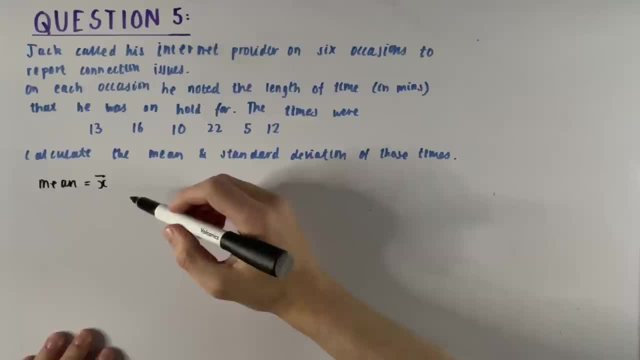 which just is the symbol for the mean, And that is just the average, or yeah, the average, of all these numbers. So we can use the formula X1 plus X2.. all the way up to 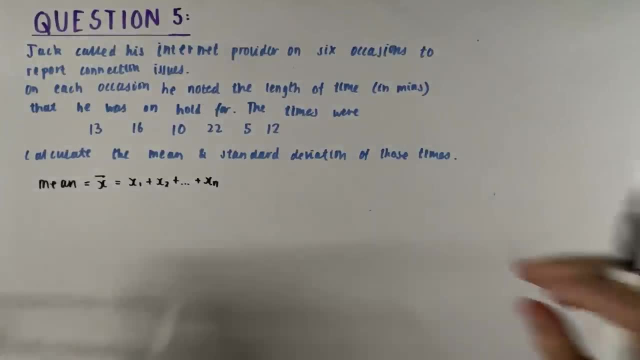 X sub N divided by N. Now this just means for all of our values up to N. N in our case is six. because there's six values, We want to add them all together. 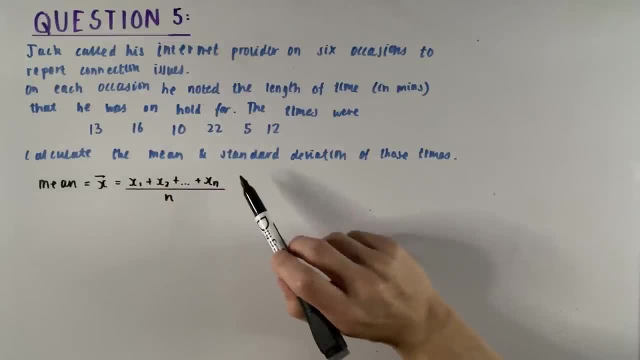 and divide by the number of just the amount of quantities we have, which is six. So in our case this equation is going to be thirteen. I'm actually going to do it just below. Let's do it down here. 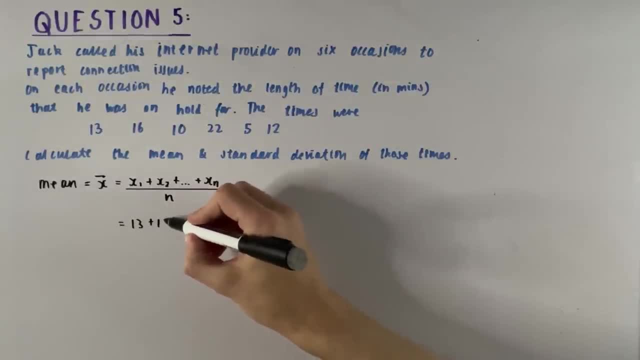 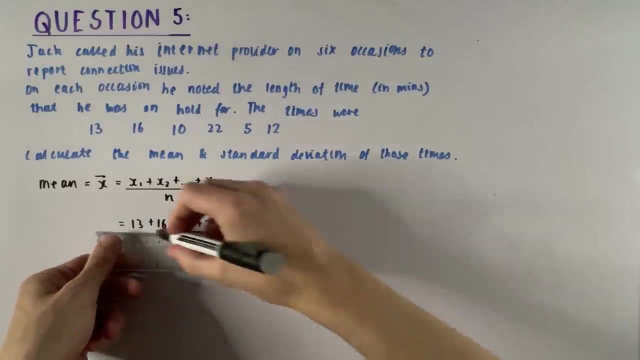 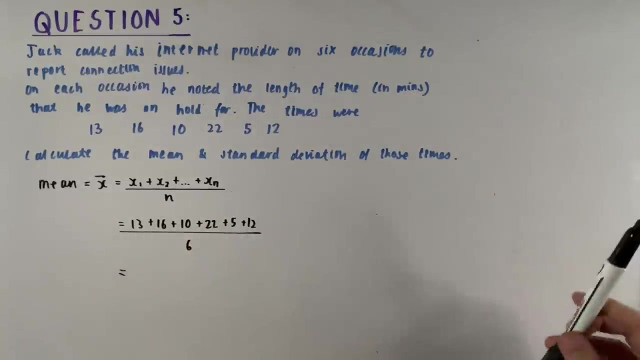 So this equals thirteen plus sixteen plus ten plus twenty-two plus five plus twelve divided by six Like so Now we could plug this into a calculator. so let's do that. 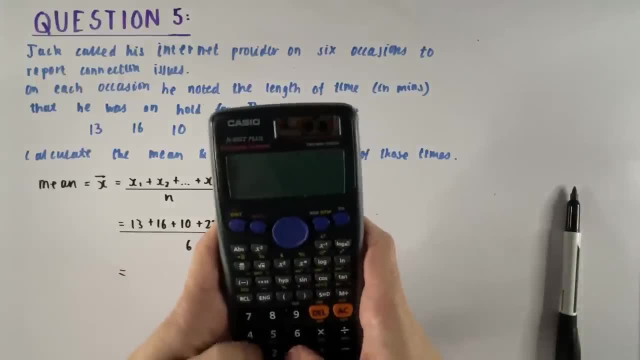 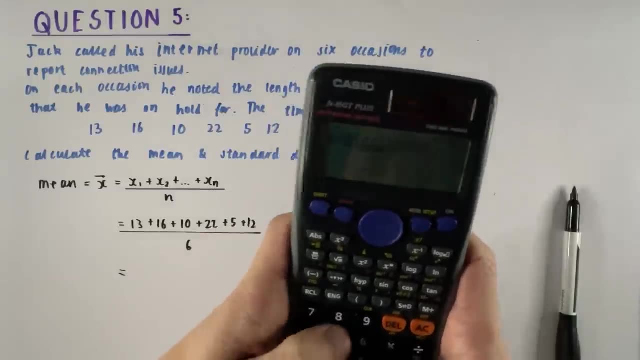 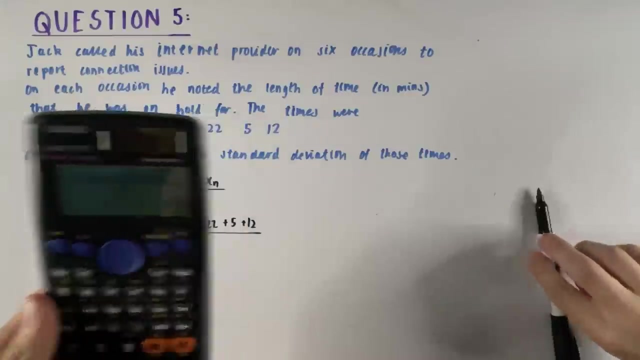 Let's add all these values together, Thirteen plus sixteen, ten, twenty-two, five and twelve, then six on the bottom, Gives us a mean of thirteen mins. So that's our mean. 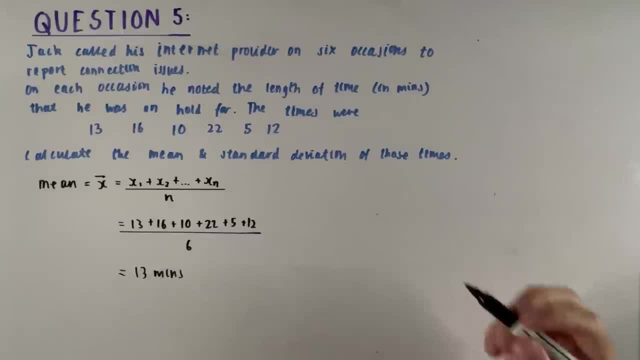 Now, moving on to the standard deviation, We can use a formula to calculate the standard deviation which is given the letter S, but a lot of the time you might see this symbol as well. 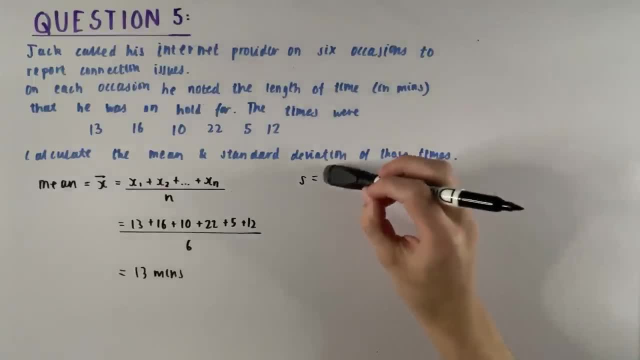 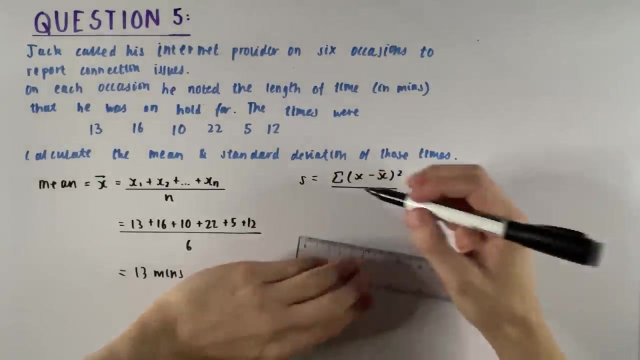 But in our case we'll just go for S. And it is given by the sum of the difference between each value and the mean squared divided by the number of values. 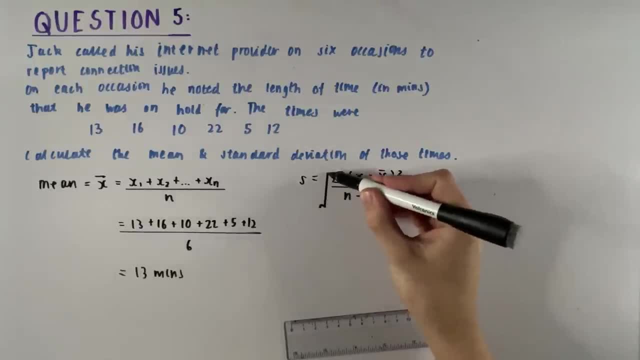 subtract one, And we want to also do the square root of all this. So we've got this big long formula that seems quite, quite intimidating, But it's not too bad once we get going. So let's begin by working out. 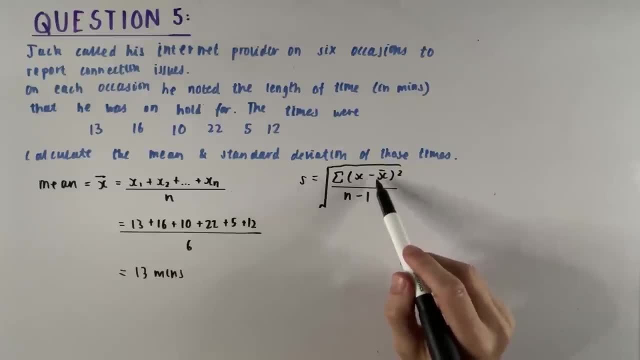 the sum of the difference between each value subtract the mean squared, So we can set up this little um array of numbers, or set of numbers, which is going to be. 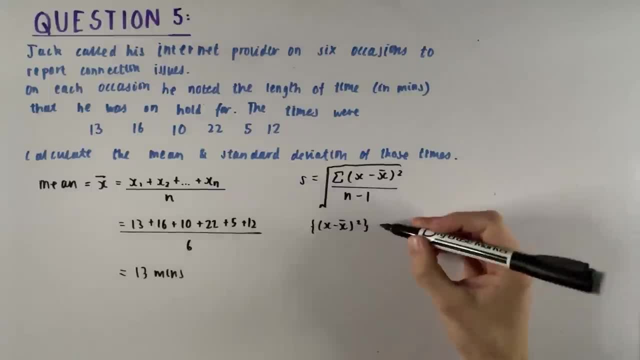 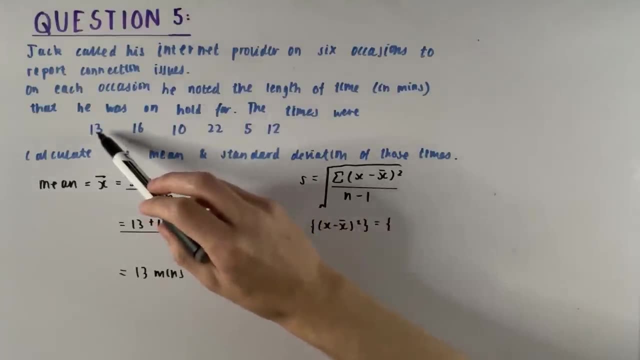 minus X bar squared, And this will give us. what we need to do is, for each value, we want to substitute that in as X and then the mean in as X bar and square it all. 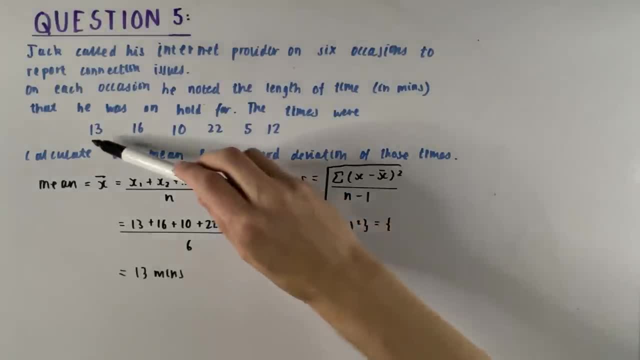 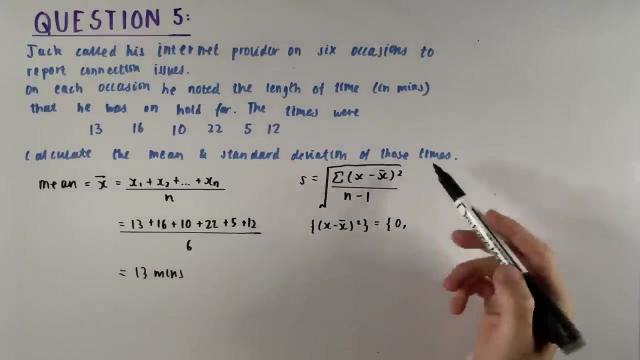 So we can do this without a calculator. actually, Let's start with 13.. 13 minus 13 is 0.. 0 squared is 0.. The next value we've got 16.. 16 minus 13. is 3.. 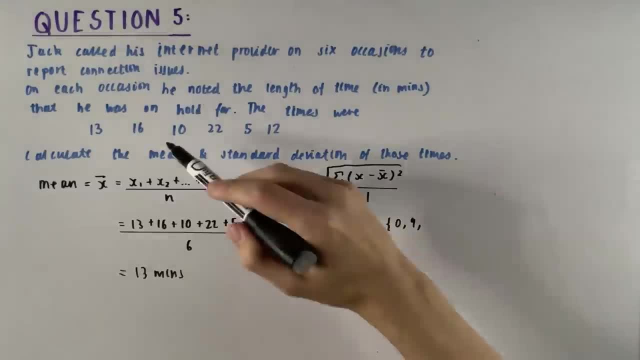 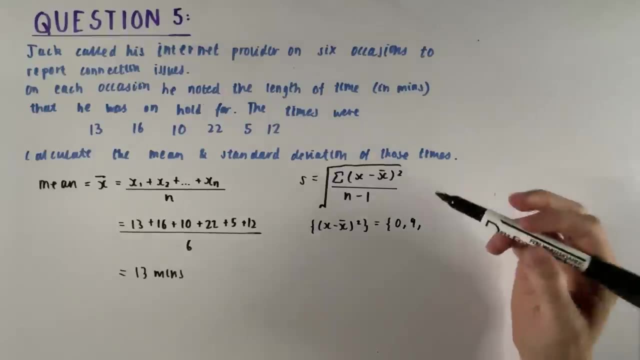 Squared is 9.. For 10. we've got 10 minus 3.. uh, 10 minus 13,. sorry, is minus 3.. Minus 3, squared is also .9.. Uh, 22 minus 13.. 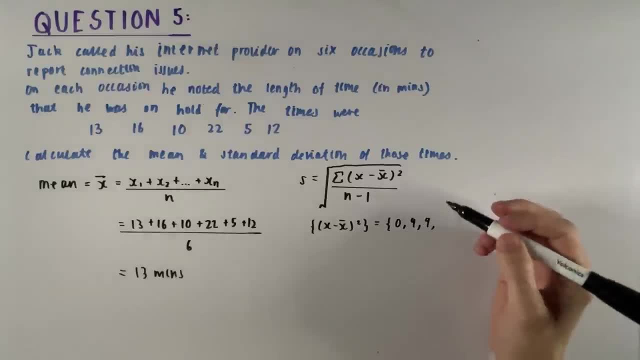 is going to give us 9.. 9 squared is 81.. 5 minus 13.. is going to give us minus 8.. Minus 8, squared is 64.. And then 12 minus 13.. 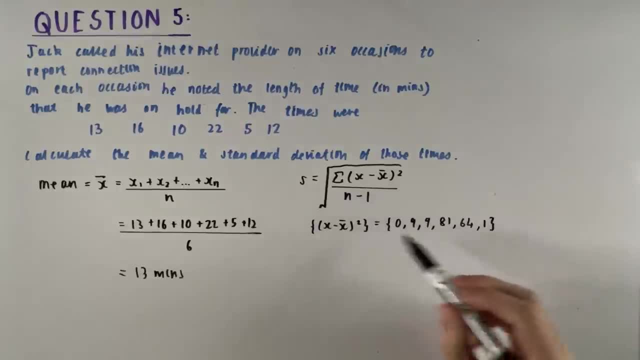 is minus 1.. Minus 1, squared is just 1.. So that is all these values in here. So now we can just substitute this into our equation. So we want to do the sum of all these numbers. So let's try and do this in our head. 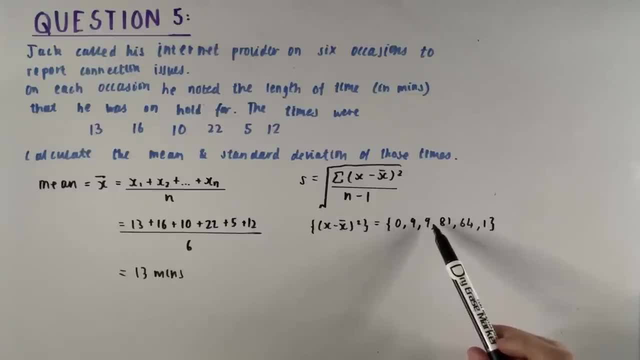 This is going to be. we can say 90.. .100.. .164.. divided by, and then n minus 1.. is 6 minus 1,, which is 5.. And then we want to do the square root of this. 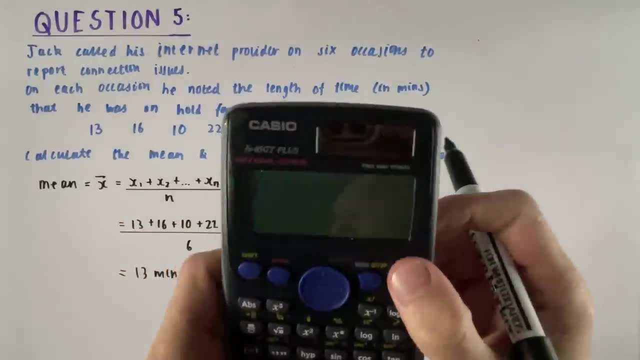 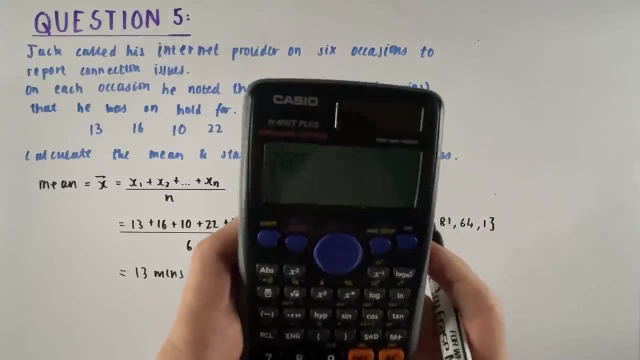 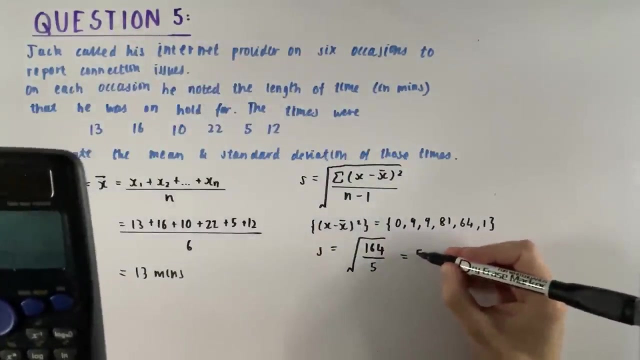 Now I'm actually going to need to put this into a calculator, So let's do the square root of 164.. divided by 5. We get this decimal number, which we'll just round to 5.7.. 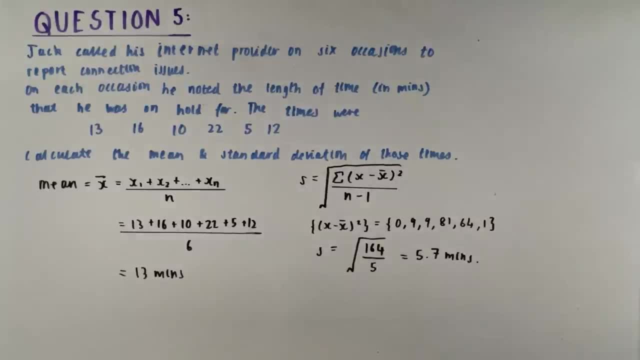 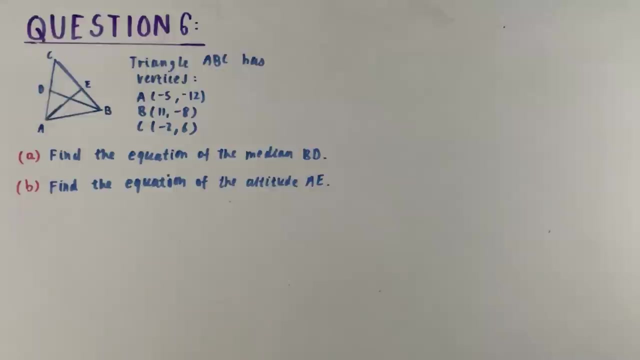 Make sure we write mins And that is our standard deviation and our mean for Jack's times that he was on hold for Alrighty. Going on to question 6.. Looks like we're doing a bit of. 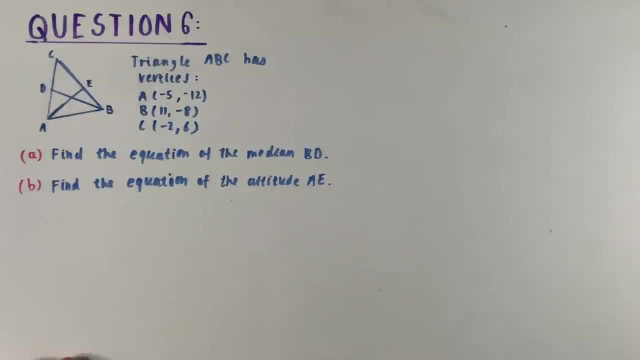 geometry in this question, Um and algebra actually. So we have got this very burly drawn diagram- I apologize- of triangle ABC And we're told that it has vertices as follows: 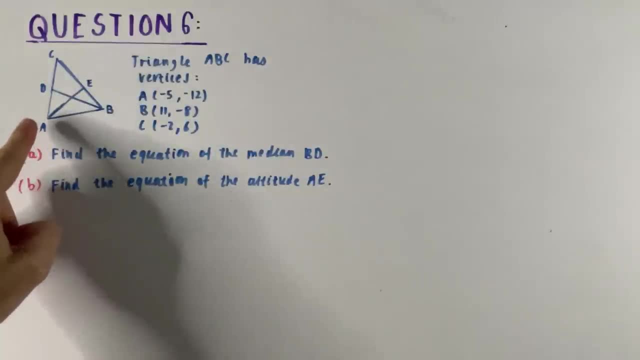 A is the point minus 5. minus 12.. B is the point .11. minus 8., And C as the point minus 3. .6.. Obviously, this is not a scale. Part A. 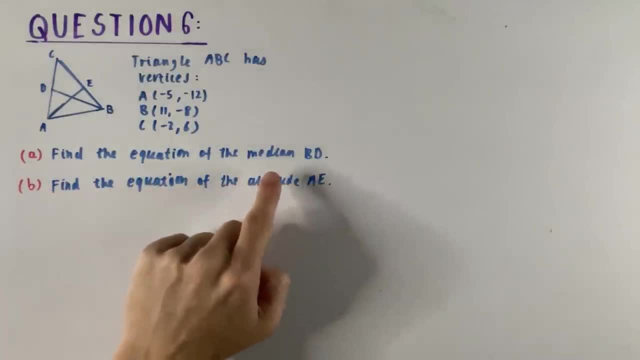 We are asked to find the equation of the median, BD, This line here It's important that it tells us it's the median. And we are also asked to find the equation of the altitude- Altitude again. 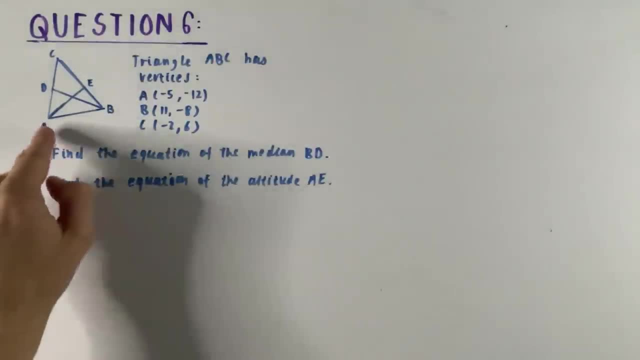 It's very important. We know it's the altitude AE, So let's tackle both parts of this equation, of this question, Alrighty. So for the first part, we're asked to find the equation. 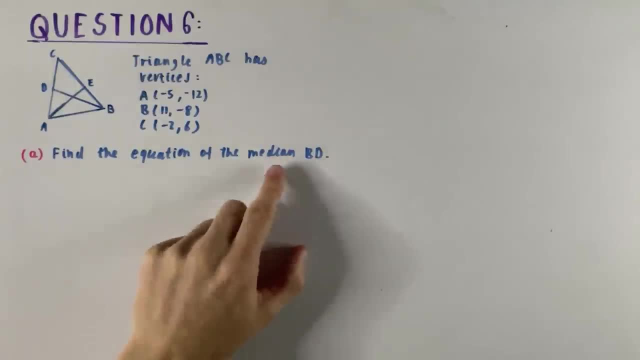 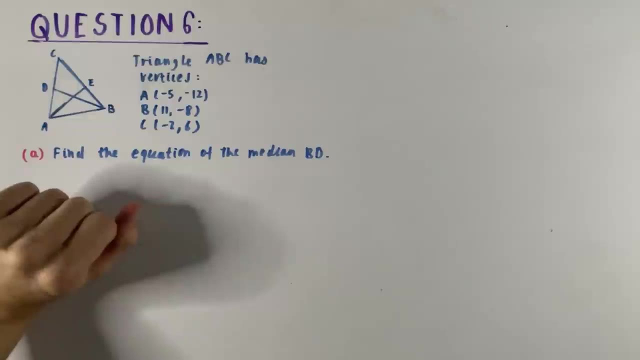 of the median, BD. Now, what does median mean? Well, it means that this line here, BD, intersects the middle, the midpoint of another line. Now, clearly, it's not this line BC. 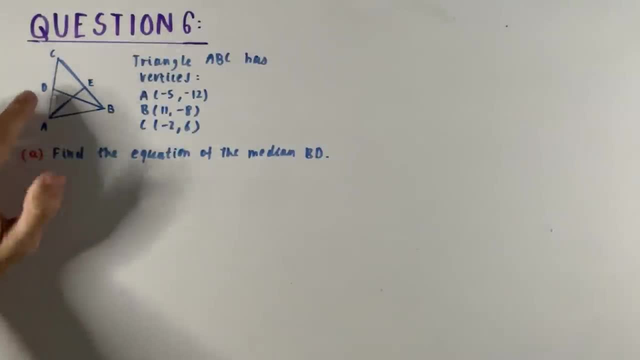 because that's the end of the line. So it's this point here, D, that intersects the middle of the line AC. So before we work out the gradient and then the equation of the line we need to work out. 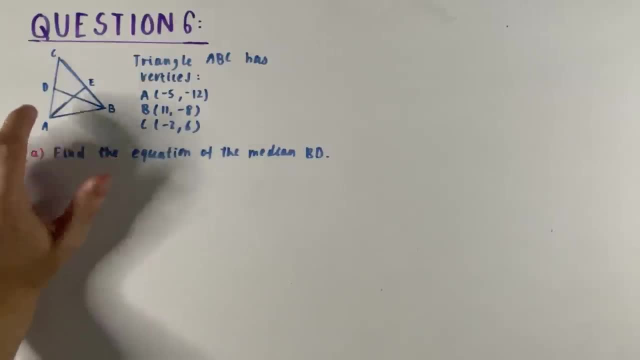 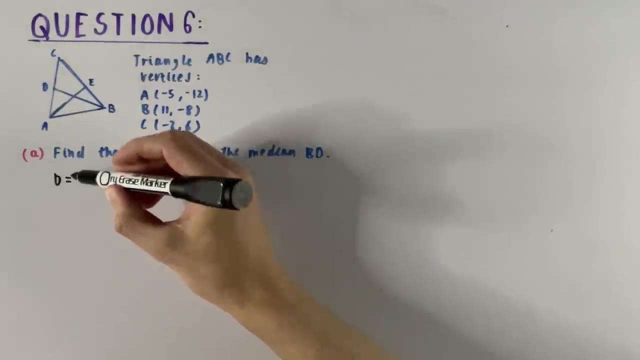 this point D. So we know it's the midpoint of AC. So let's write that D equals the midpoint of AC. Now what is the midpoint? It's the middle of A and C. 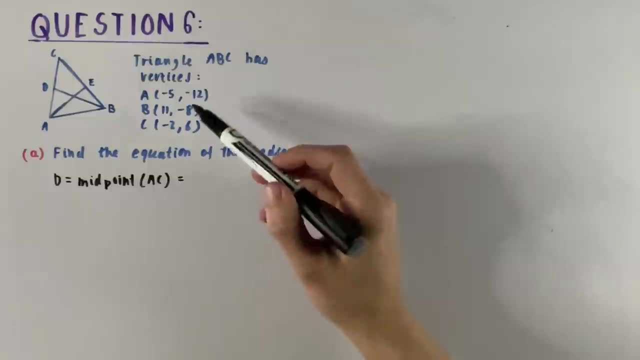 So we can work out what the middle of that line is, because we have the coordinates of A and C. Now the equation for a midpoint is the first x value, So in our case it will be 5.. 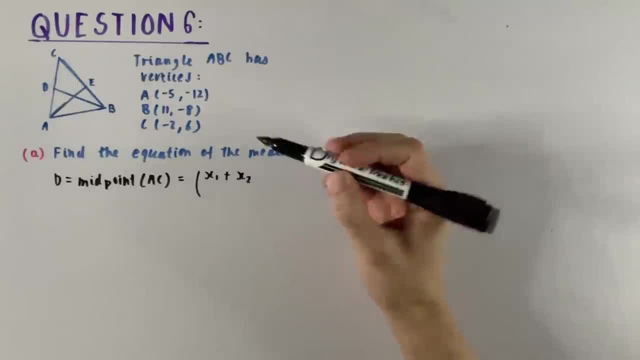 plus the second x value, In our case it will be minus 3.. And it's the middle of this, So it's the average kind of You. divide it by 2.. Heck, let's not use a ruler. 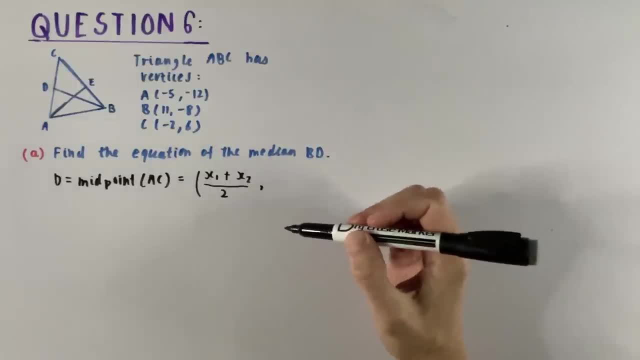 It's a tiny equation, Tiny fraction, Sorry if it bothers you. And the second point is similar. It's just the middle of the y values. Just trying to do a better straight line here, There we go. So this is our equation of the midpoint. 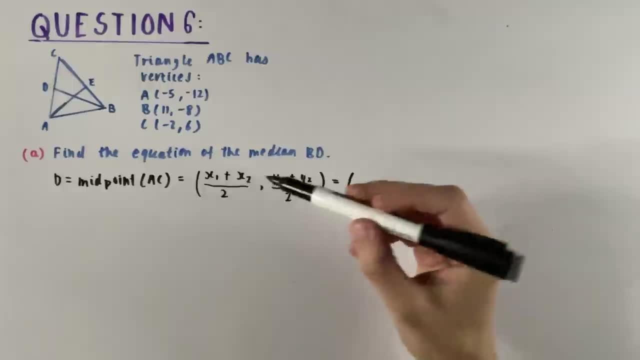 So let's substitute our values in, So the first coordinate is going to be minus 5.. and then plus minus 3.. Let's just simplify that to minus 3.. Divide it by 2.. And the second coordinate is: 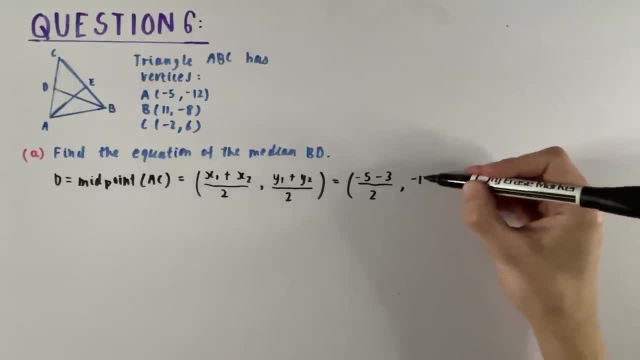 or the second point is going to be minus 12.. which is our y1. And our y2 is 6. So plus 6. And then we're dividing that by 2.. So we have just evaluated. 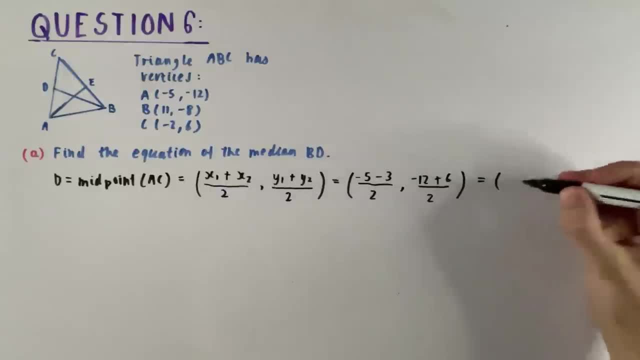 that the point D is the point Well, that's going to be minus 8.. divided by 2 is minus 4.. This is going to be minus 6 divided by 2., which is minus 3.. 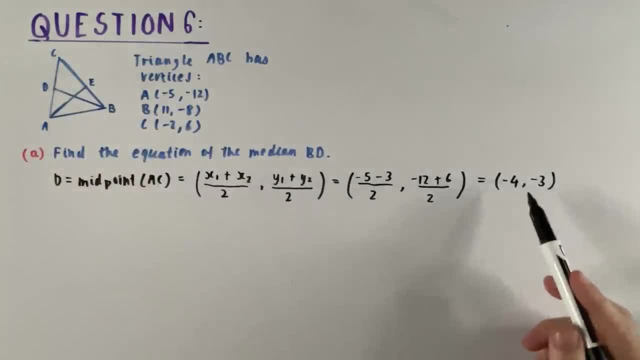 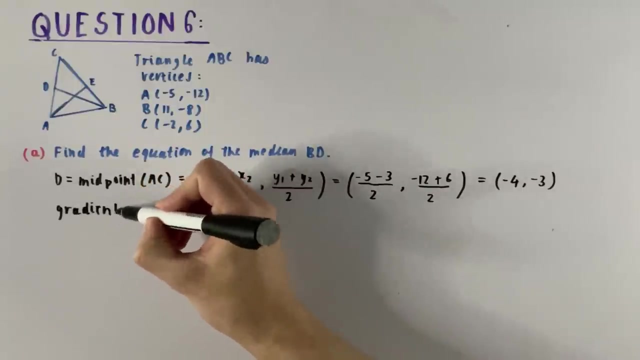 And that seems to be about right. So that's our coordinate of D. So now that we have the points B and D, we can work out the gradient, the gradient gradient of the line BD. 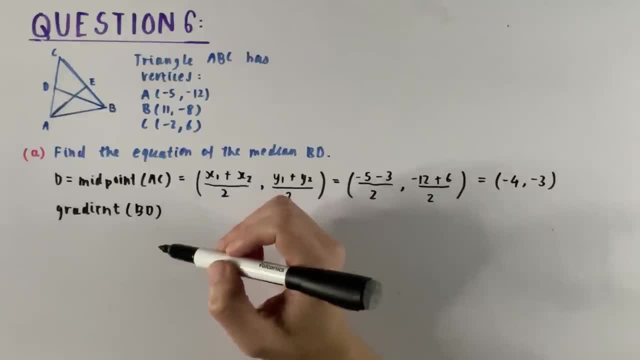 So let us do that. Let's do that. Now the gradient. we've got this equation here: y2, take y1.. divided by x2, take away x1.. the difference of the y. 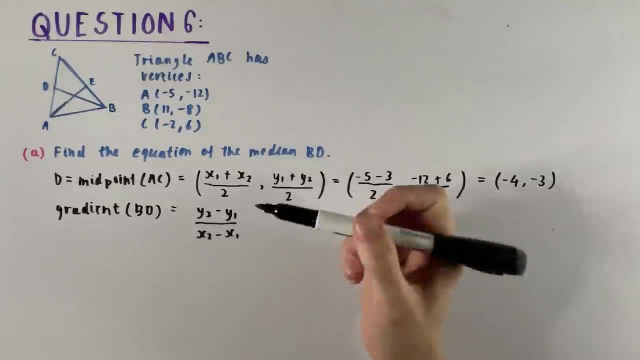 over the difference of the x. As we know, that's what a gradient is. It's the slope, the steepness of the line. So let's plug these values in Now. in our case, we can let y and x be. 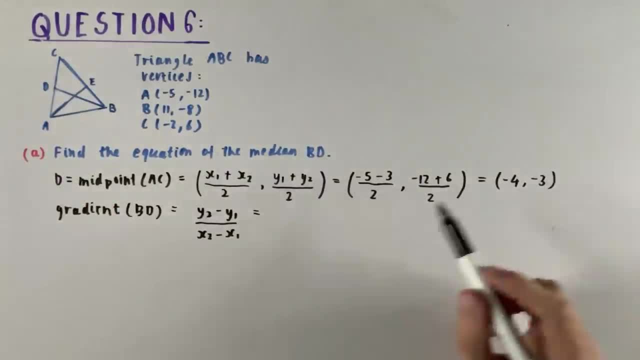 any of the way-arounds of B and D. What I mean is our y2.. can be either this coordinate here, this point minus 3. or it could be minus 8.. 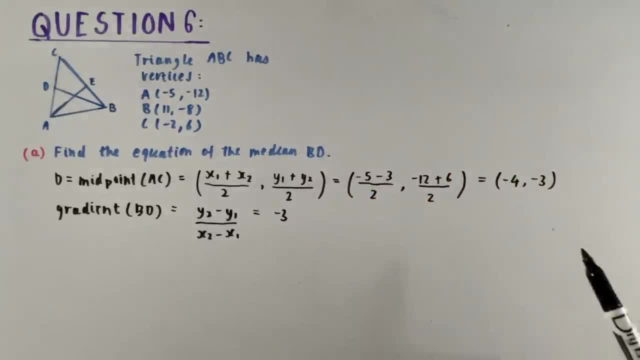 Let's just go with minus 3, though Now we are subtracting minus 8. which is the same as adding 8. And now that we've done it that way around, we need to stay consistent. 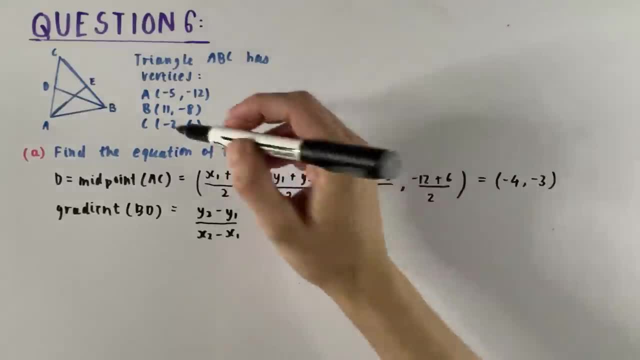 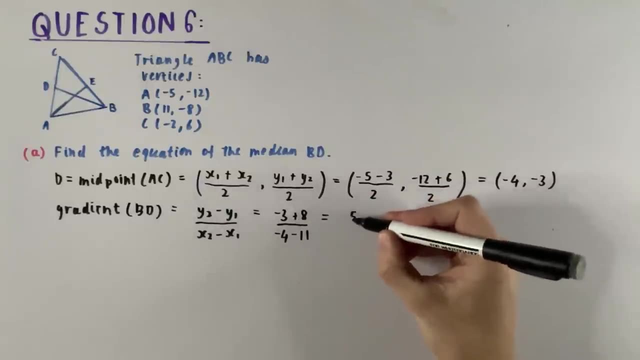 So we need to let x2 be minus 4. and x1 be 11. So minus 11.. Like so. So this is going to give us .5. over minus 15., Which we can simplify. 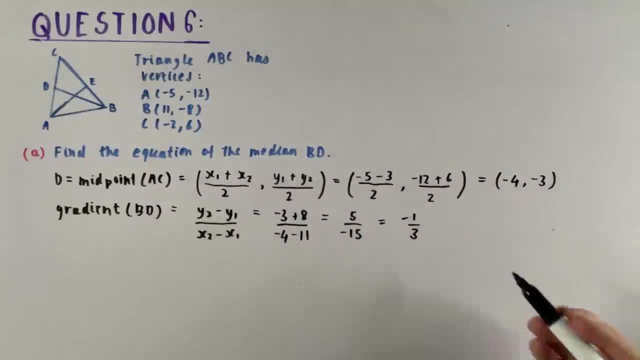 to just be minus a third. So that's our gradient of the line BD. Now that we have the gradient of the line BD and we've got two points, we can actually find the equation. 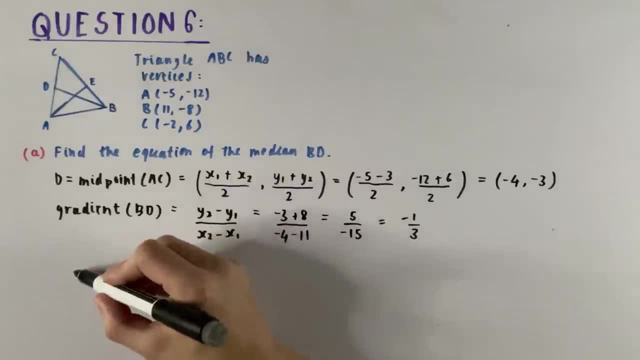 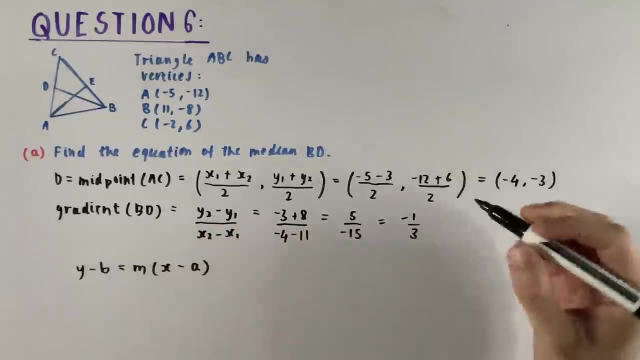 So we know when solving the equation, we can use this equation here. Let's just say that that's equal to M, because that's the symbol for gradient. Make it consistent down here. 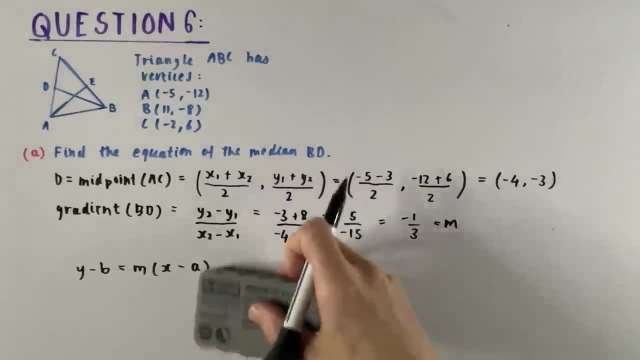 So this is our equation of a line, So we'll sub in our values. Now our a and our b are the x and y coordinate of either B or D. Let's just 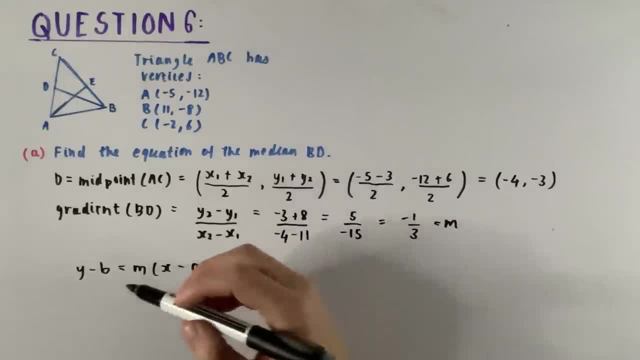 go with D, So we can say that this here is equal to y. Now our b is minus 3.. So plus 3.. Our m is minus a third x and then a is minus 4.. 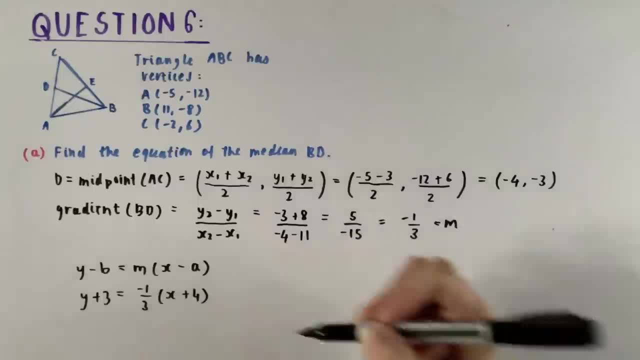 So minus minus 4.. Plus 4 is plus 4. And we can simplify this by actually multiplying everything by 3. Because this will just get rid of this fraction here. So we get. 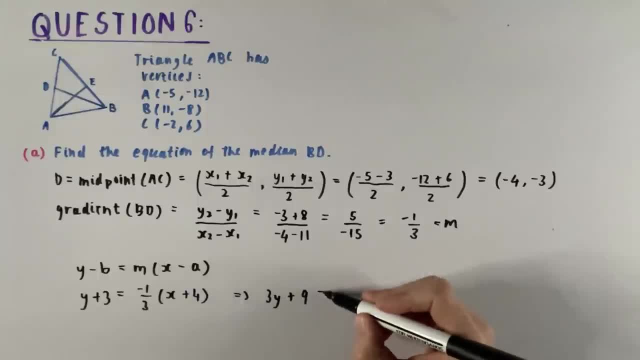 .3y plus 9. is equal to minus 1.. x plus 4. And we'll just write that out again as .3y plus 9. is equal to minus x. 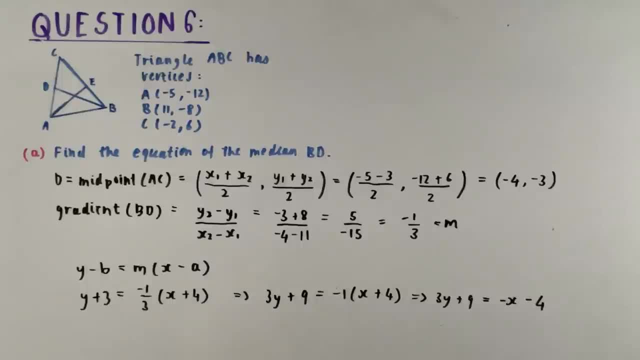 minus 4.. And then we can rearrange this: The 3y is gonna equal minus x, um minus .13.. That doesn't seem right. Oh no, That doesn't seem right yet. 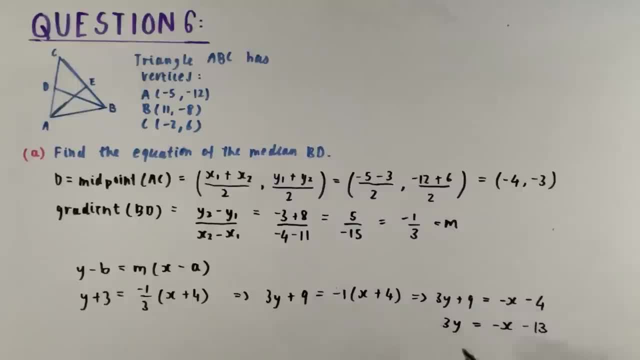 That's the equation of the line. Now it's okay to leave it like this. We don't need to rearrange. That should be okay Now. in fact, if I were a teacher, I would have just accepted this. 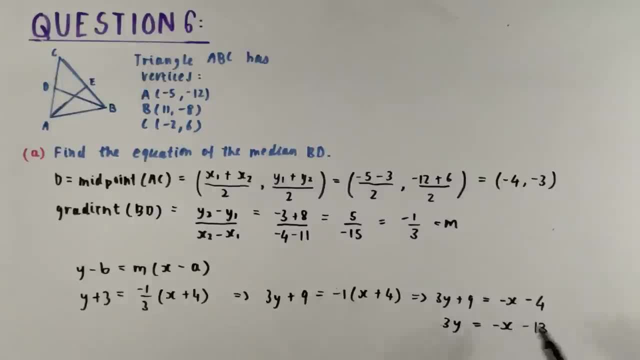 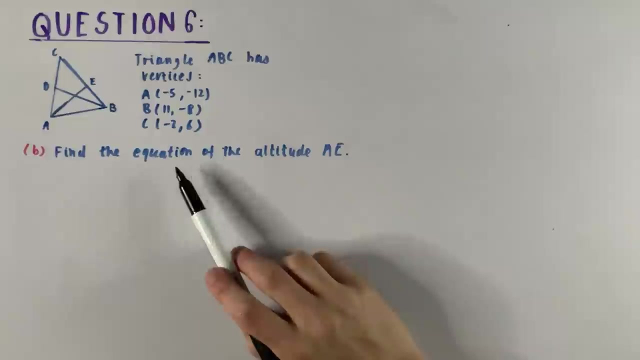 as the answer here, but it's probably best to get it in this form down here. So that's part A, Swiftly moving on to part B. We were asked to find the equation. 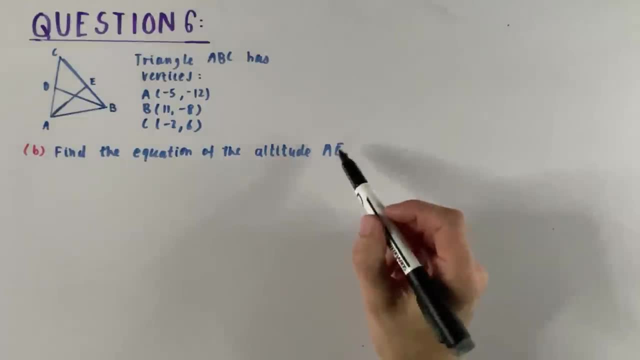 of the altitude AE. It's a bit of a badly written E, but this line here, A to E Now, because we're told it is the altitude, we know that the altitude. 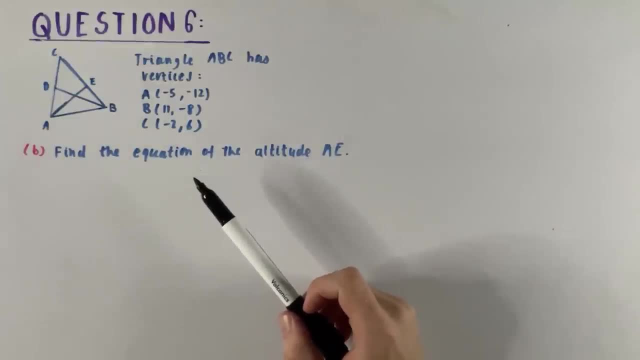 is perpendicular, perpendicular, perpendicular to another line. Now we know it's not AC because, well, they don't look perpendicular, and we know it's not AB because they definitely don't. 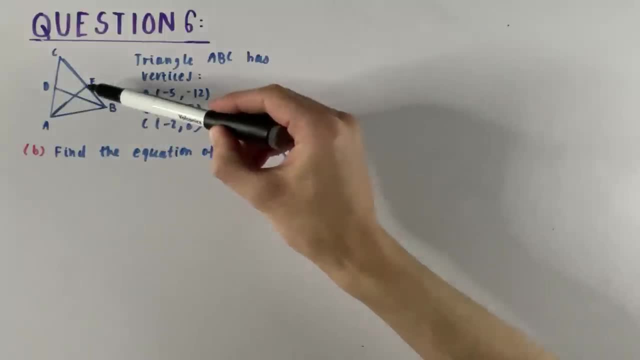 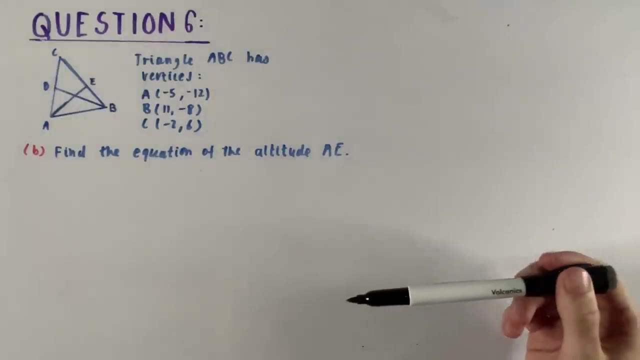 look perpendicular, So the altitude AE must be perpendicular to BC. So why do we need to know this? Well, perpendicular lines have opposite gradients. Um, what I mean is, whatever the gradient of BC. 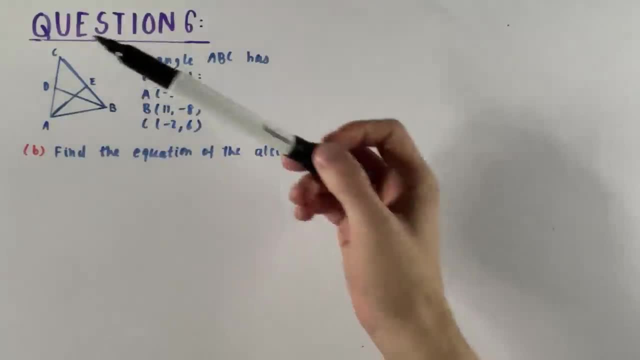 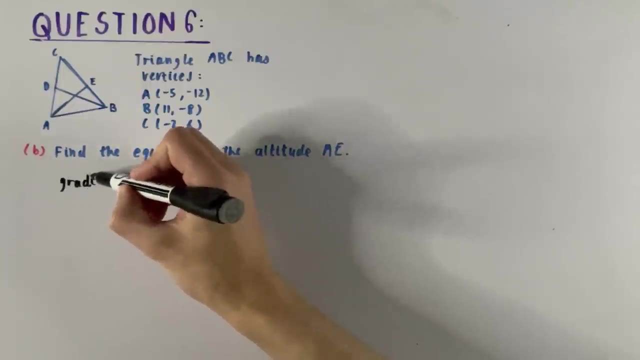 is, we can work out the gradient of AE By doing so. So let's see the gradient. We need to work out the gradient of BC first, So the gradient of BC, we'll just do our formula. 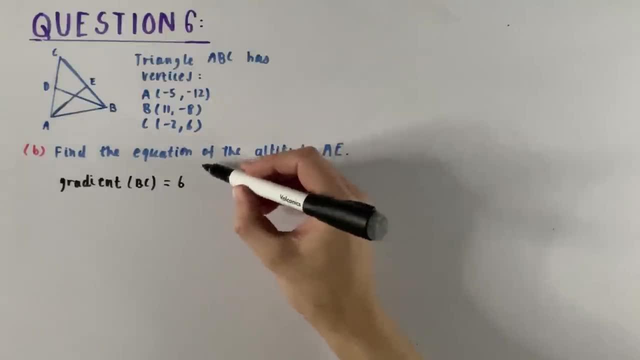 from the question before. so we're gonna have six minus minus eight, which is just plus eight divided by minus three minus eleven, I believe, And, um, yeah, that's gonna give us. 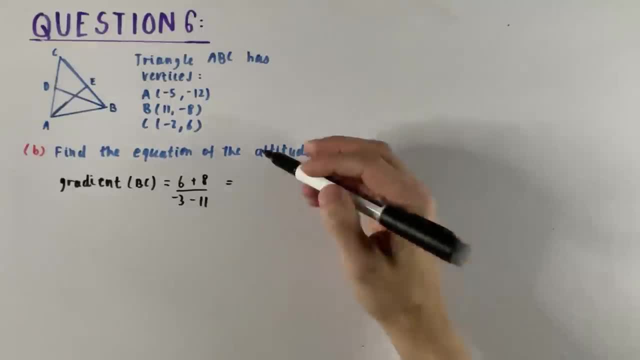 um, we're gonna have fourteen over minus fourteen, which is actually just negative one. Now, because we know this, we can say: therefore: that little symbol there just means: therefore: 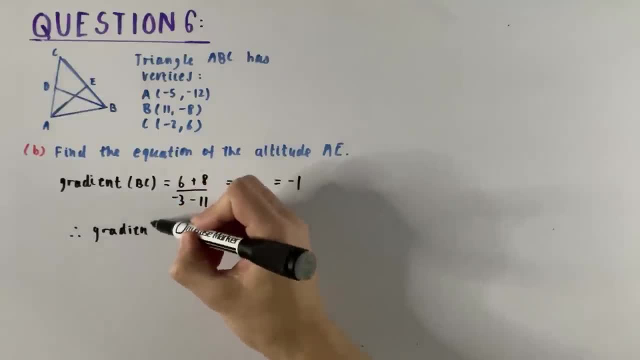 the gradient of AE is equal to one, Because it's the opposite of minus one. the formula basically is: you multiply this by another number to give one, So multiply by some unknown. 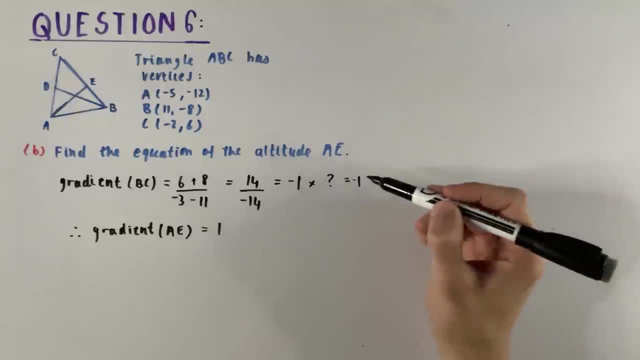 to give one. It's obviously uh minus one, sorry, It's obviously going to be one. So now that we have the gradient of the altitude AE, we can do just what we did in the first part using the formula. 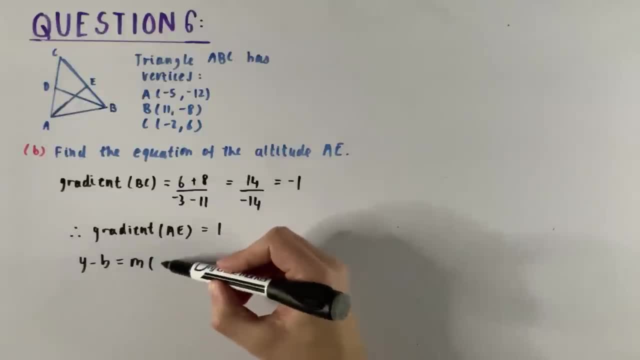 y. take b equals m x. take a Again. let's say that this here one is our gradient, So we can sub in our values. so we're just gonna have y. Now again our a and b. 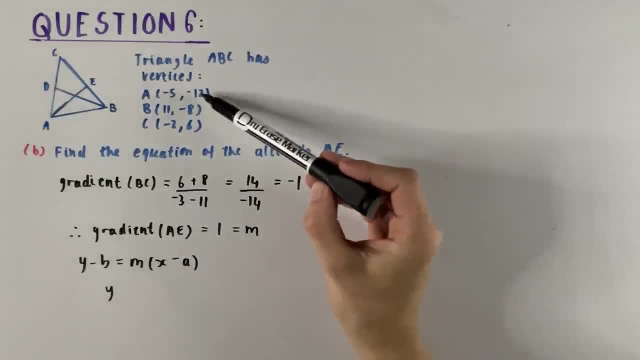 are the x and y coordinates of either point A or E. Now we don't know point E, so we have to use point A. So it's gonna be y, take b, uh, ace or the second part. 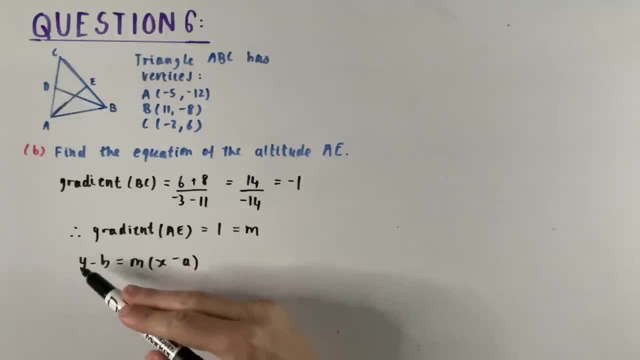 So y take away twelve is uh y sorry, y subtract minus twelve. So y plus twelve is equal to one. We'll just drop that, though, And we're gonna have x subtract minus five, so x plus five. 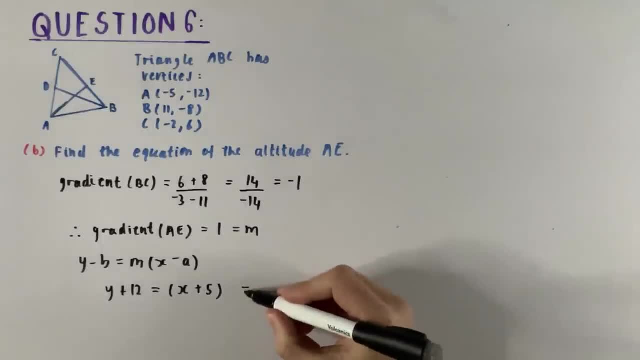 Now again, I would just accept that, but it's probably best to rearrange that and just say: y is equal to x subtract seven, And that is our equation of the altitude AE. 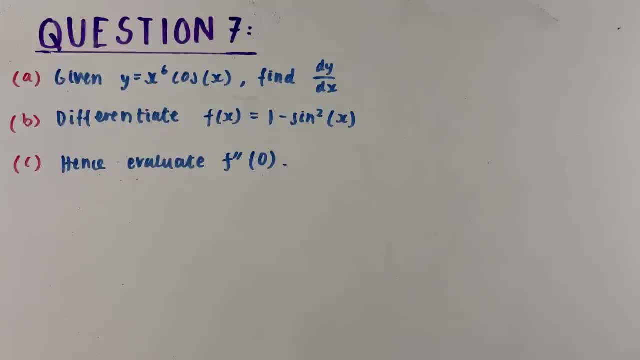 Question number seven, My favourite, A nice question about differentiation, Differentiation, Differentiation. And we've actually got not two but three parts to this question. So the first part says: 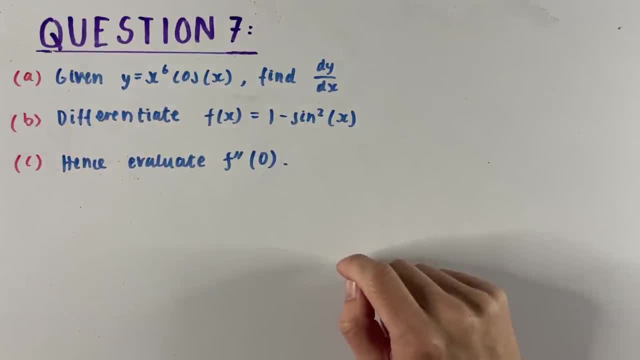 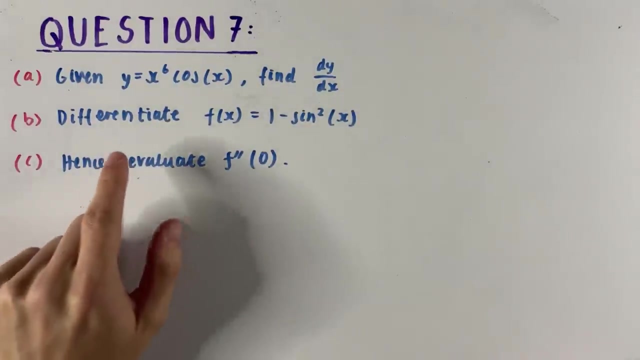 given the equation: y equals x to the power of six. multiply by cos x, find the derivative, derivative dy by dx. part b says to differentiate the function in terms of x. 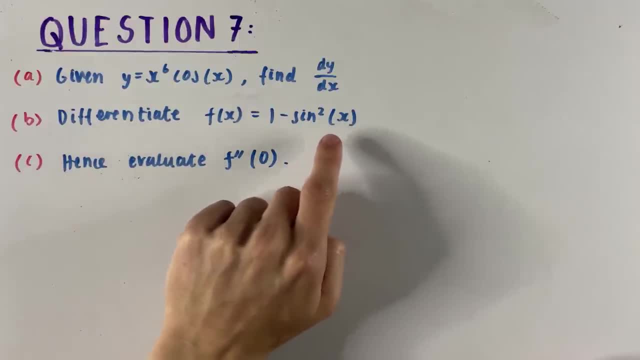 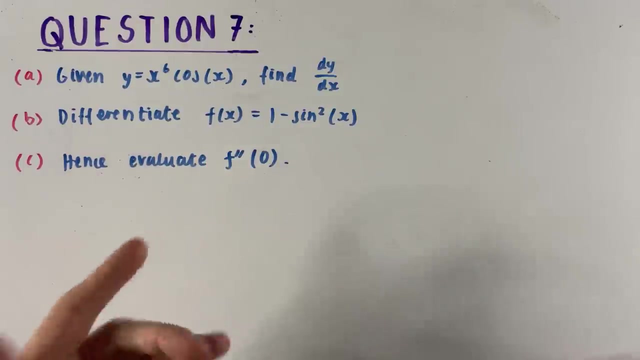 one minus sine squared x, and part c says: hence evaluate the higher derivative, the second derivative of the function of x, at the point zero or at the 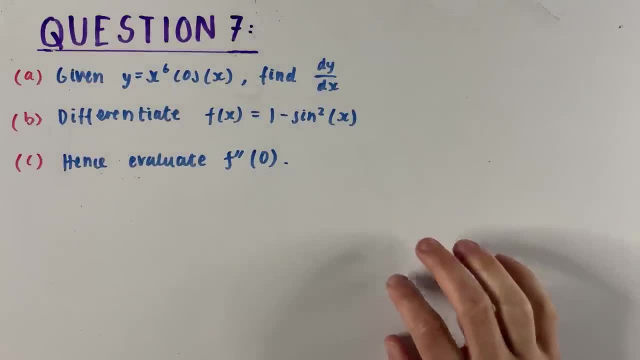 value zero. so we can't do part c without doing part b. but obviously we'll begin with part a, So part a. we have this equation: y equals x to the six. 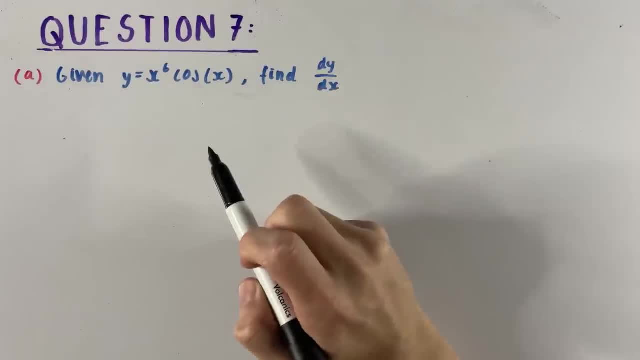 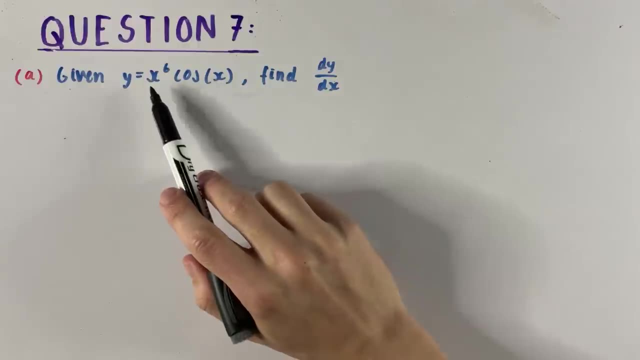 cos x and we're asked to find dy by dx. Now, because we have two functions in terms of x, we've got x to the six and cos x multiply by each other, we have to. 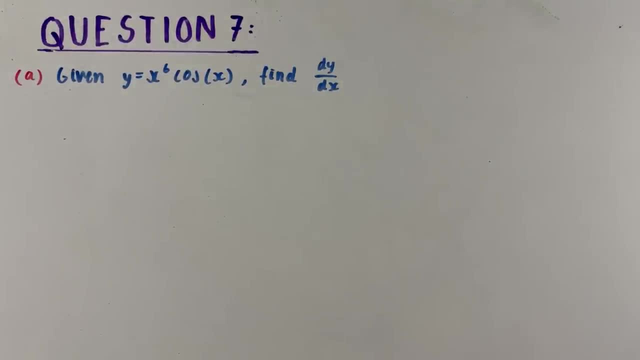 do a rule called the product rule. Now again, kind of like the other questions, I'm gonna tell you what that is, but I'll assume that some of you out there will know what that is. So 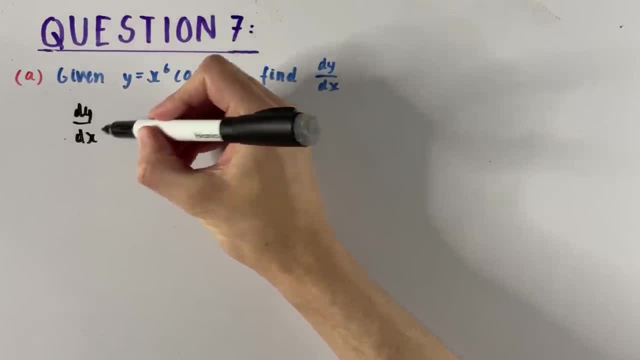 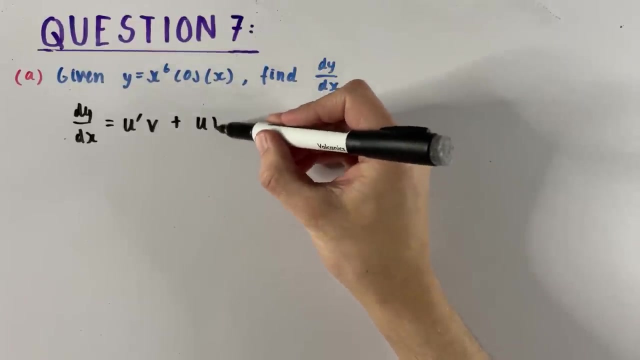 the product rule states that the derivative dy by dx is equal to some function. u derived, multiplied by v plus u. just standard. u multiplied by the derivative of v. 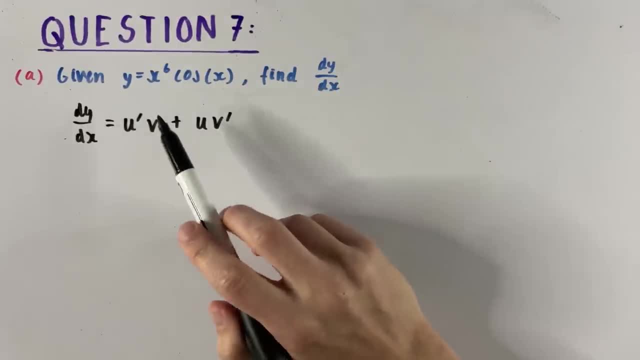 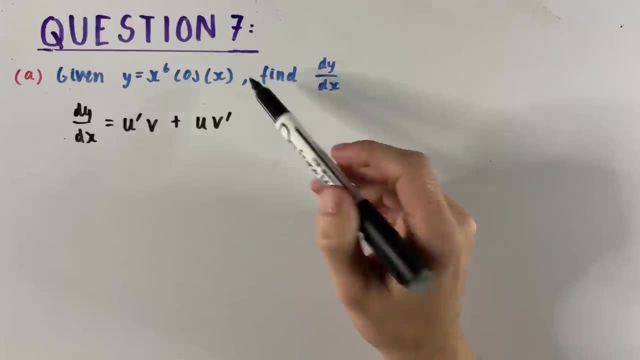 Now, what this means is we need to let one of these bits be u and one of these bits be v, Calculate the derivatives of them and then sub them into this equation. 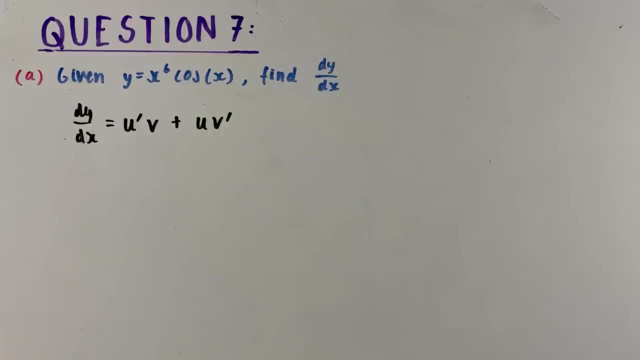 So to do that, I have this second pen here. I've got this light blue one, so let's out to the side here evaluate what u and v are going to be So 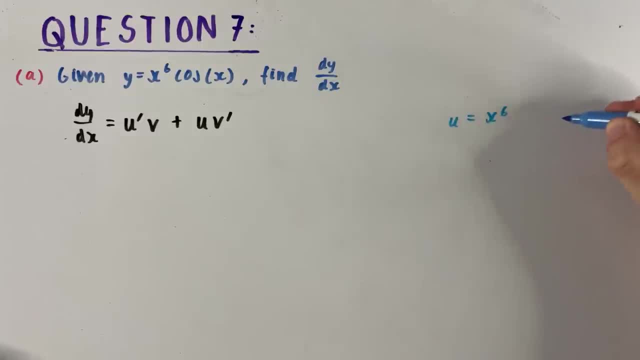 let u be x to the sixth and v can be our cos x. Now the derivative u dash. that just means du by dx, so we can derive that to be 6x to the power 5.. 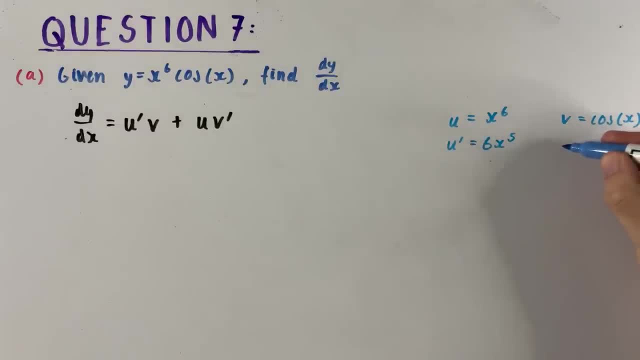 bring the power down to the front. subtract 1.. now v. we've got cos x, we've got a trigonometric function and the derivative of cos x is minus sine x. 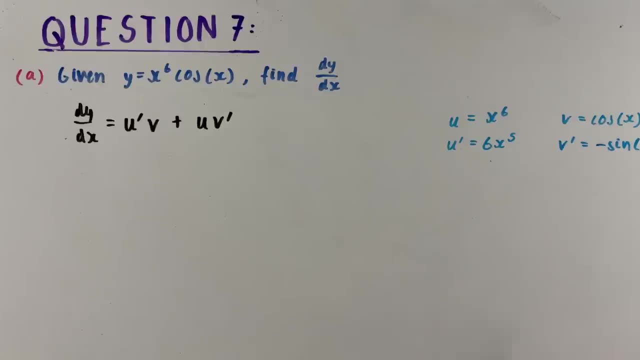 like so, And now that we've got this, we can sub them back into our equations. So let's sub them in. So first we do u dash times v, so it's going to be 6.. 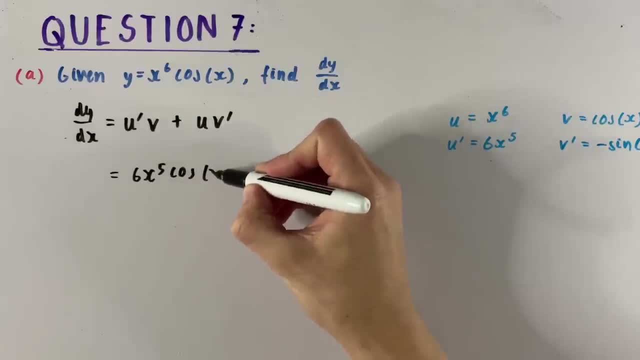 x to the 5. cos x plus, and then we're just cross multiplying those two plus those two. so actually this is going to be minus, because we've got minus sine x. 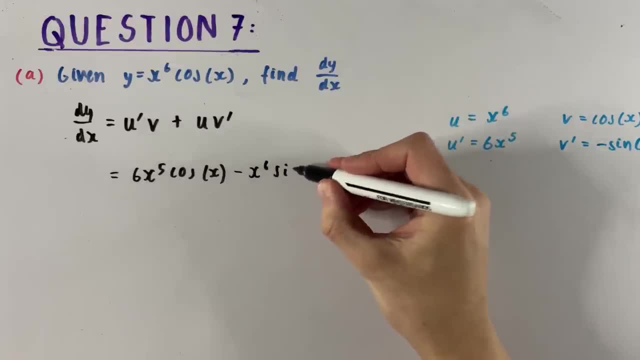 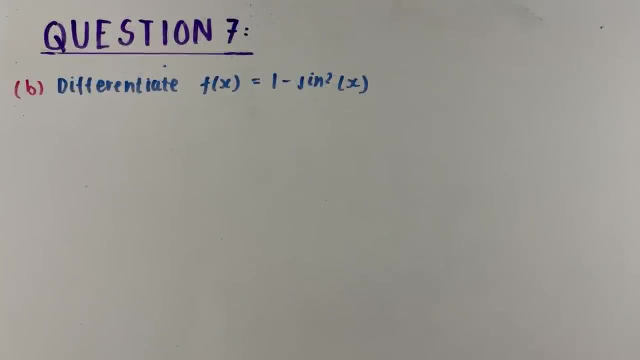 so it's going to be minus x to the 6. sine x. and that is that for part a. Part b asks us to differentiate: the function f of x equals 1.. 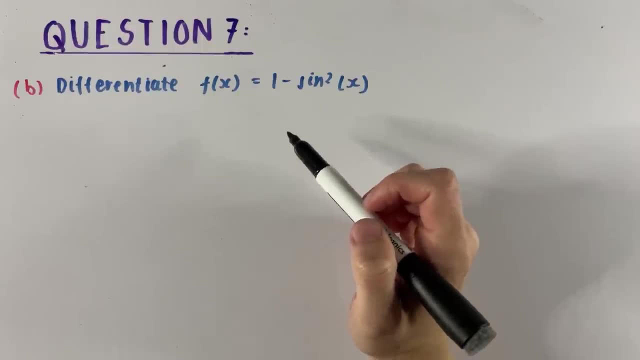 minus sine squared x. Now we could solve this through by differentiating .1 and then differentiating minus sine squared x. or or, or, or. we can use the fact that: 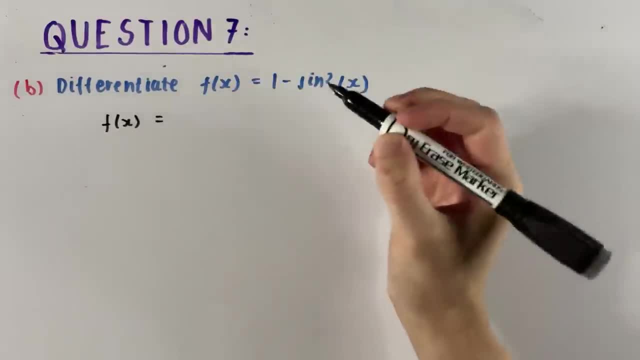 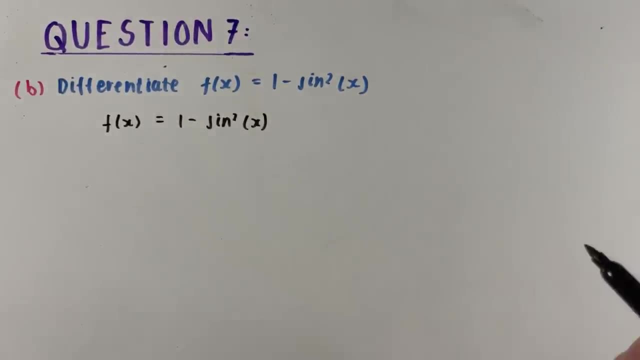 f of x, which equals .1 minus sine squared x. we can use one of our trigonometric identities, which is the identity that sine squared x plus cos squared x. 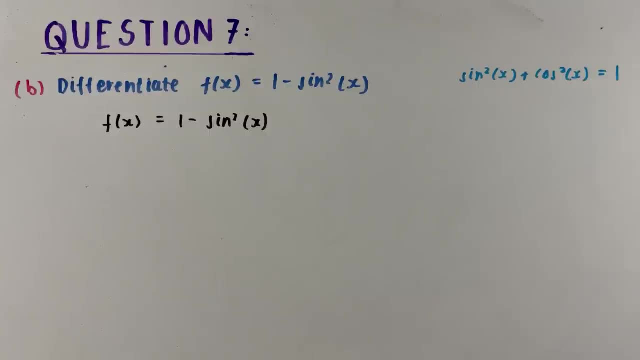 is equal to 1.. Now we can rearrange this to get: cos squared x equals 1. subtract sine squared x, which is what we have here, So we can say that this is the same as cos. 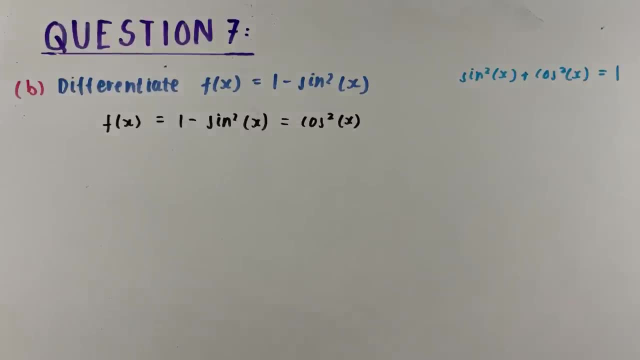 squared x, And now that makes it a little easier for us to differentiate, So we can differentiate f dashed x to give us. now we have to do a bit of chain rule here actually. 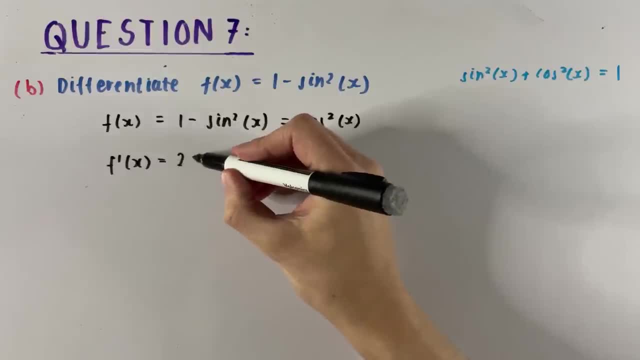 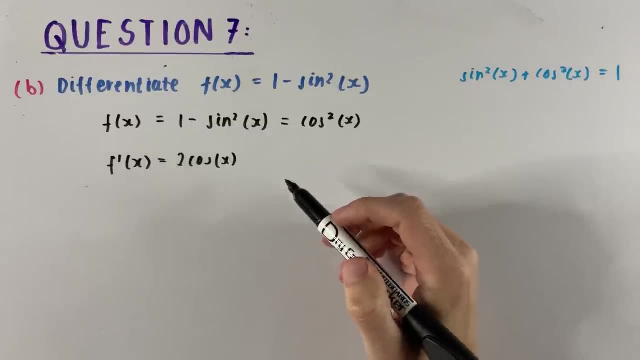 We begin by bringing the power down to the front, So we get 2.. cos squared x and we take away 1 from the power, so it's just cos squared x. Now we have to do chain rule. 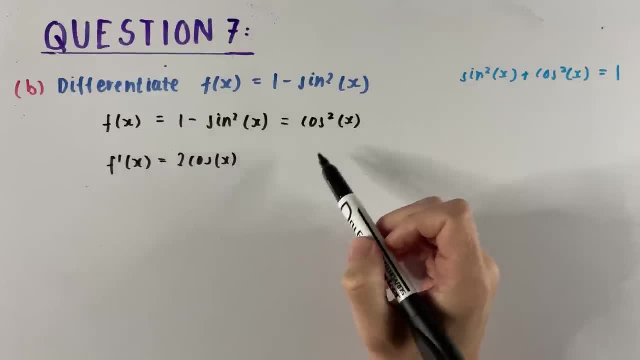 so we also have to multiply by the derivative of cos squared x, which is minus sine squared x, And this is actually another um metric identity. Wow, This question has a lot of um. 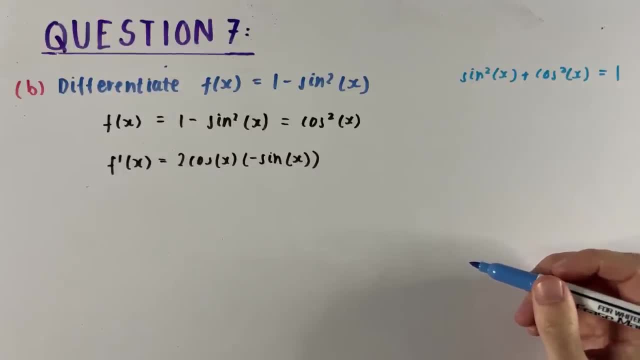 using your trig knowledge. So this question here has the identity that? um well, the original identity is that do sine x, cos x is equal to sine. 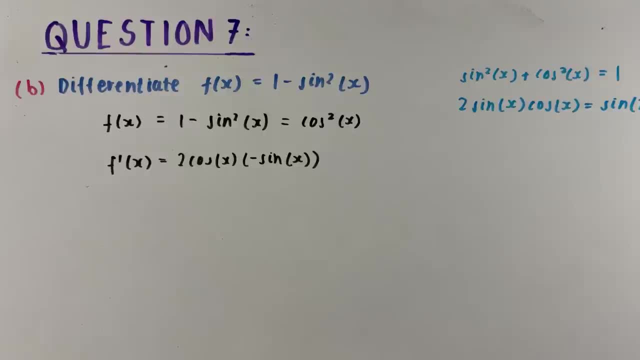 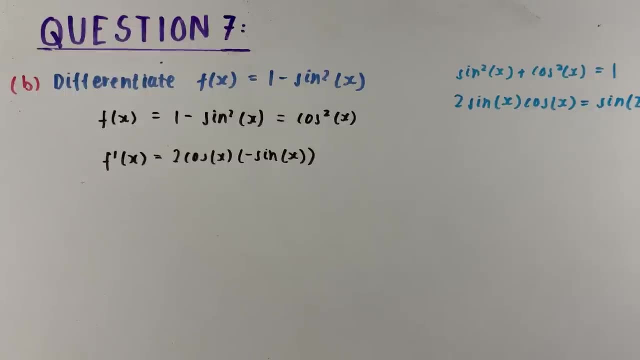 two x. That's the original um identity. It's kind of going off the screen there, my bad, Let me. let me write this underneath: It's equal to sine two x. 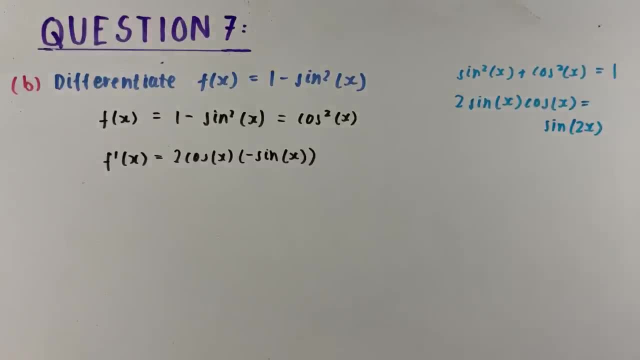 That's just a generic identity that we're taught. However, r's looks like this: Minus two, sine x, cos x, Which is quite similar to this, except with the minus at the start. 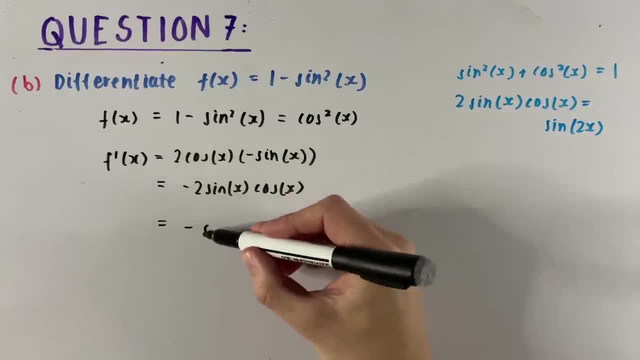 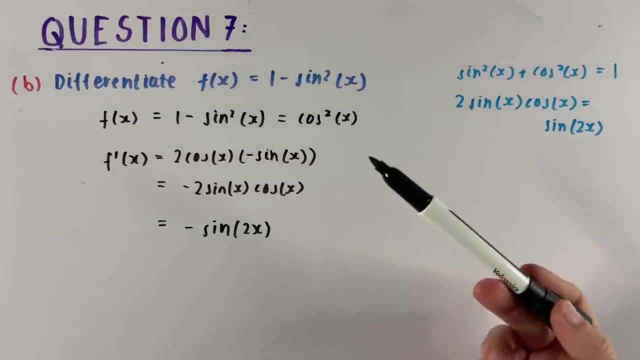 So we can just say that that is the minus sine two x. So we can use our trig identities in this question to get um this final answer here, which is minus sine two x. 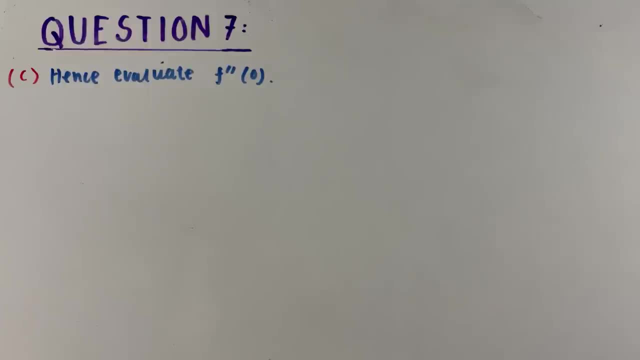 For part c. It says: hence evaluate the second derivative of the function at zero, Where x is zero in our case. Now we need to be really careful that we don't 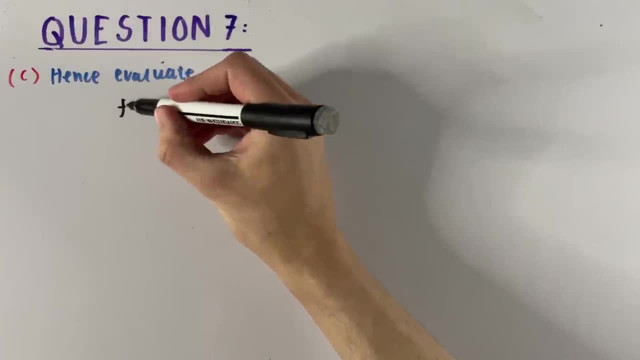 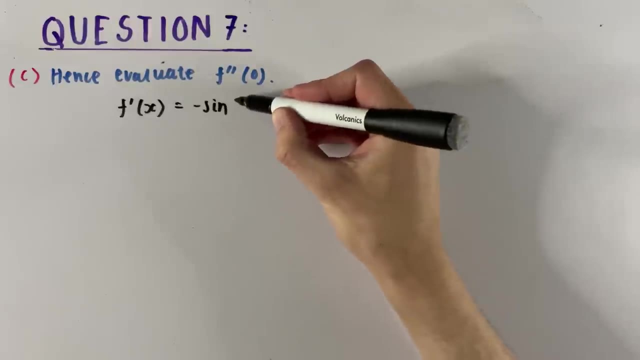 substitute our zero into our f dashed of x, which we said from the question before was minus sine two x. We need to be careful that we don't substitute zero. 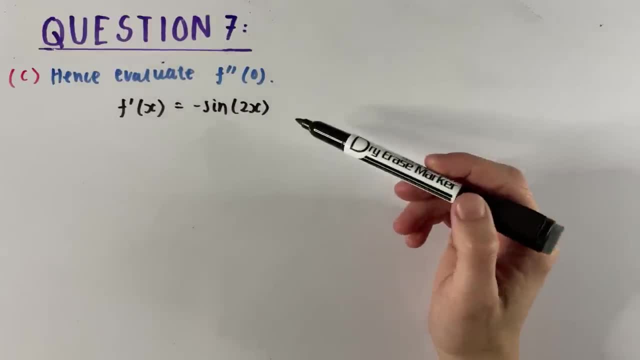 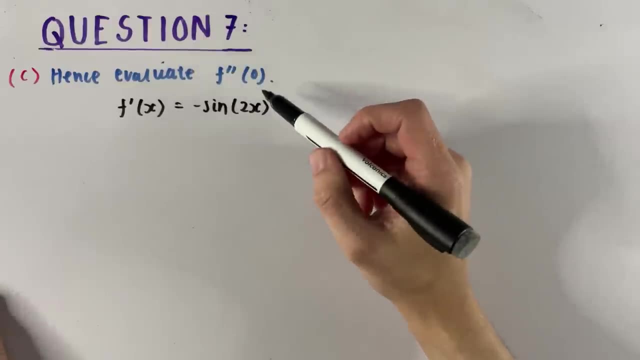 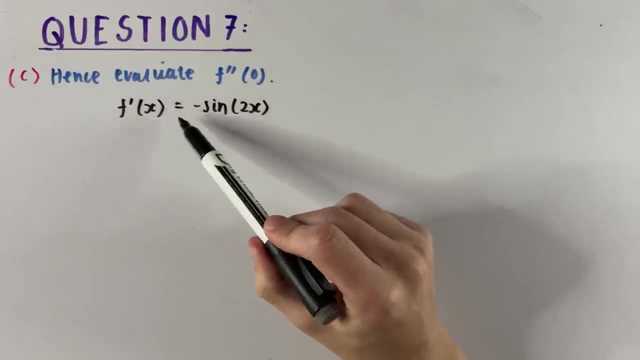 into that, Which would actually just give us zero. That would be the wrong answer, Because we have this second dash here. We now need to work out the derivative of this function here, This f dashed of x. 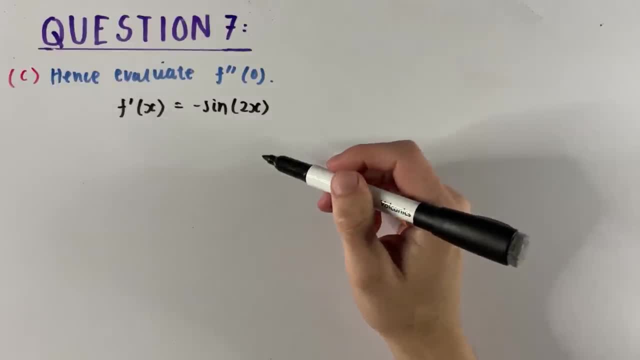 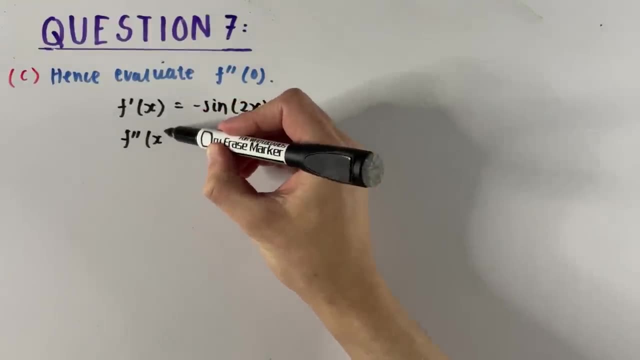 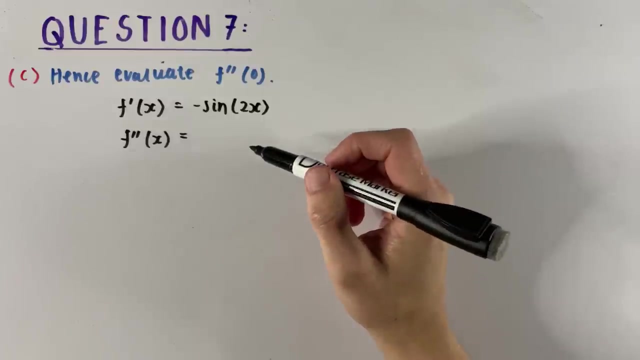 The second derivative of our original function. So let's do that first. So the second derivative is the derivative of minus sine two x. So let's work that out, So we know that. 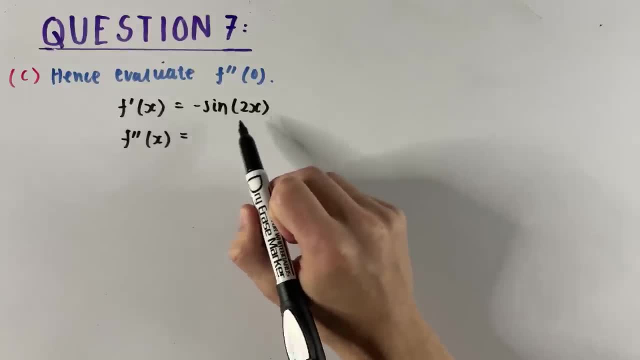 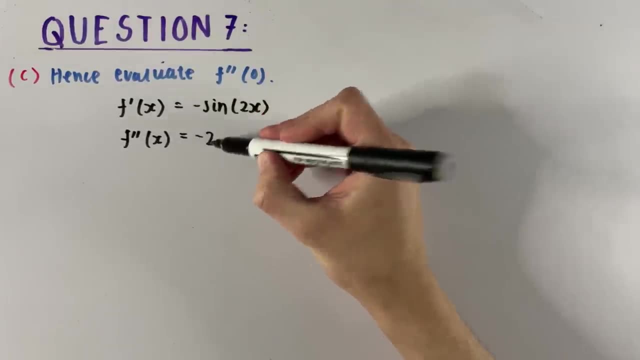 with sine two x, it's going to go to you. take this bit out here. If this is a, for example, you want to take a out to the front, So we get minus two cos. 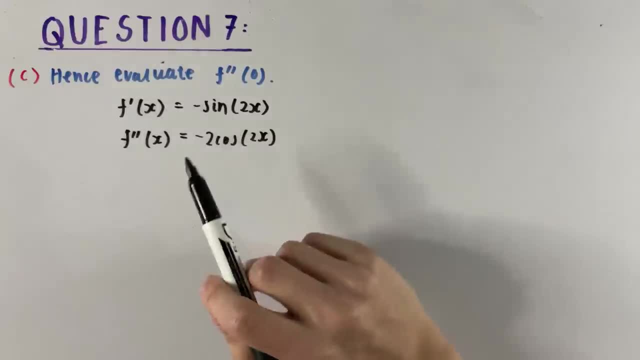 two x. That would be just the answer, So that's not too bad actually. However, we need to work out what f double dash of zero is, So to do this. anywhere we see an x. 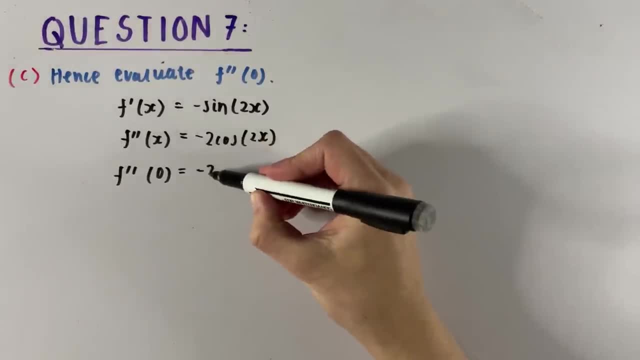 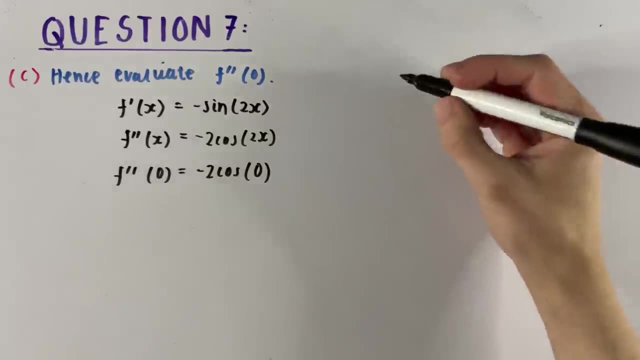 we sub in the value zero, So we've got minus two cos, and then two times zero is just zero. Now we are going to use the rule that cos of zero is equal to one, Which? 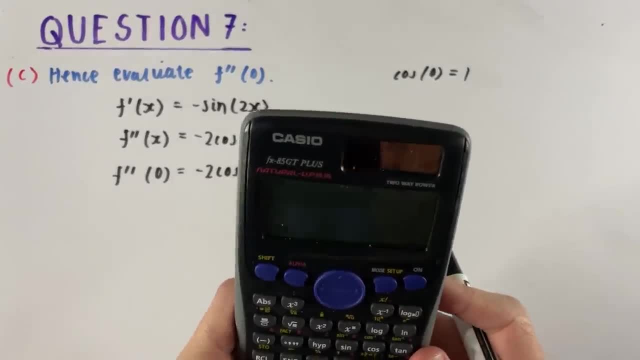 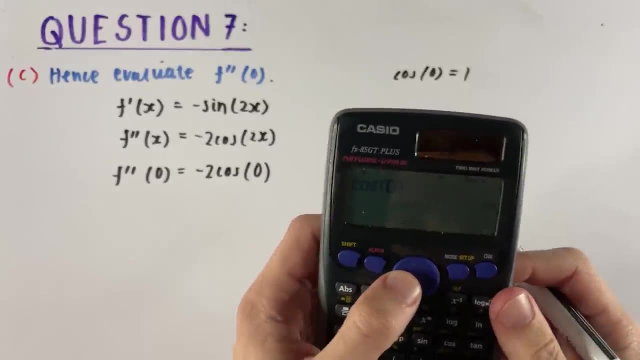 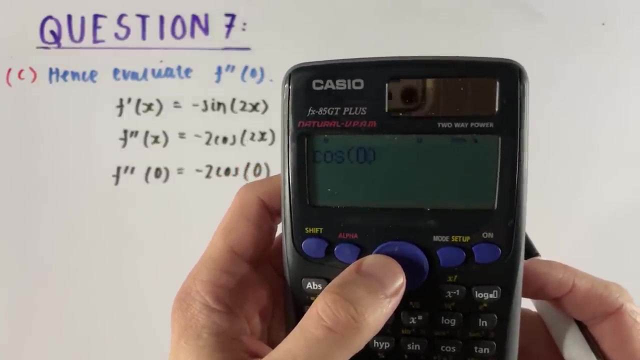 if you didn't know in an exam, you could just put into your calculator: um cos of zero is equal to one, And you could actually just stick the minus two in front. It's not letting me go to the front. 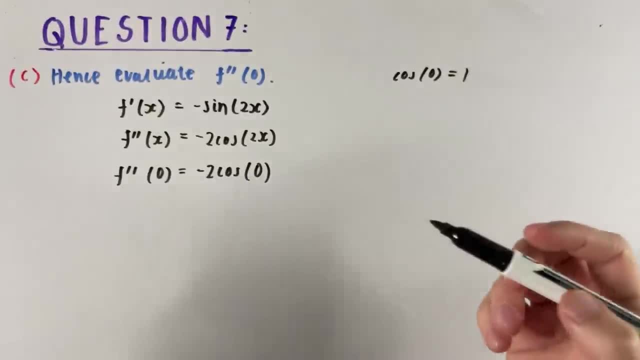 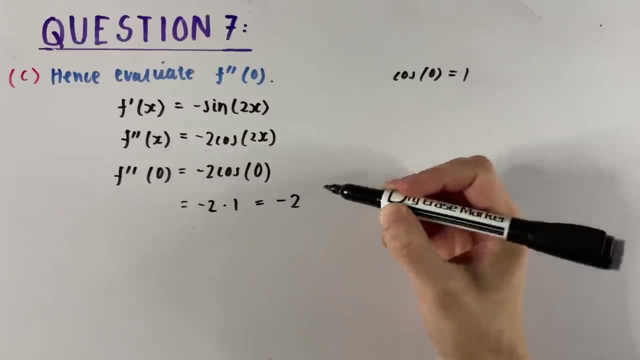 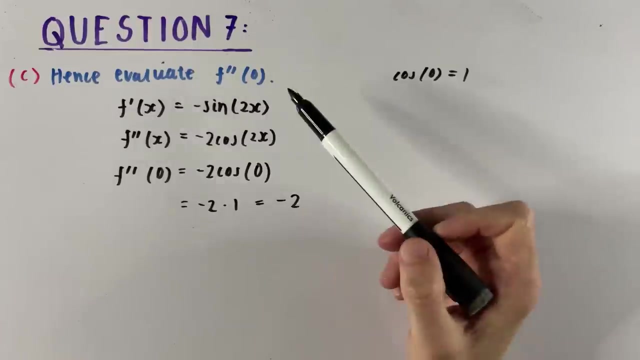 There we go. Minus two, cos of zero just gives minus two, Because it's just minus two times one, which equals minus two. So that is the answer for part C, Evaluating the second derivative. 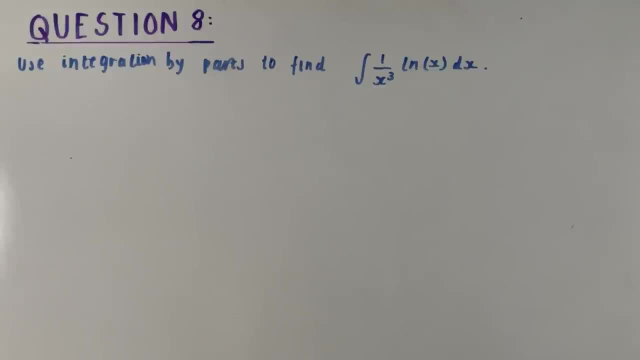 at the point zero For question number eight. We're going to be doing some more integration, A bit of further integration here In this integration question. we are strictly told. 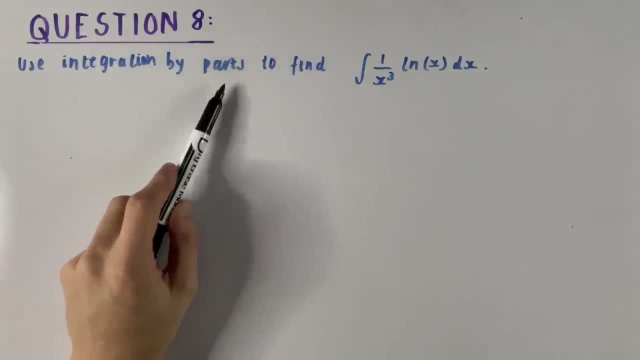 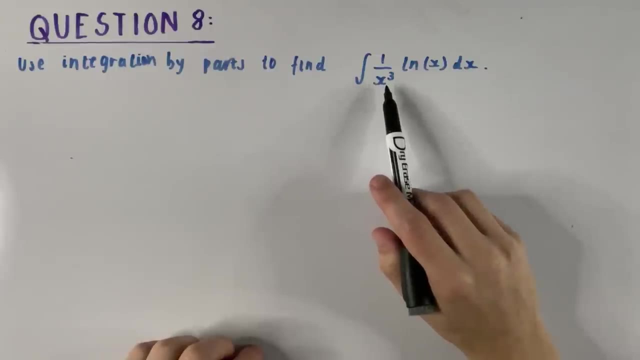 use integration by parts to find the derivative of one divided by x cubed, multiplied by the natural log, which is ln of x, dx. Okay So, 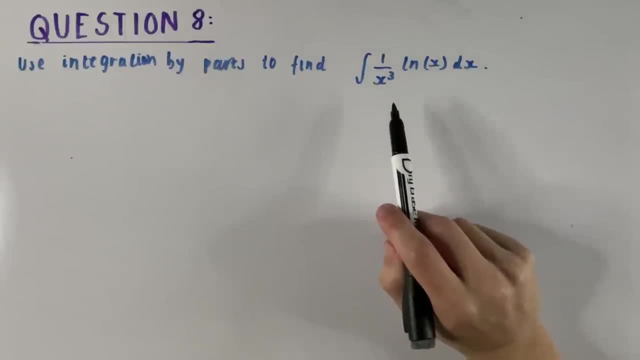 integration by parts can be quite fiddly, but again, I will give you our formula: integration by parts, for those that either don't already know it or have forgotten it. So, basically, to evaluate this integral: 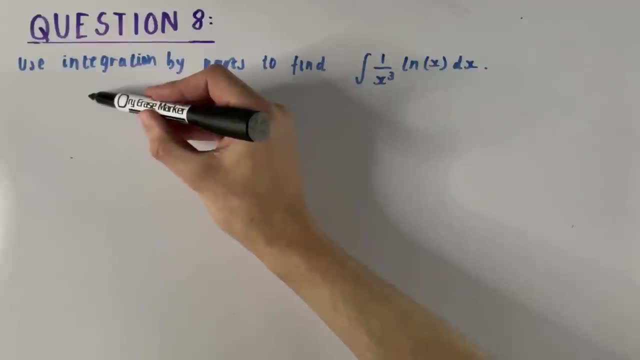 we're going to say that the integral, we're going to just sub in some different values. we're going to say u v dash is equal to u v minus. 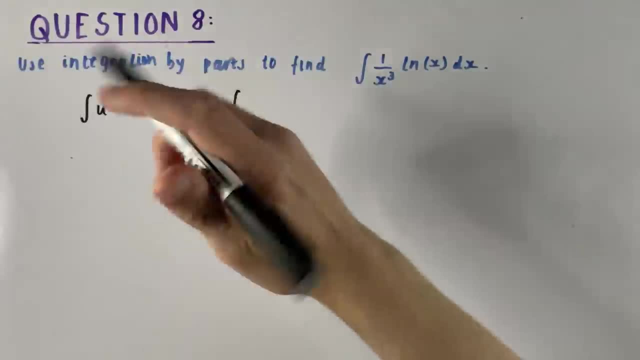 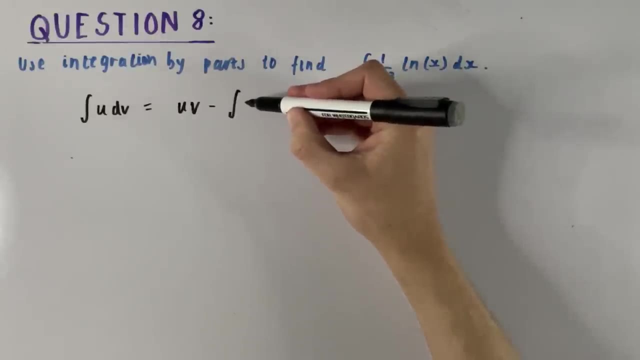 the integral. actually We'll write. we'll write: u dv in our case is equal to uv, the integral of v d u. So this is just a little formula that we can use. 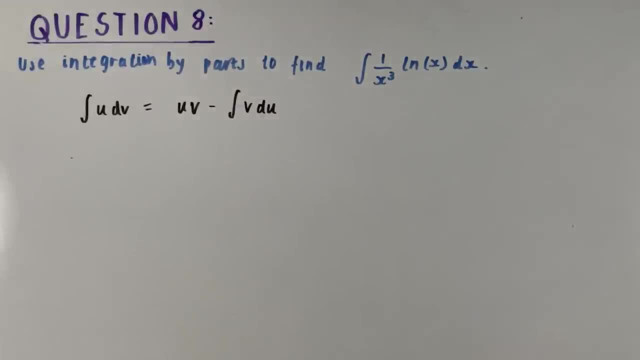 to evaluate the integral by doing integration by parts. Now, similar to like we did earlier with the product rule, I'm going to do a little working at the side To work out what u v dv. 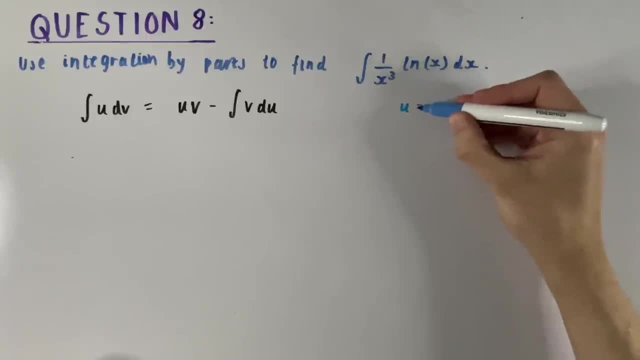 and du are Now. when doing integration by parts, you want to look at which one is going to be easier to integrate And which one is going to be easier to differentiate, Because our 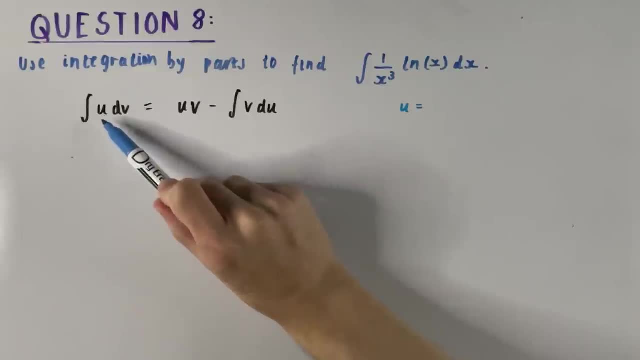 formula that we have is u- dv. So u is some function that we're going to differentiate And dv is some function that we're going to integrate. Now I can tell you straight by looking at this: 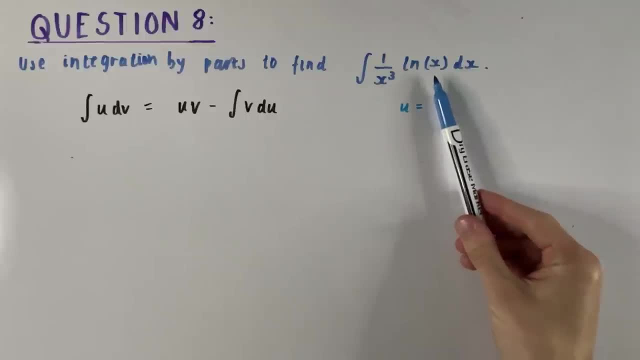 that I want to differentiate the natural log of x, Because that is just going to become 1 over x by our differentiation rules And this looks like it's going to be easier to. 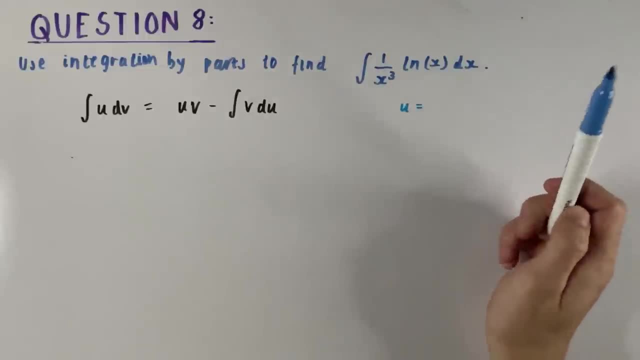 um, integrate as well anyway. So that's what we'll do. So our u, in our case, is going to be the natural log of x, Because du is going to be 1. over x. 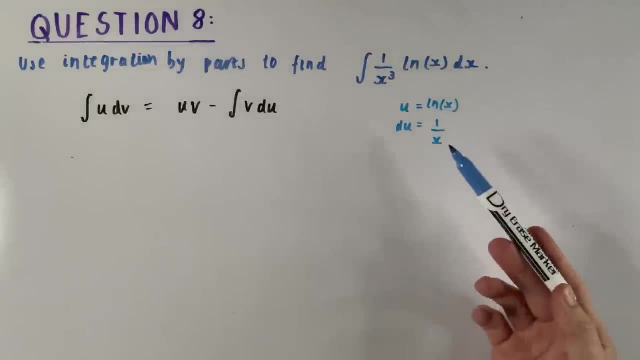 Now again, this is just a differentiation rule. There's proofs for it out there that I'm sure you'll find, but I won't get into it in this video. Now our dv is this thing here: 1 over x cubed. 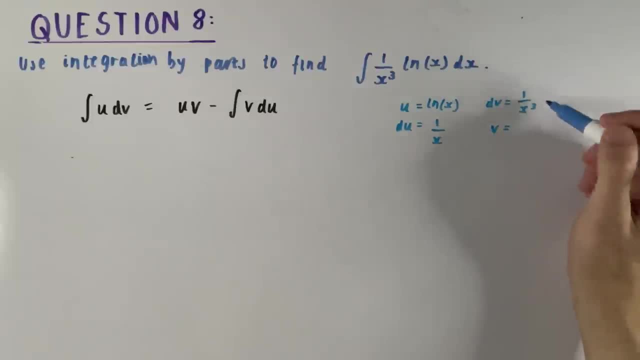 We want to integrate that, to work out v. So, integrating this, we are going to just to say that this is x to the minus 3.. It's the same thing essentially. So, integrating that, increase the power by 1.. 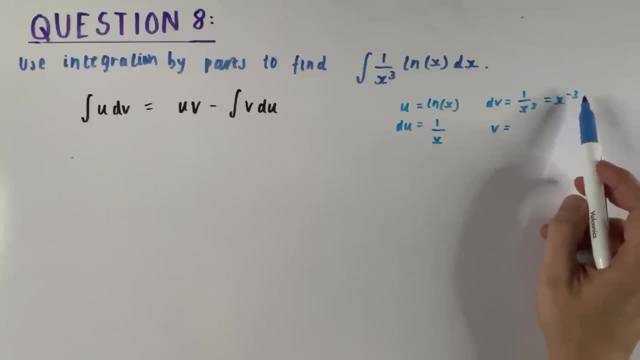 So it's going to become x to the minus 2.. Divide by the new power, Which is dividing by minus 2.. Now, dividing by minus 2. we're just going to say is minus a half, And then x. 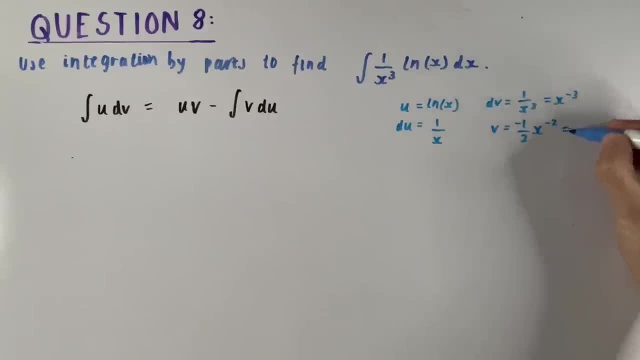 to the minus 2.. Now, actually I am going to rewrite that As minus 1.. over 2x squared Like so, Just to make it nicer for us. So now that we've got, 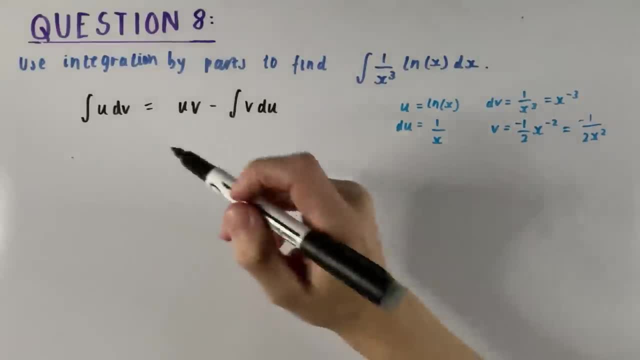 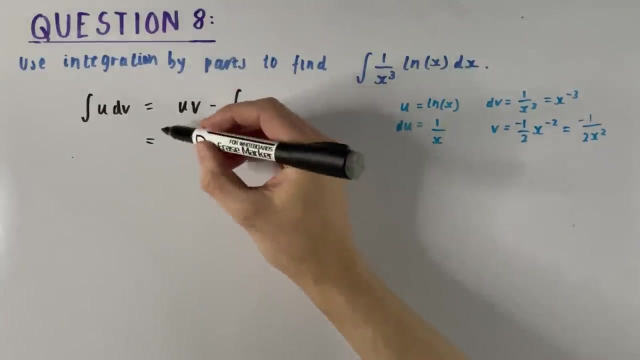 our values of everything. here we can evaluate the integral. So let's substitute, substitute, substitute our values in. So we begin by working out u times v. We can just write this as: 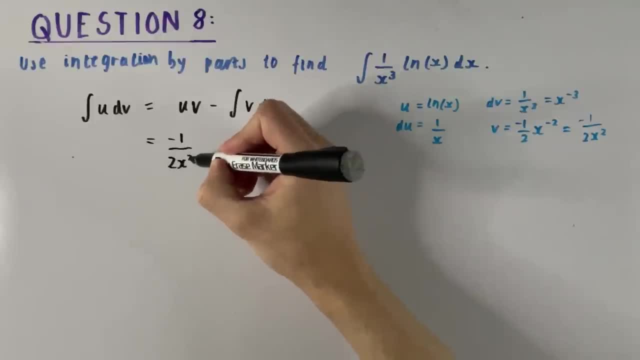 minus 1.. over 2x squared Natural log of x, And we are going to hope I have enough space for this subtract, the integral of v, du. So this is going to be: 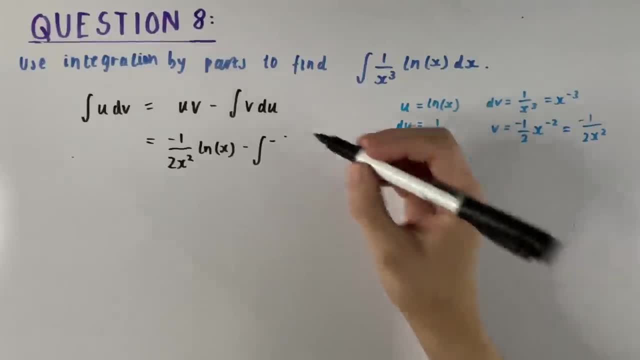 minus .1.. Actually, I've noticed that when we multiply these together, we're going to get minus 1 over .2x cubed, Because 2x squared times x is 2x cubed. 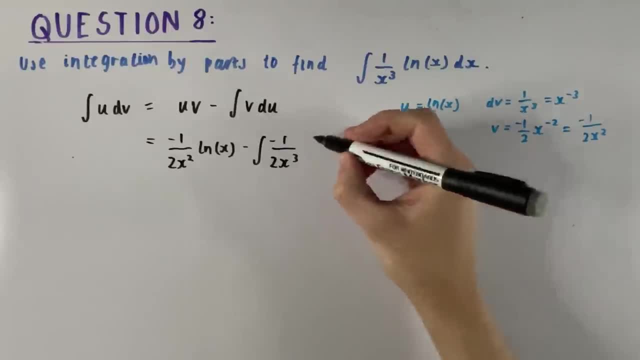 So minus 1.. over 2x cubed. Don't forget our little dx. Now we can actually simplify this further because we have this factor of minus 1 half. We can just pull that out of the. 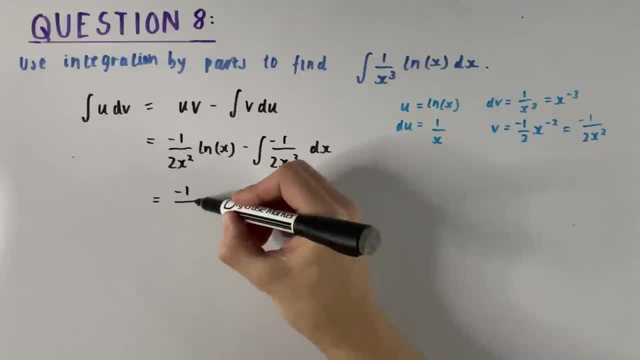 integral. So let's do that. This constant, I should say, is not really going to change. So when we pull out a half, we get plus a half times the integral of, and it's going to be 1 over x cubed. 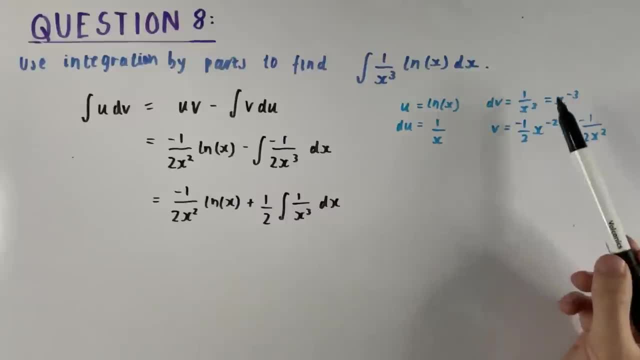 dx. Now, luckily for us, we've actually already done this, so it's even easier for us. We can just say: this is minus .1 over 2x, squared lx percent of x, And then we're going to do: 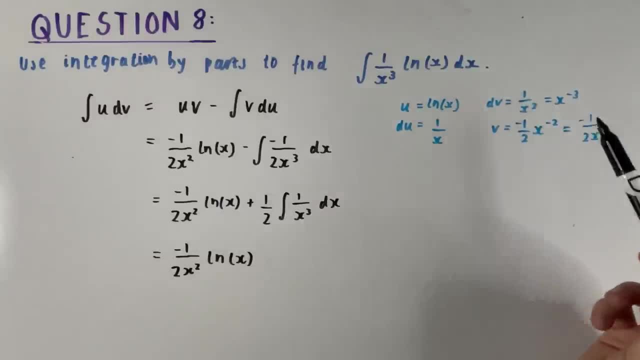 a half times this thing here, So it's just going to be um plus .1 over um. actually, let's just do it like this: a half times the integral of this. 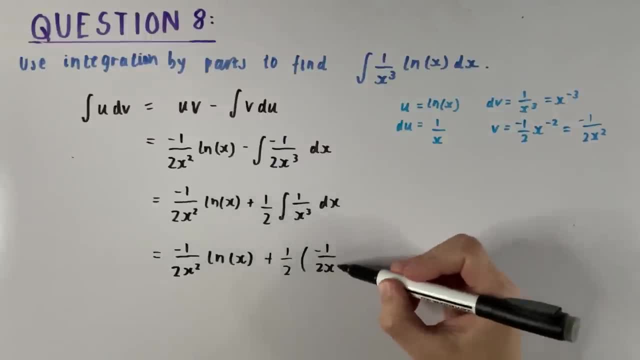 which is minus 1 over 2x squared. And the reason I've done it like this is to show you that we can simplify this bit here to get minus 1 over .4x. 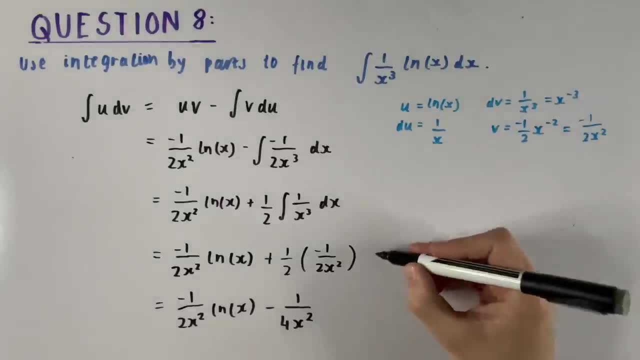 squared like so, Oh, and we need to make sure we remember our constant of integration like that. So a bit of a more complex integration question, but we got it done in the end and it was. 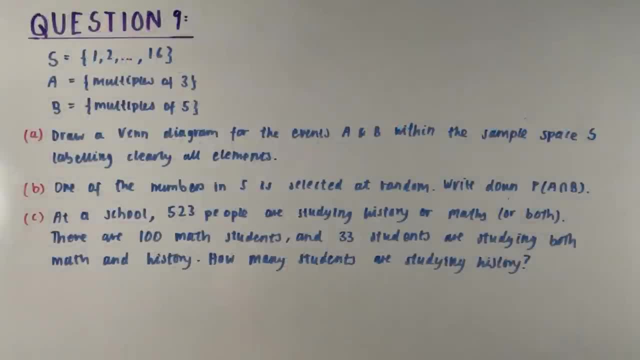 not too bad. So, guys, we're going to be moving on to question number 9.. which is the second last question in tonight's video, And we're going to be doing what looks to be. 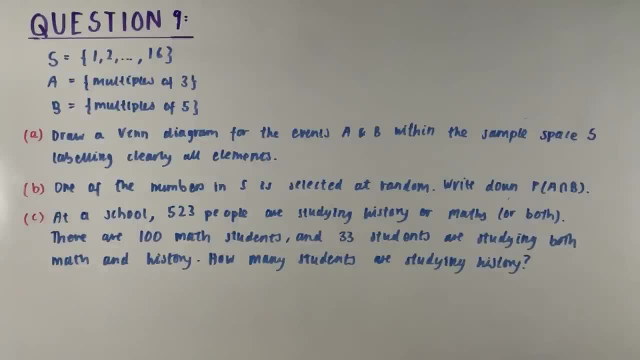 a bit more statistical, statistical analysis. Some statistics here. So let's take a look at what this question asks us. So we are initially given three sets, or it looks to be. two of them are events. 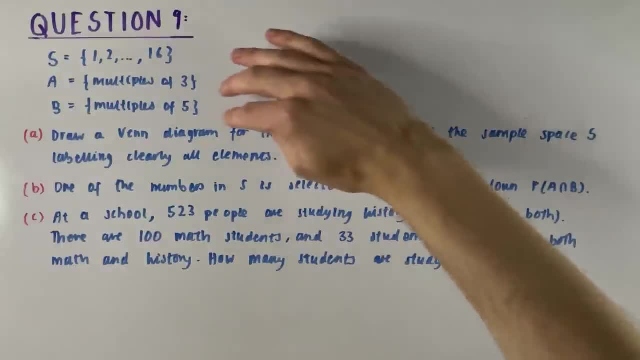 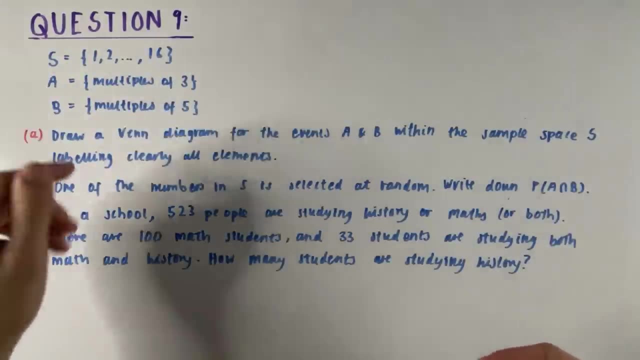 and actually, well, technically they are sets, but we've got three sets. We have the set S, which is the numbers 1 through .16.. We have the set A, which is the set of all multiples of. 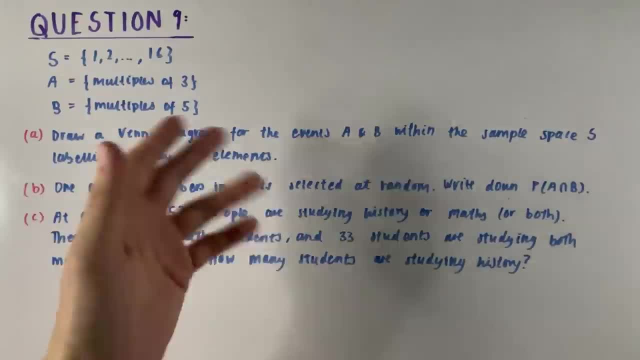 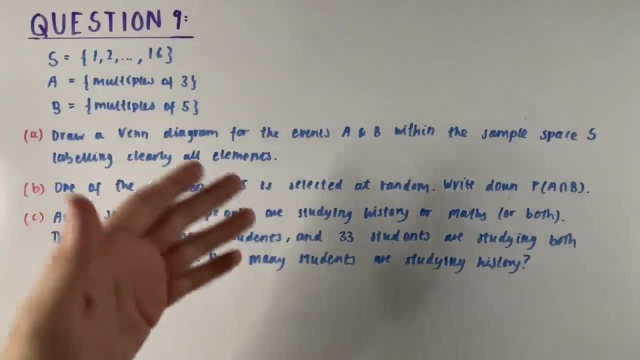 .3.. So that would be .3,, 6,, 9,, 12.. um so on. And .3 is the set of all multiples of .5. So 5,, 10,, 15.. 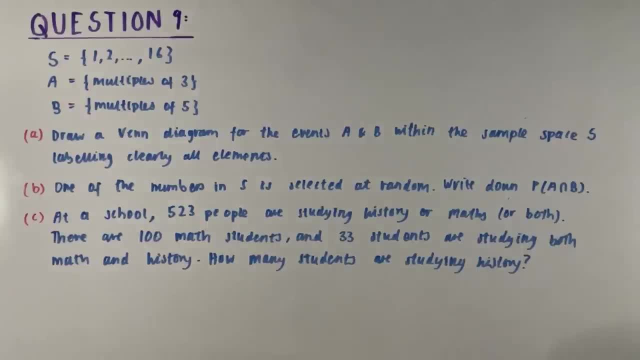 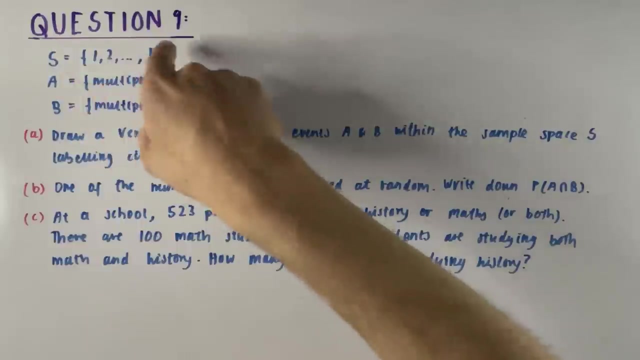 .20 and so on. Part A asks us to draw a Venn diagram for the events A and B within the sample space S. So that's the sample space. So these 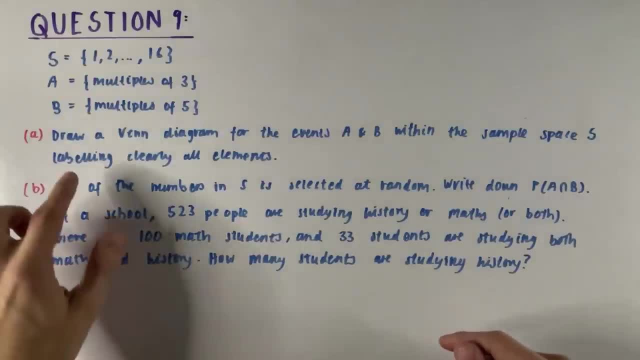 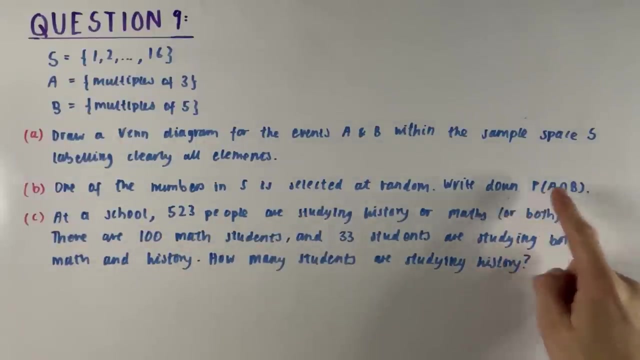 occur within those numbers. it all makes sense Labeling clearly all elements. Part B says one of the numbers in S is selected at random. Write down the probability of A intersect B. 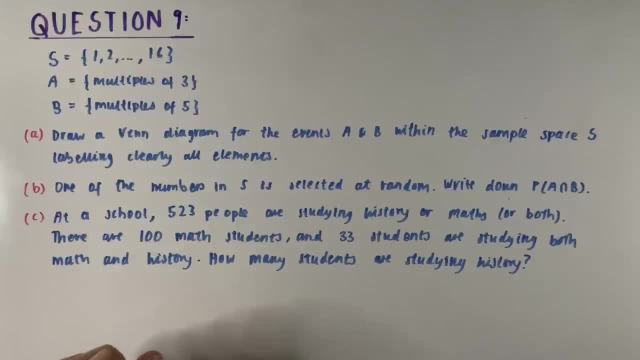 And for part C, we are told this looks like an entirely new question- umat a school .523.. people are studying history or maths, or both. There are 100 maths students. 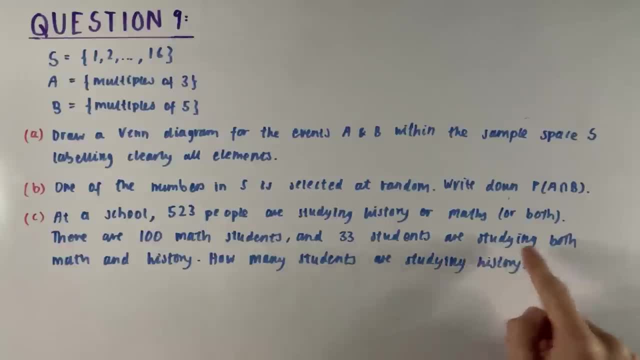 and 33.. students are studying both maths and history. How many students are studying history? Great, So bit of probability, probability, probability, probability. So let's tackle this question by. 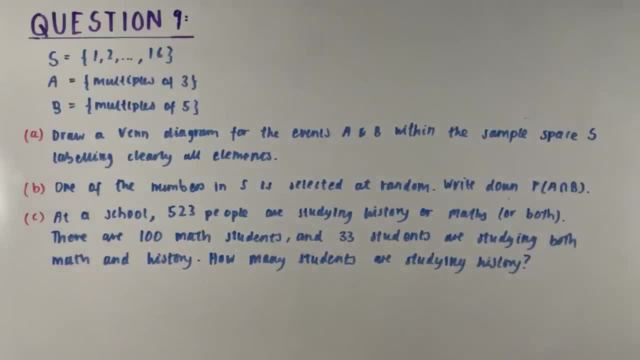 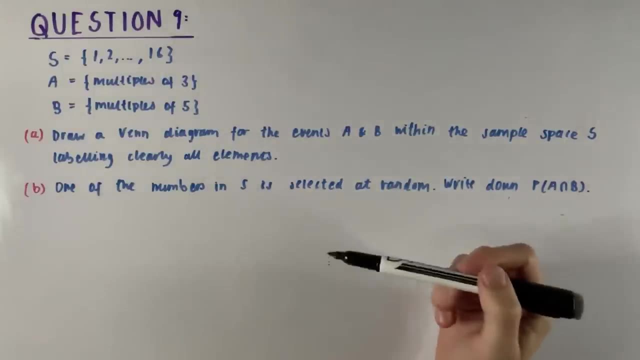 first drawing this Venn diagram. So I've kept question A and B up because they're both about this question here. So part A asks us to draw the Venn diagram for the events A and B. 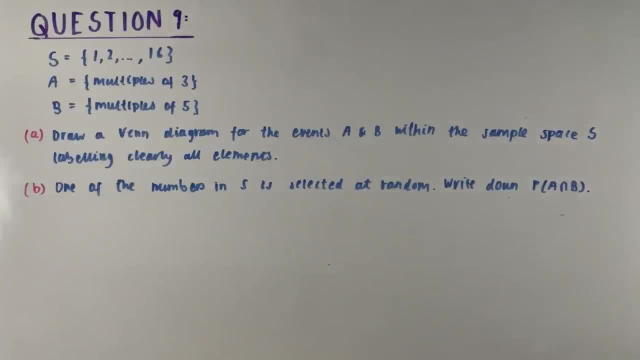 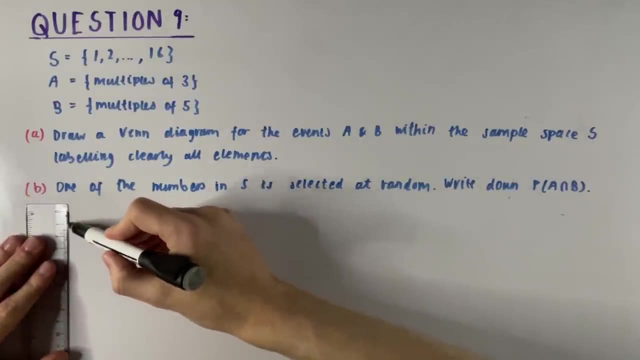 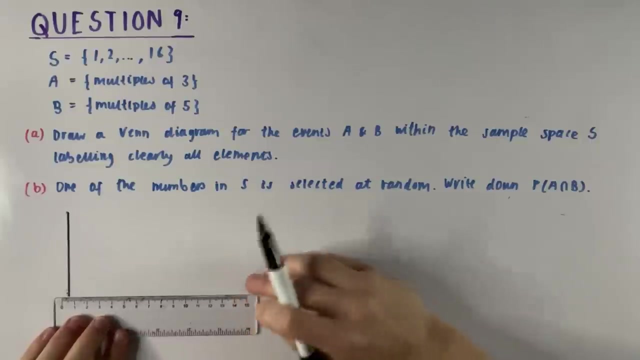 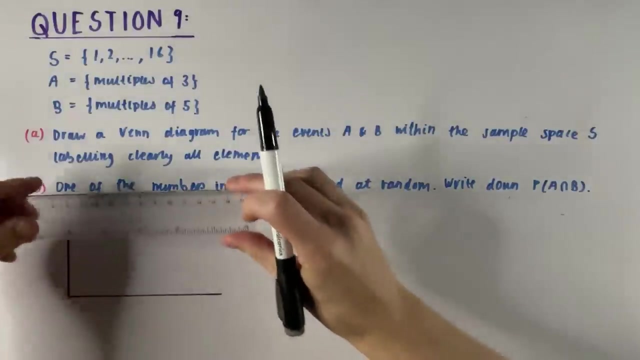 within the sample space S. Okay, so let's begin by drawing our sample space. um, we'll just do a nice rectangle using our ruler, like. so you have to bear with me, I'm trying not to. 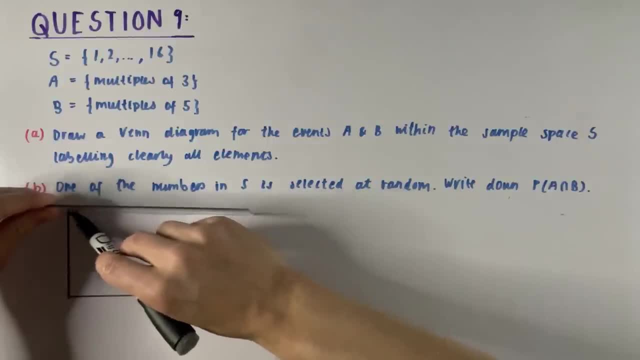 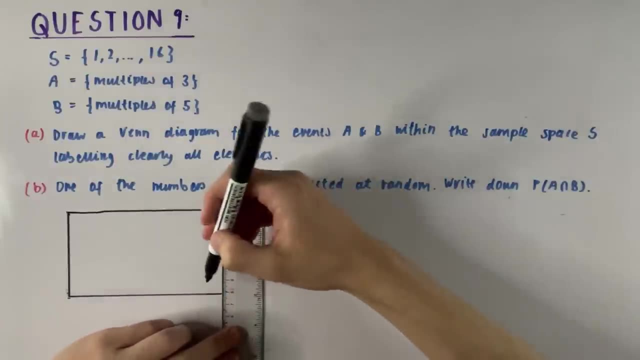 get the ink everywhere because it will- oh, it's very wonky whoops- and then down here like: so this is going to be our sample space, this early drawn rectangle. 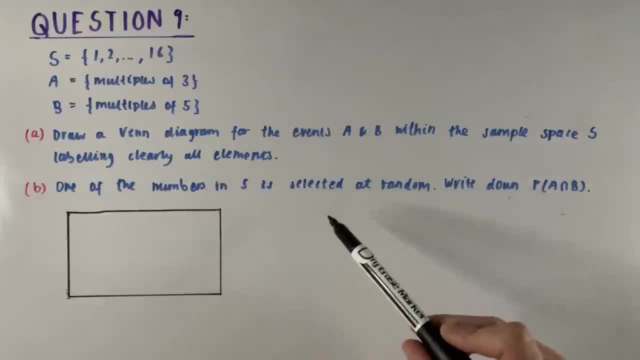 now the events A and B. now from part B we can actually see that they do intersect. so we're going to try and draw two circles that intersect. so let's do one circle like this. 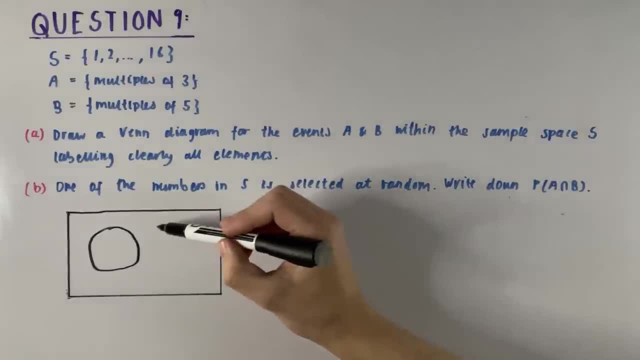 obviously it's a terrible circle, but I'm freehanding this and another circle like this. they don't even have to be circles, really just blobs will do- and let's label this. 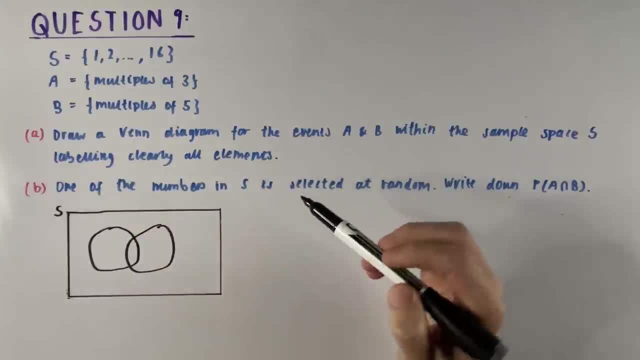 S as our sample space, because we've got to label clearly all elements and then we've got the events A and the events B as these blobs. so we want to label clearly all elements. 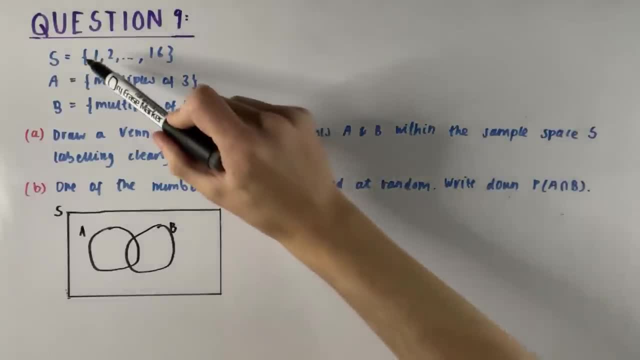 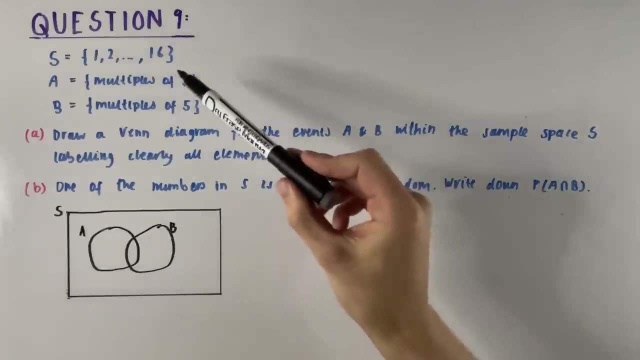 so the elements in the sample space are the numbers .1 through 16, so all of them have to be within here, however, the multiples of 3.. within the sample space, so all multiples of 3.. 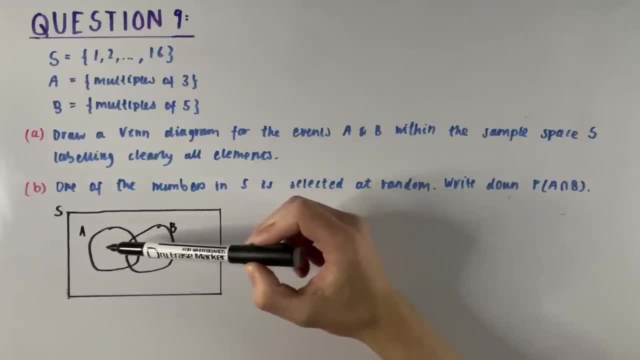 from 1 to 16.. must be in A, all multiples of 5. within 1 to 16.. must be in B and all multiples of 3. and 5. in S. 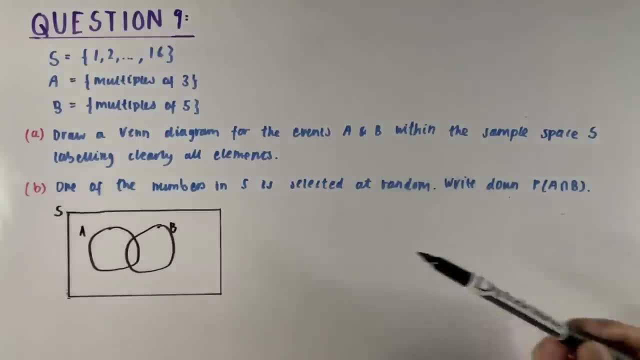 must be in this little gap in between, which is the actually the part for we need for part B. so let's do this. so, starting off with the number 1.. this is not a multiple of 3 or 5.. 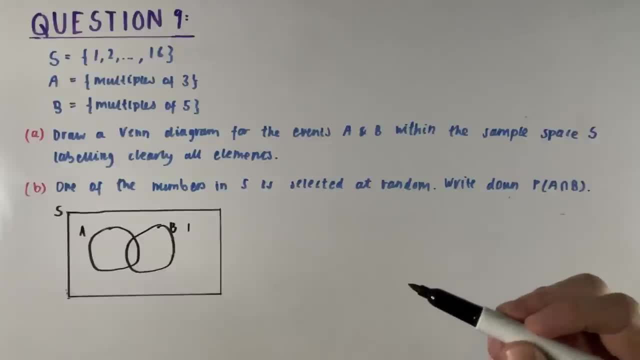 so we'll put that outside both events. same with number 2.. put that outside both events. number 3, however, is a multiple of well, A is a multiple of 3.. so 3 is a multiple of 3.. 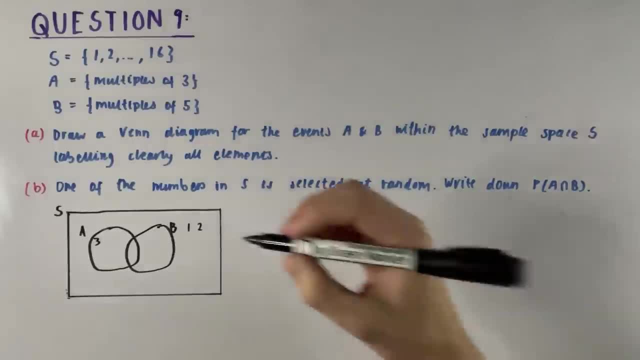 we'll pop that inside, A number 4.. again, outside, it's not a multiple of 3 or 5.. .5, however, is a multiple of 5.. it's not a multiple of 3.. 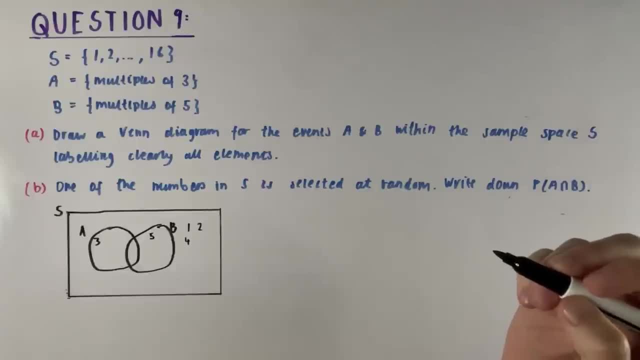 so it just goes in B: .6. is a multiple of 3. but not of 5.. .7. is neither a multiple of 3 or 5. .8. is a, not a multiple of anything again. 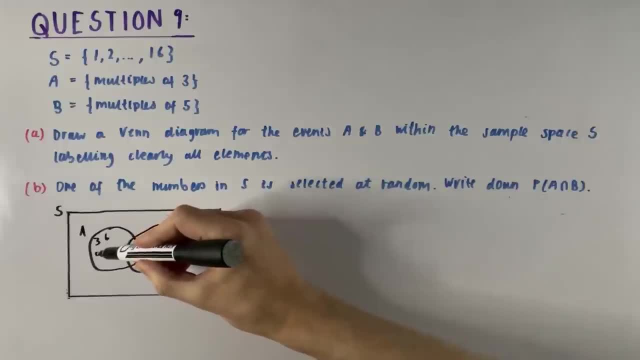 .9.. is a multiple of 3.. stick that in there. Ten is a multiple of five, but not of three. Eleven is not of three or five. Twelve is a multiple of three but not of five. Thirteen is neither a multiple of three or five. 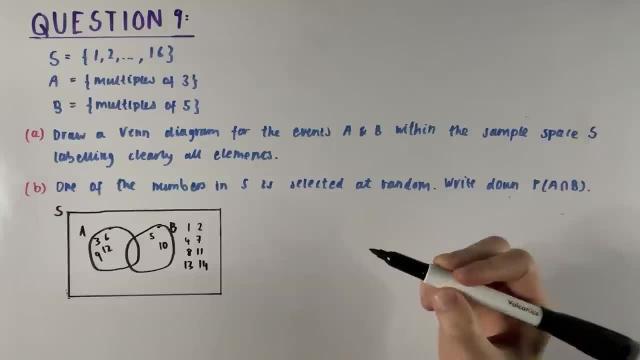 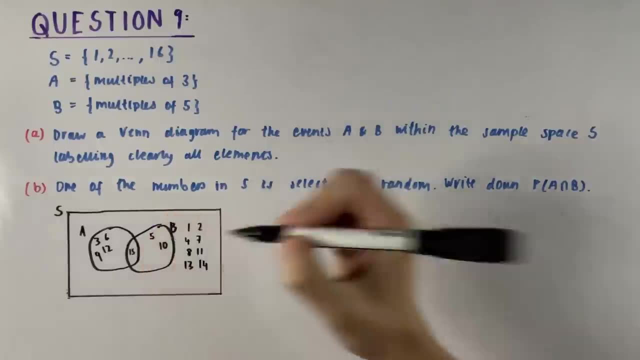 same with fourteen. Fifteen actually is a multiple of three and five, so that we've got to try and squeeze in here like so. And then sixteen is neither a multiple of five or three. so that is our Venn diagram complete. Part B says one of the numbers in S is selected at random. Write down the. 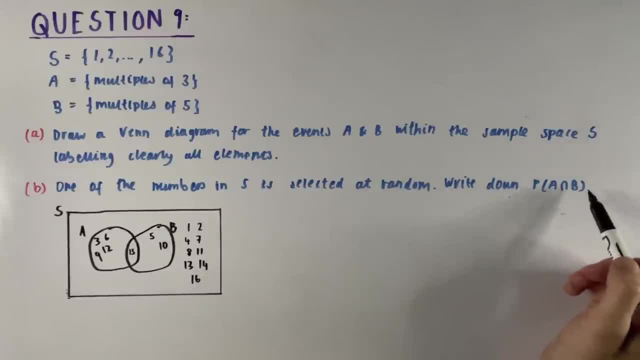 probability of A intersect B. So that is the probability that out of all the numbers in S, which is one to sixteen, the probability that the number is A and B. And now A and B means, let's write out, A intersect B is the probability that it is a multiple. 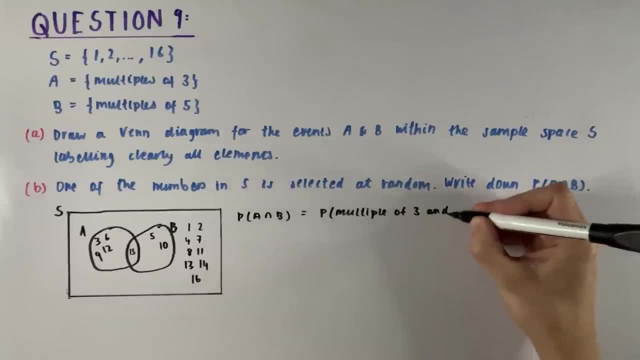 of three and five. Now we know there's only one number, so we're going to have that. this is one over the. what do you call this? again? one over the- oh god, I've forgotten the name, but it's one over the amount of elements in S. It's the absolute value, but it's not. 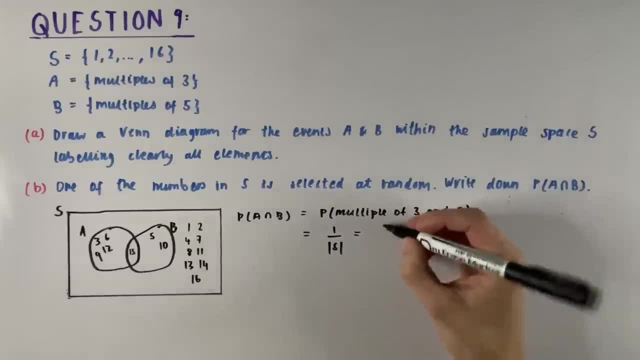 it's just the number of events, the number of elements in S. So the number of elements in S, well, we know it's one to sixteen, so it's one over sixteen and that is our probability. We can see there's one number out of sixteen, numbers that are a multiple of three and five. So the probability, 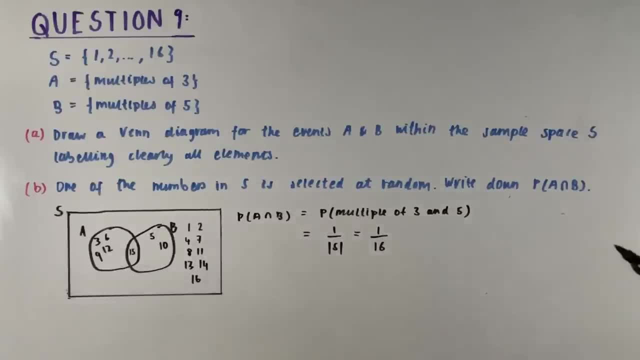 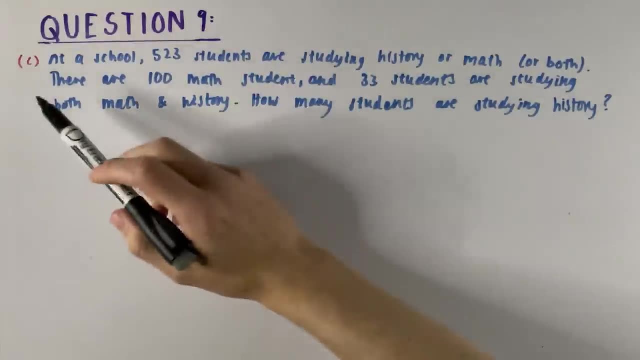 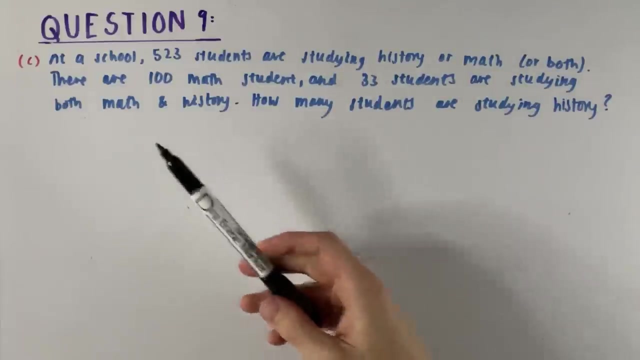 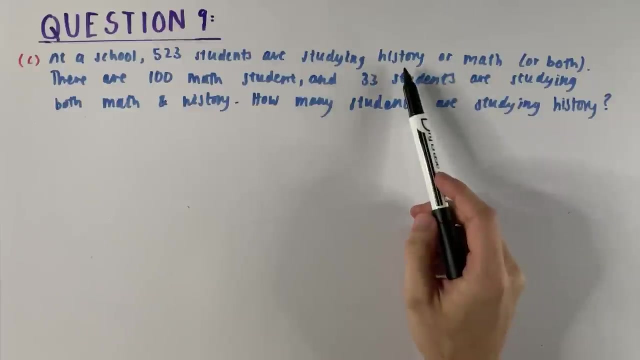 of one picked at random, is one in sixteen. Moving on to question number three in question nine, part C, I should say We've got this nice wordy question which I'll re-read for you. So at a school, 523 students are studying history or math, or both. There are 100 math students and 33 students are. 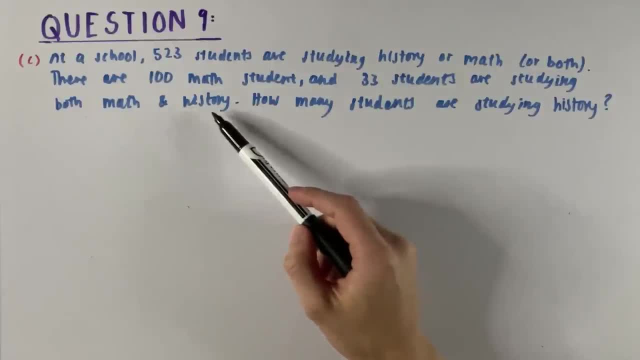 studying both math and history. How many students are studying history Now? when you study statistics or probability, you learn quite a lot, and I mean a lot of um, let's say rules and axioms, and lots of theorems and things like that. So 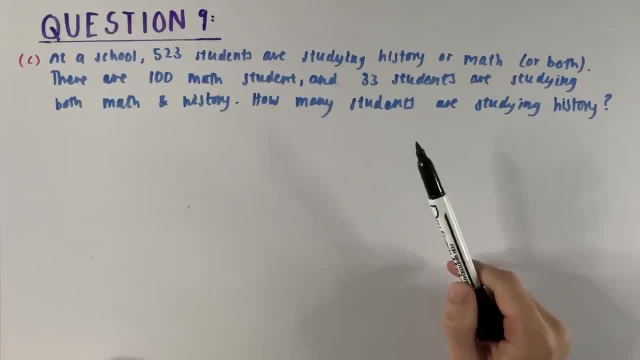 when we look at this question, although it seems all over the place, there's a very nice rule that we can use to work out how many students are studying history, and it's a probability rule. a probability rule And this rule, which I'll write down the name for in light blue, in case you guys want to go, 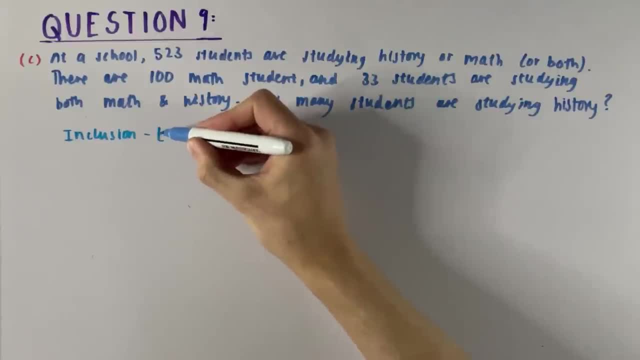 and do some reading about it, but it is called the inclusion exclusion. I think they call it a principal. le right al is a principal, like a principal teacher, I don't know. so the inclusion exclusion principal. is that the right spelling of principal? I don't even know, i'm terrible at english, but this rule or this principle states that the probability 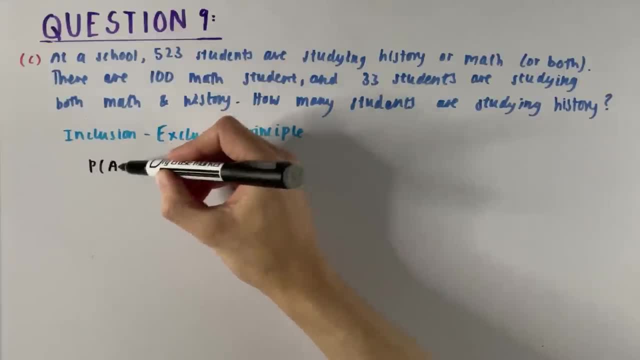 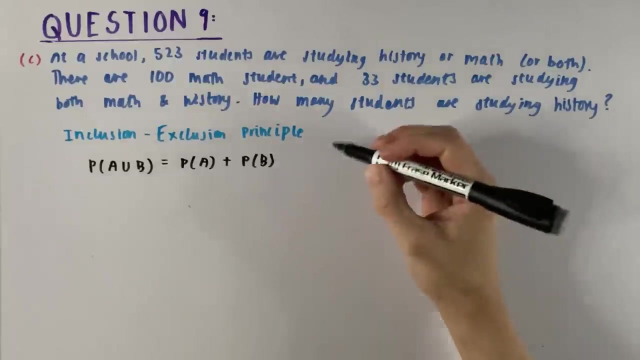 of um an event a and the event b occurring is equal to the probability of of A occurring plus the probability of the event B occurring. Subtract the probability of A intersecting with B. Now we can visualise this using some Venn diagrams. again, Let's 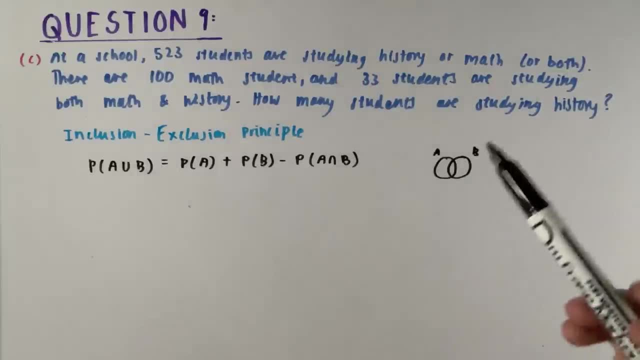 call this A and this B. So what A union B means is A or B, So both of them combined. So that is going to be this. It kind of looks like this. That is this entire space in here. Now we can see that this is A plus B, minus A intersect B. 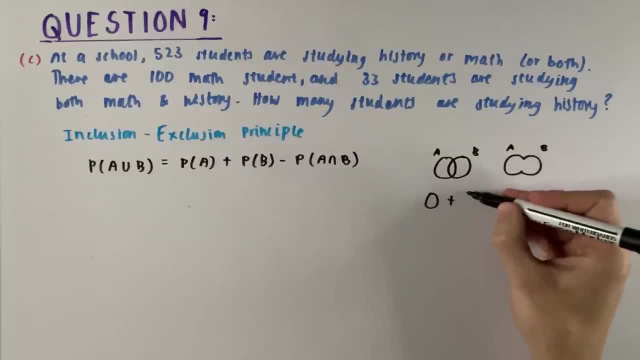 Now we can see that this is A plus B minus A intersect B. Now we can see that this is A plus B minus A intersect B. So when we have this, we've got A plus B plus this extra bit in the middle. Now we don't. 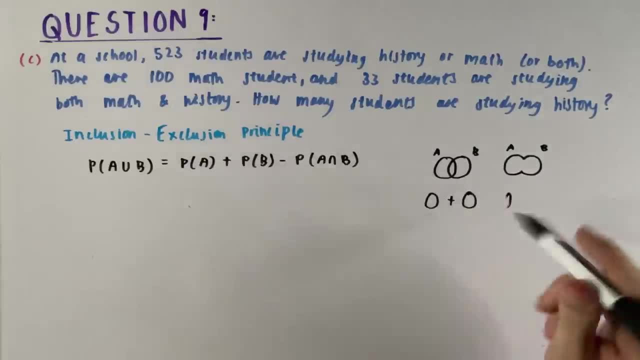 want this extra bit in the middle. We want to get rid of that. So if we subtract that, we are subtracting this bit here, So we don't count it twice, If that makes sense. So, applying this principle to our question, we can say: well, we've not actually got any probabilities here, We've got values. 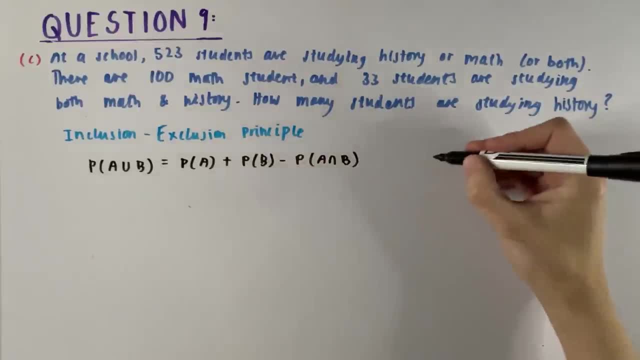 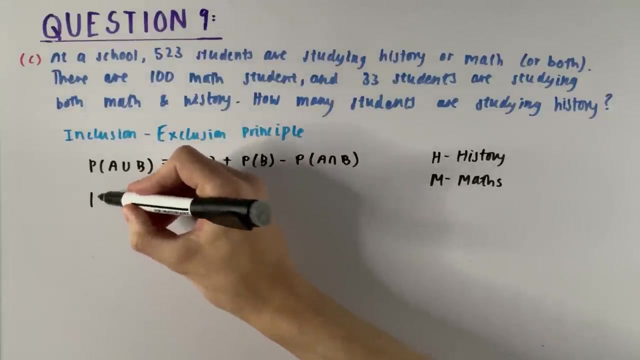 So let's say H is a student studying history And M is a student studying math- I say maths, but people sometimes say math. So we can say that the value of students studying history or maths- It looks like um- is equal to the number of students studying history, plus- and this is 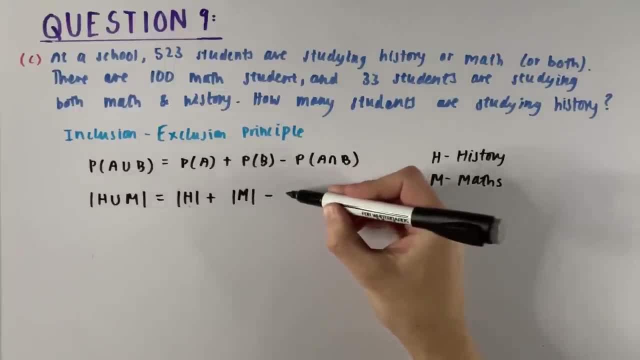 going to be the number of students studying math Subtract the number of students studying history and math. Now we are given some of these values in the question. We are told that the number of students studying history or math is five hundred and twenty three. 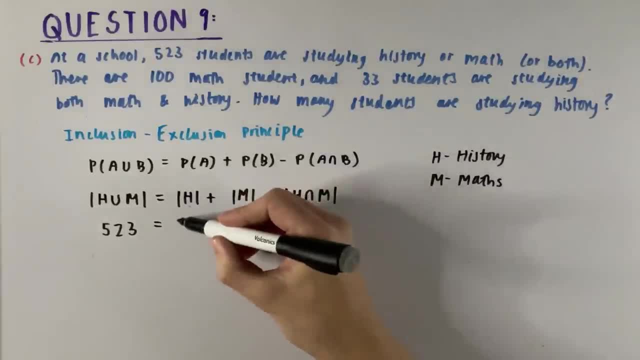 Now we want to work out the number of students studying history. so we don't know that. However, the number of students studying just math is one hundred, and the number of students studying both math and history is thirty three. Now we can just rearrange this to solve for. 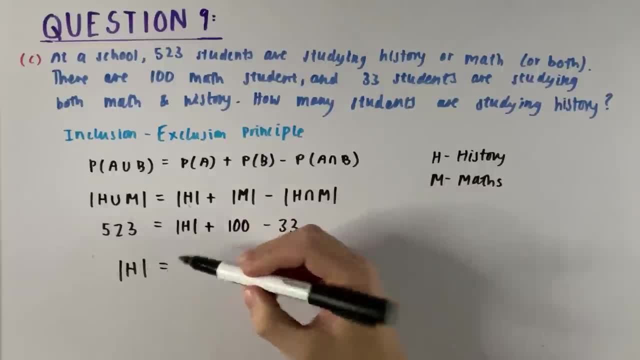 the number of students studying history. So we're going to have this is going to be six: 67.. 523 subtract 67 is 456.. So that is the number of students studying history. So we'll see There are 456 students. That's quite a lot Studying history, Like so. However, some of 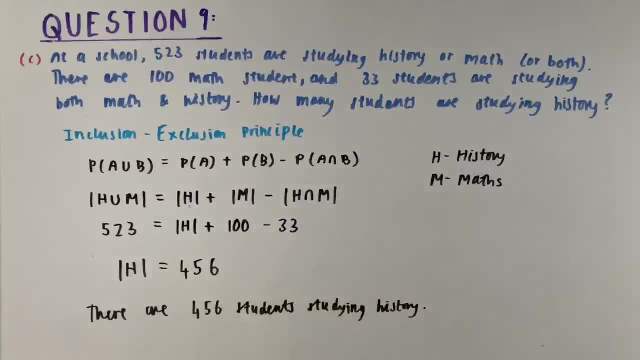 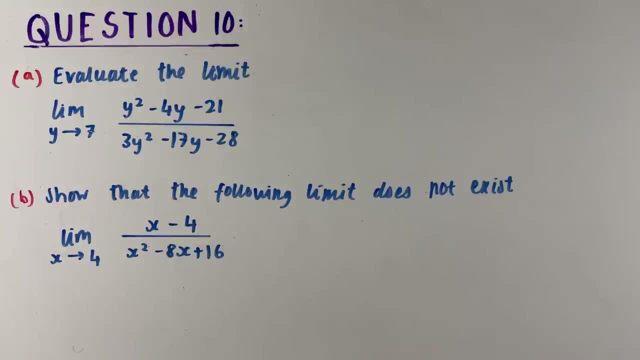 these are studying history and math. So good on you, students In the last question in tonight's video, question number 10.. 1, 2, 3, 4, 5, 6, 7, 8, 9, 10, 10, 9, 8, 7, 6, 5, 4, 3, 2, 1.. 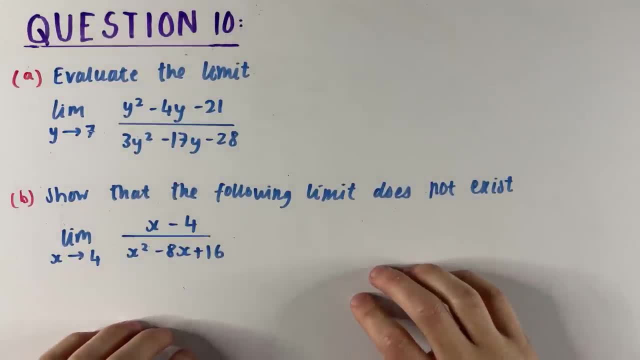 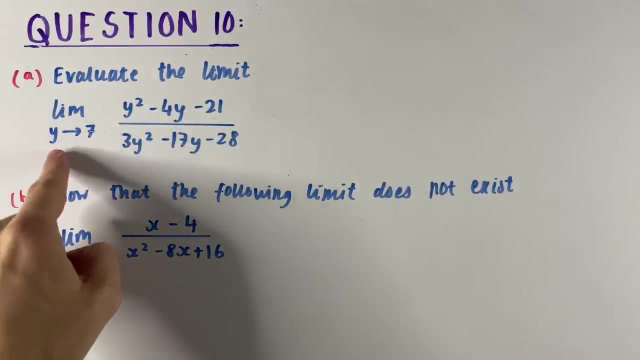 We have a question about limits, A bit of calculus going on here again. So we have two questions. The first question says to evaluate the limit, The limit as y tends to 7.. 3y squared minus 4y minus 21, divided by 3y squared minus 17y minus 28.. And part b is: 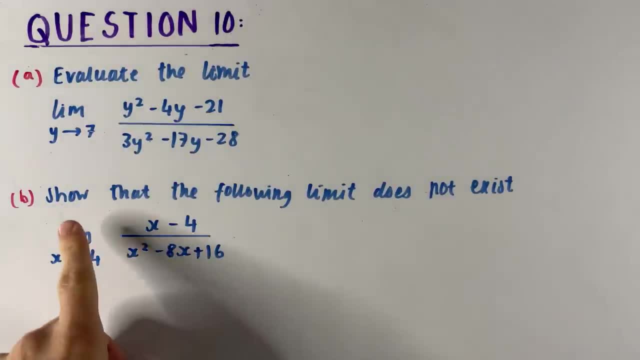 a slightly more tricky question that asks us to show that the following limit does not exist. The limit as x tends to 4 of x minus 4 divided by x squared minus 8x, Plus plus, plus plus 16.. So let's have a go at this. So for part a, we want to evaluate 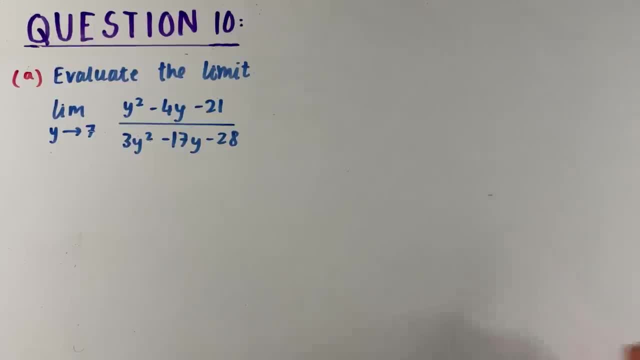 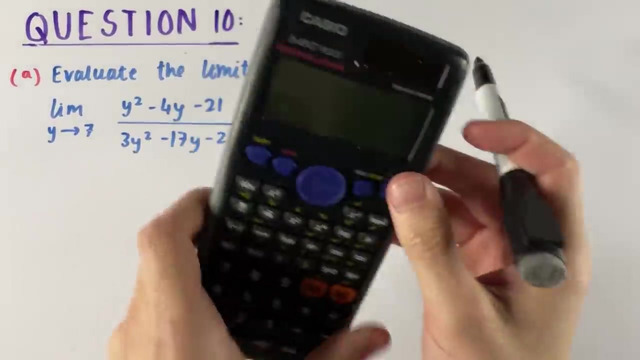 the following limit. Now we can see that when we substitute 7 into this equation, we're going to get 49 minus 28,, which is 21.. Subtract 21,, which is 0.. And this is going to be divided by 7 squared. Oh wow, I'm going to have to do a calculator. 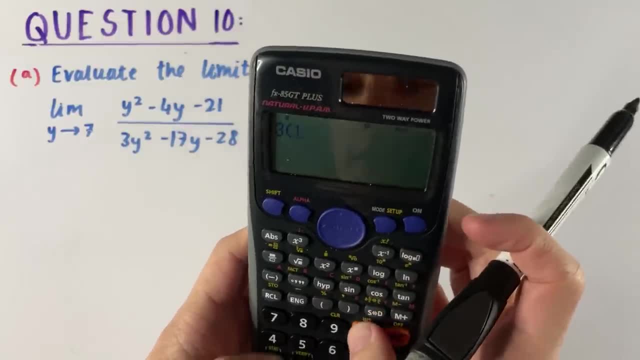 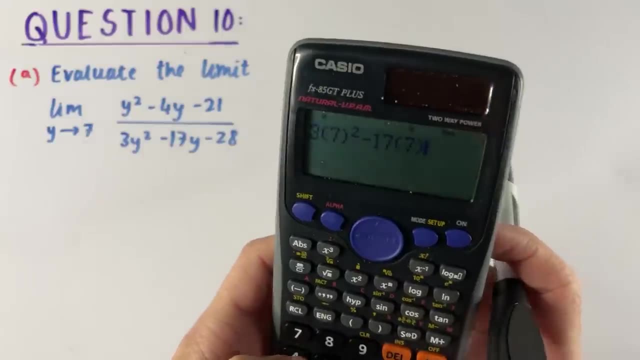 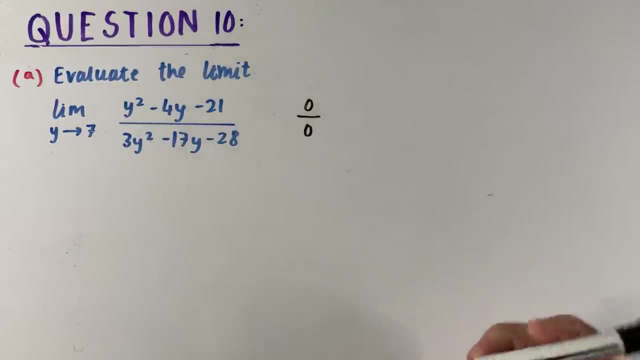 for this bit: 3 times 7, squared minus 17, times 7 minus 28, also gives us 0.. So we need to do: obviously: 0 divided by 0 is undefined, It's an error. So we need to do a bit of manipulation, Manipulation 2. The limit that we are solving. 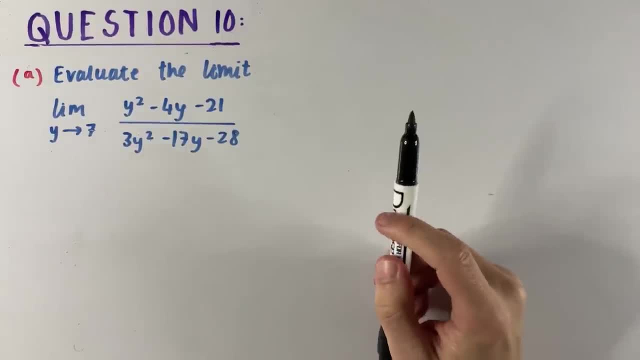 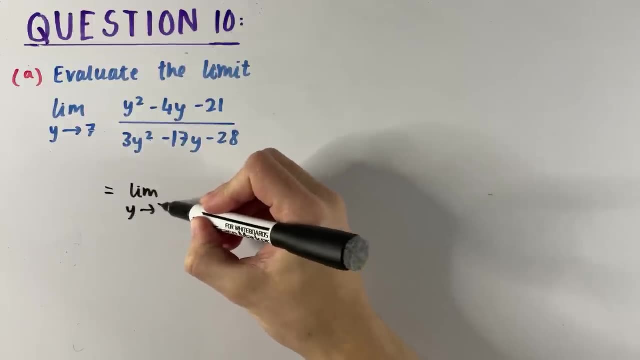 before we work out the limit. So we can say that this thing here is the same as the limit, as y tends to 7.. You know what? Let's just factorize the top and the bottom parts of the fractions. So on the top we have the top and the bottom. 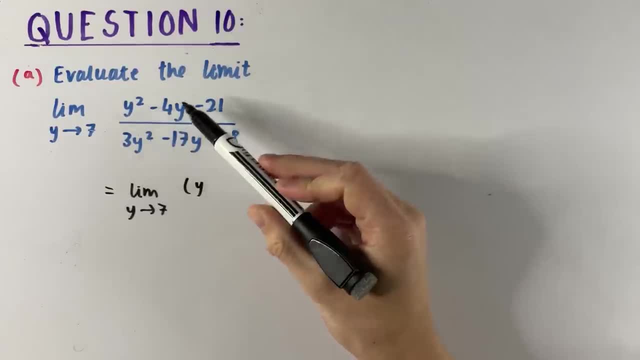 On the top part, we're looking for factors of 21 that we can make 4 with or minus 4, I should say 7 and 3, we've got minus 7,, yep, plus 3.. Now I'm immediately thinking on this bottom part of the fraction. I think we're trying. 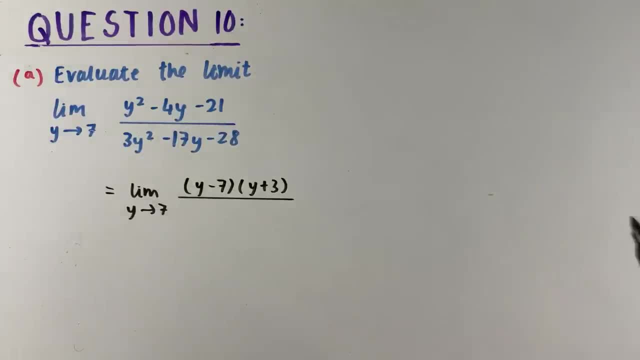 to look for another bracket that will look like this. So let's see if we can use one of them. Let's see if we can work out this. Well, we're looking for factors of 28, so 7 would make sense. So I think y minus 7 is going to be one of them. Let's just assume that. 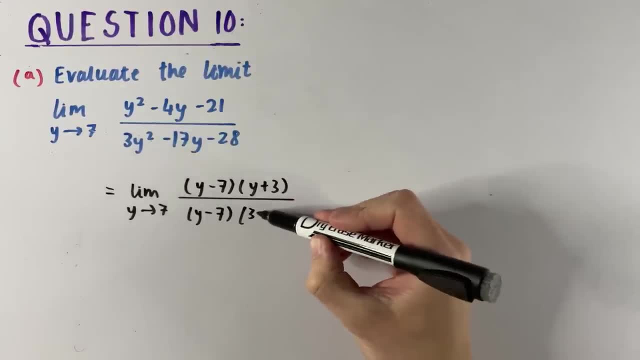 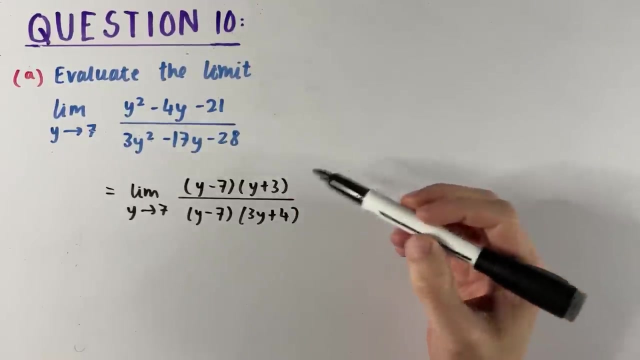 it is. and the second one? ah yeah, the second one is going to be 3y plus 4, because this will give us 3y squared minus 21y plus 4y, which is minus 17.. Y and then minus 28,. so that's all good, And this is also the same as the limit, as 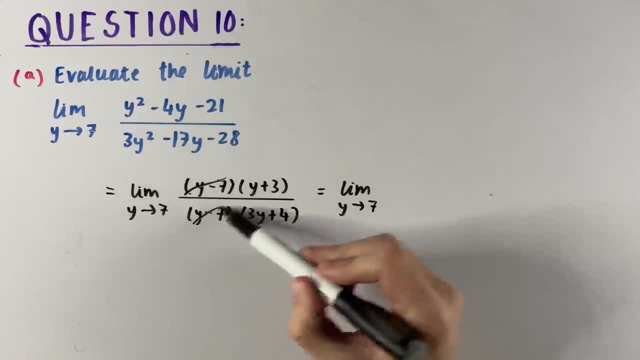 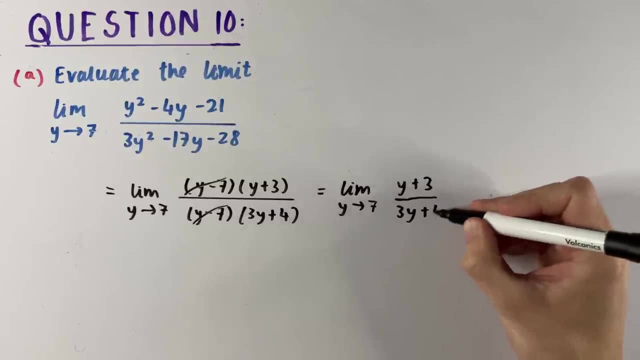 y tends to 7.. We've got these that can cancel out, So we've got y plus 3, just don't use a ruler again. Always use a ruler. guys, don't take advice from me. Sorry, this have I written. 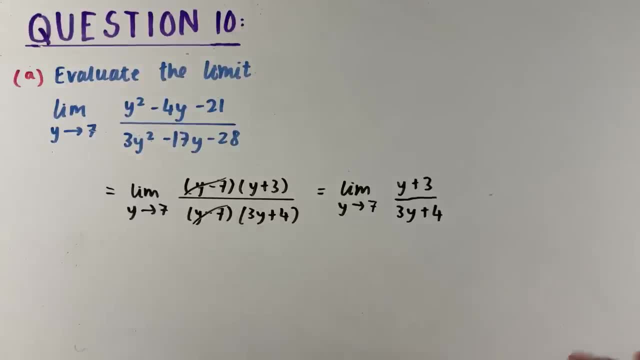 that out? right? I think I have. yeah, that's all good. Now let's see what happens. if we sub in, y is 7.. Now we're going to have 10 on the top, which looks good. 21 plus 4 is 25 on the bottom. So this is going to simplify. 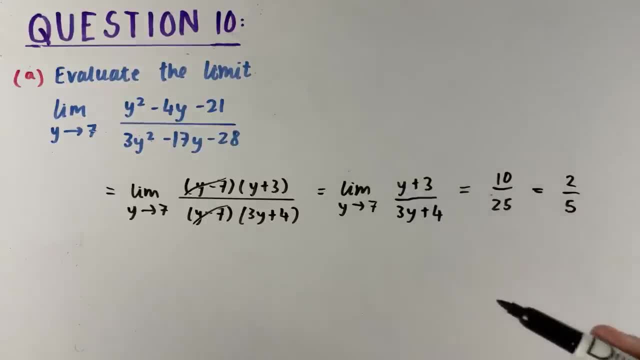 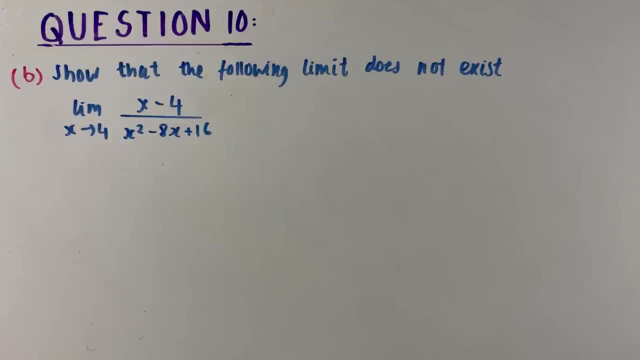 to 2 over 5, which looks good. So that is us evaluated that limit. For the second part, part b, we want to show that the following is going to be the same as part b. So we want to get the following limit. So we want to get the following limit. 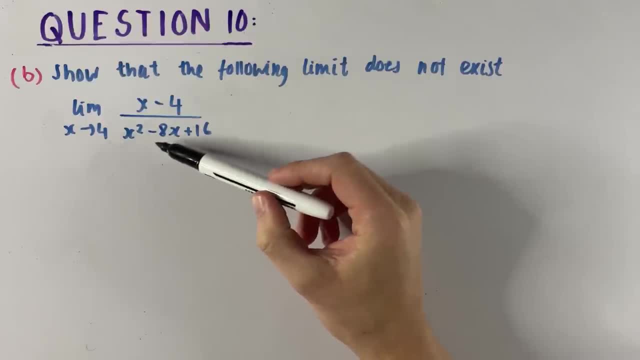 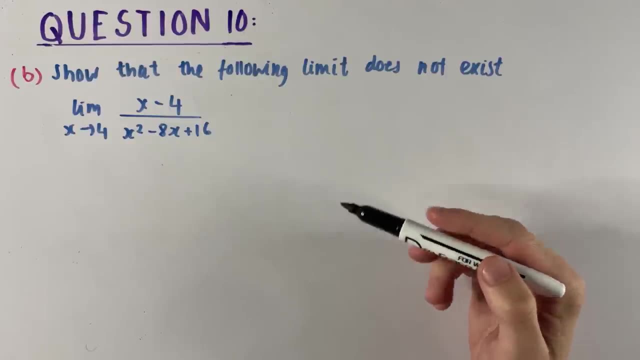 as X tends to 4, which is x minus 4 over x squared minus 8x plus 16.. So kind of like the question before: when we try and sub in the value as 4, we're going to get 0 on top. 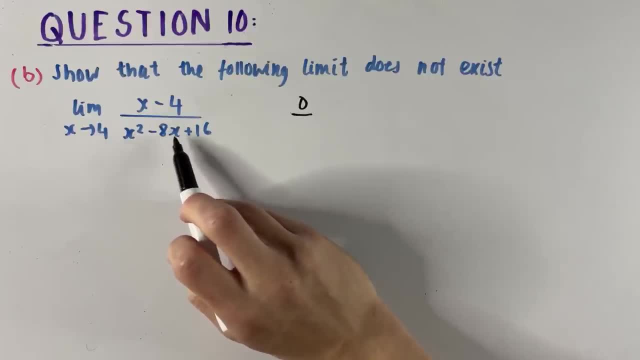 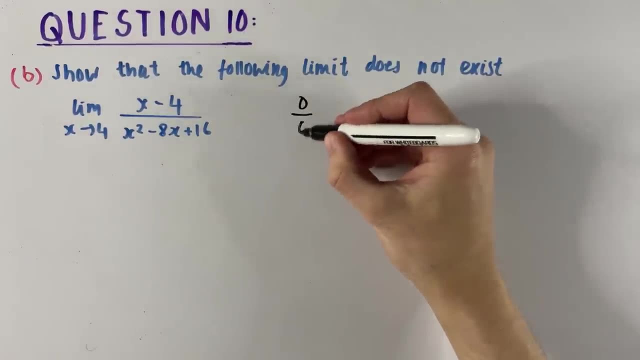 them, we've got: 4 squared is 16 minus 8 times 4, which is 32, and then plus 16, so that's going to be 32 minus 32, which is 0.. So again we have this statement that doesn't make sense. 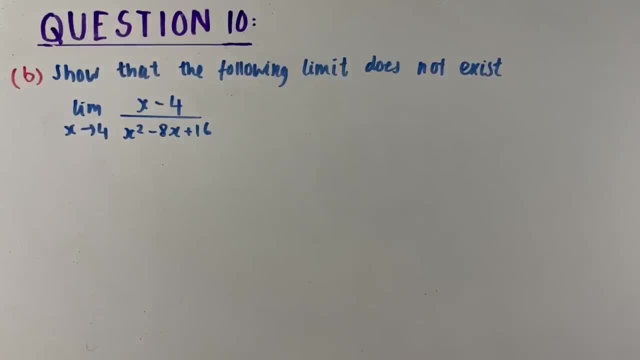 so to show that a limit doesn't exist, let's try and work out the limit, shall we? and if we cannot get one, then therefore it must not exist. So let's again do a bit of manipulation now, kind of like the question before. I'm noticing that on the top we have this x, subtract 4. 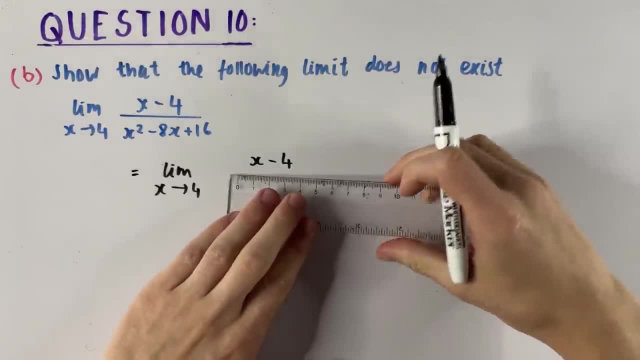 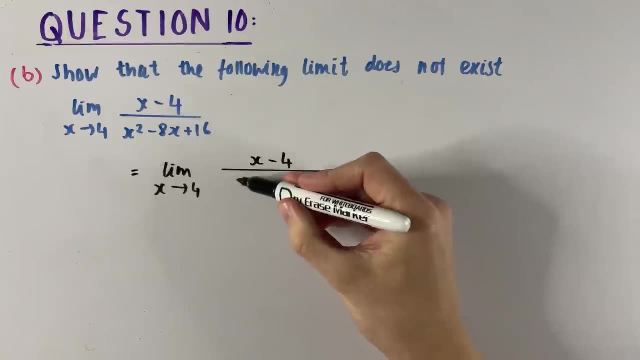 so I have a feeling that on the bottom we're going to have another bracket of some sort that has x. So let's see if we can factorize this bit here. Oh yeah, it's just going to be x minus 4 squared, because that gives x squared minus 8x plus 16.. So we can simplify this by saying: 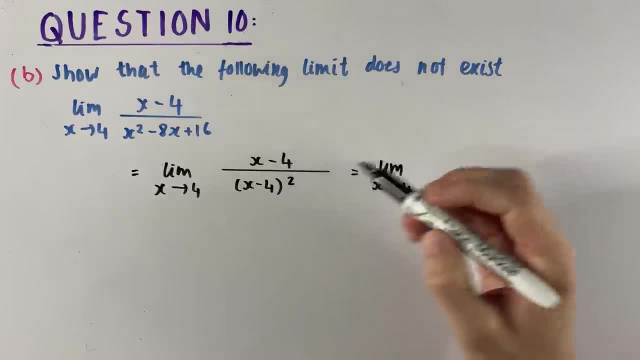 this is the same as the limit, as x tends to 4.. Now we can just get rid of the 2, get rid of that and just put a 1, so it's the same as the limit. The limit has 1 divided by: oh yeah, look at that straight line: x minus 4, substituting. 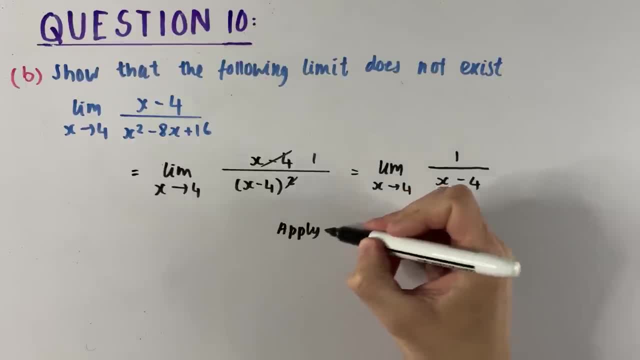 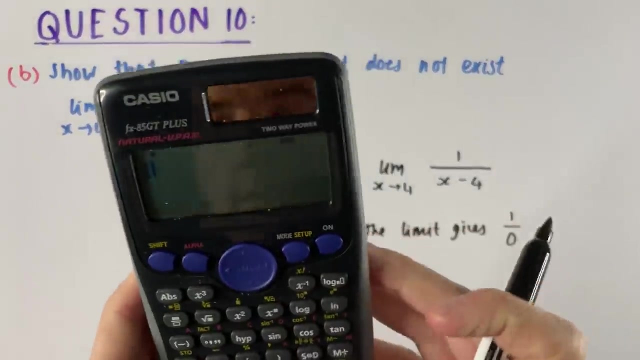 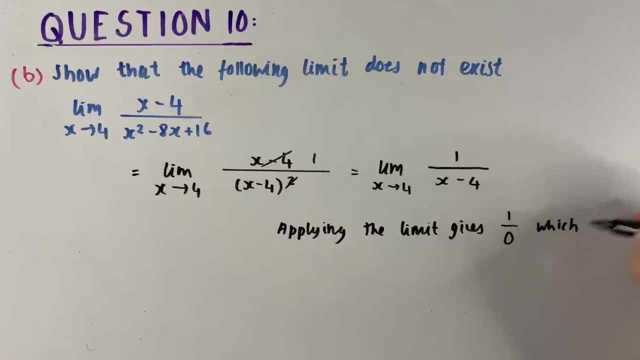 or we can, we can just say: applying the limit gives 1 divided by 0, which again is actually 0. So we can say which is undefined. So we can say which is undefined Undefined. So we can say: hence no limit limit. limit limit exists. 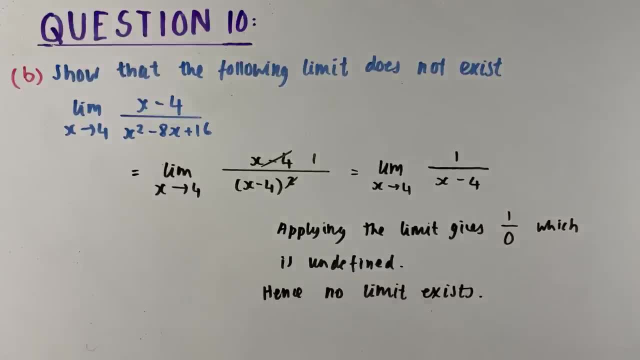 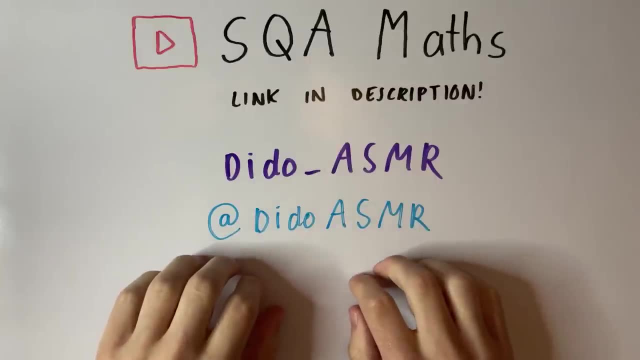 And that is going to be it for the very last question of the night. So thank you for watching. I hope you enjoyed this video And I hope you enjoyed watching tonight's video. So, guys, that is going to be it for tonight's ASMR Maths Video. 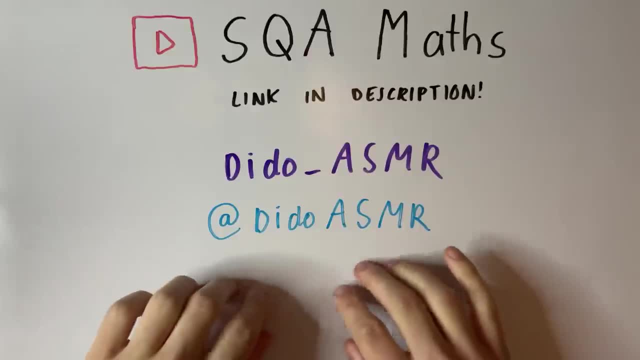 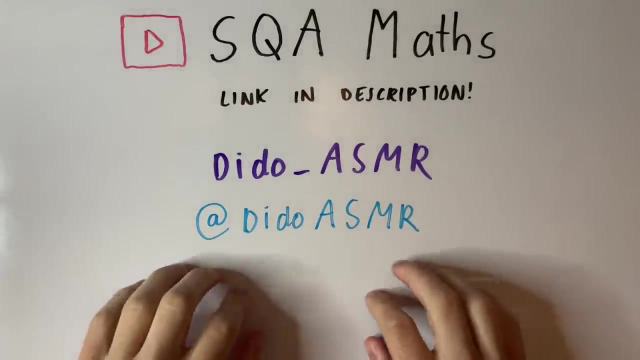 So, guys, that is going to be it for tonight's ASMR Maths Video: Mathematics, mathematics, mathematics, mathematics, mathematics, mathematics. I really hope you all did enjoy it. maybe you learned something new, and I had so so much fun making this video. Again, Before I wrap it up, 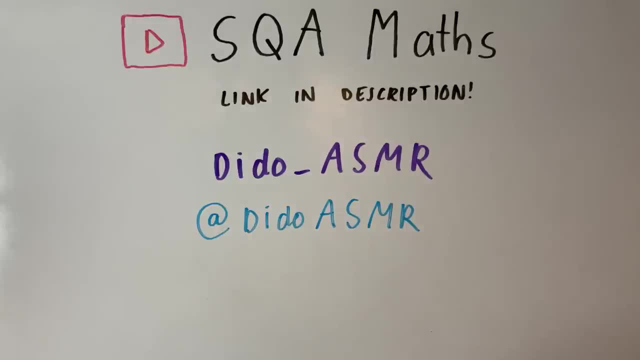 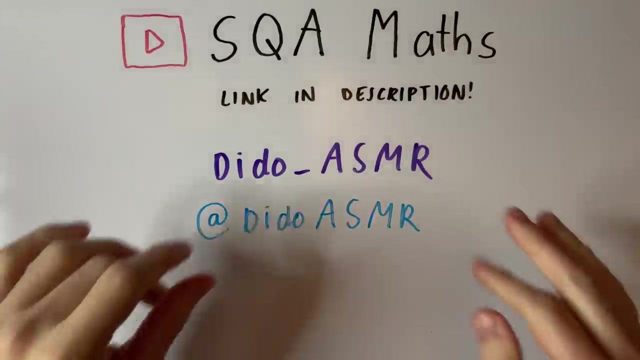 up. I do want to quickly just announce my SQA Maths YouTube channel where I will be teaching mathematics, particularly at the Scottish qualifications level. Please go and check it out. It would be greatly appreciated. I'll pop a link in the description And yeah. 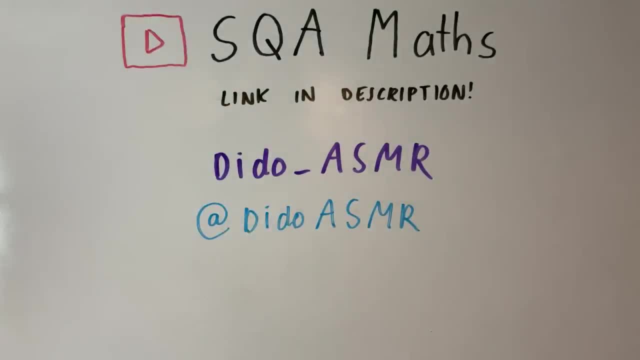 if you guys also have any questions regarding maths or anything in this video, do not hesitate to drop a comment or drop me a message on Instagram or on Twitter, which are also in the description. And yeah, thank you guys so much for watching. If you did enjoy, then,